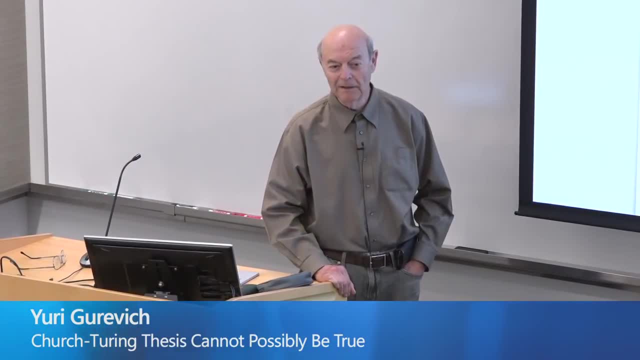 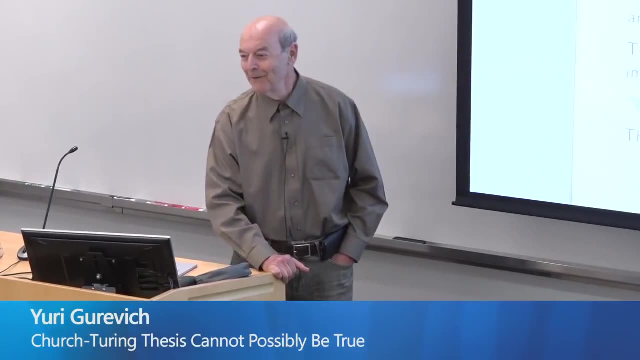 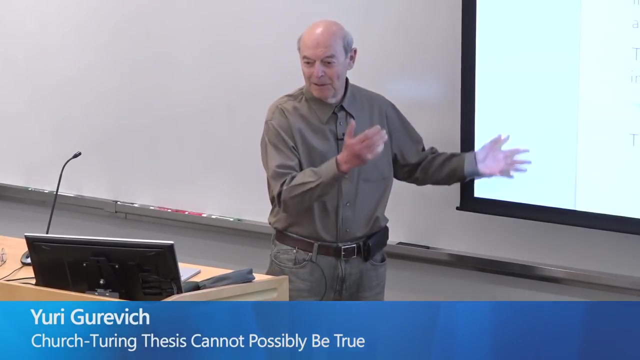 algorithms. Now, what do we mean by classical algorithms? Now, quantum, people hijack the word classical. It became to me non-classical, non-quantum, but our meaning was classical in the sense: algorithms from time immemorial till certainly 1950s till 1960s. 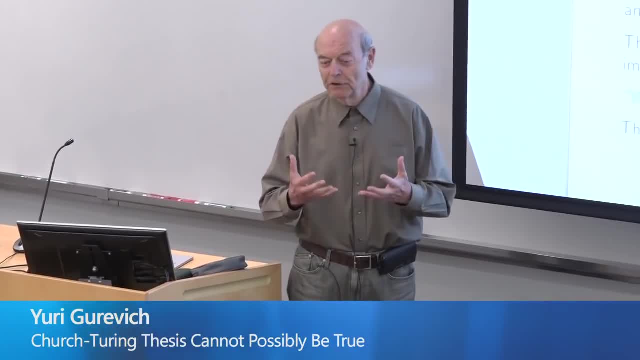 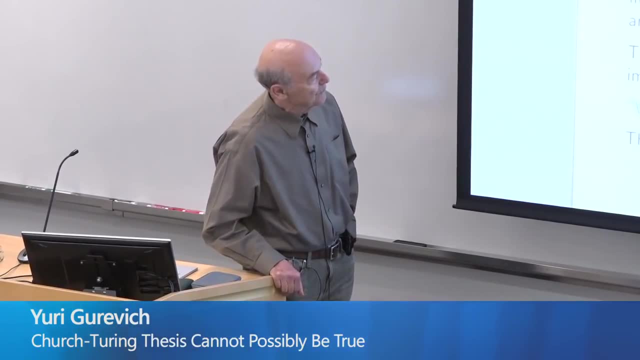 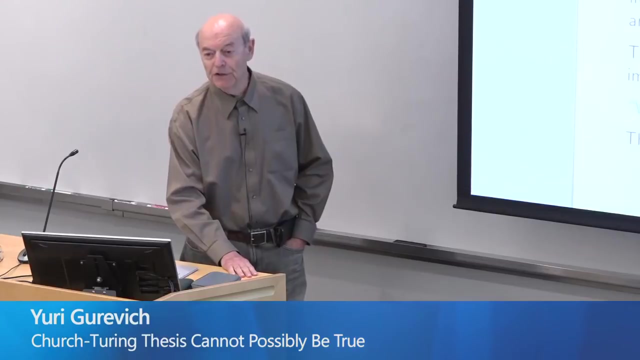 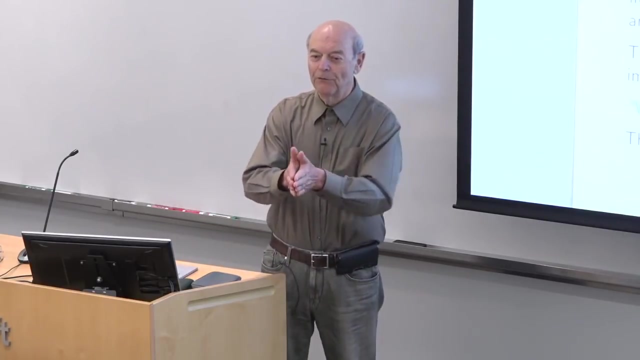 So this is the algorithm that Church and Turing had in mind when they put forward their theses. So another name for this classical algorithms is traditional algorithms or sequential. I will call them mostly sequential because the first sort of non-classical, non-traditional algorithms were parallel. 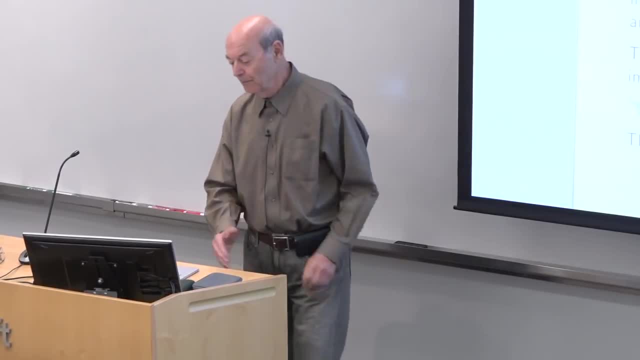 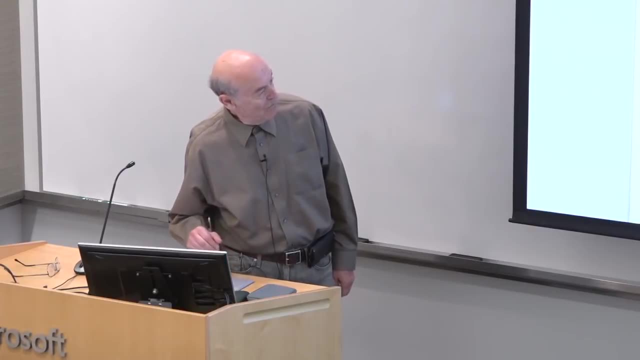 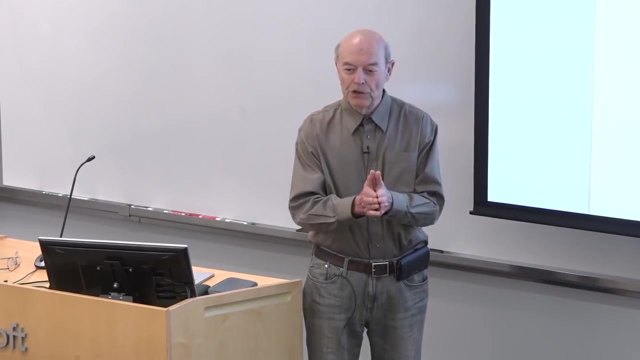 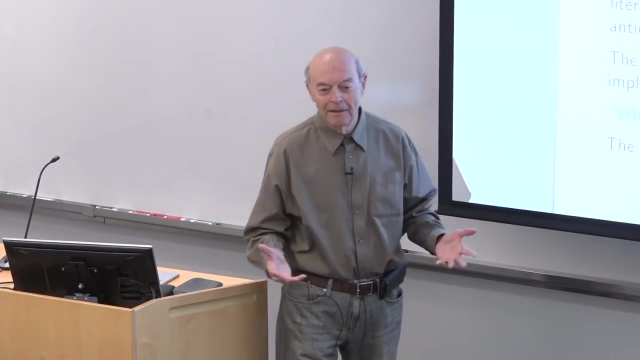 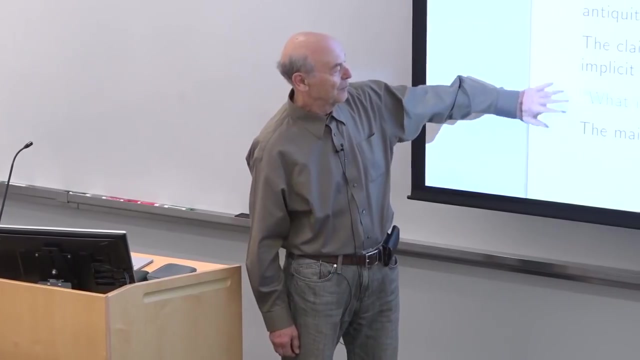 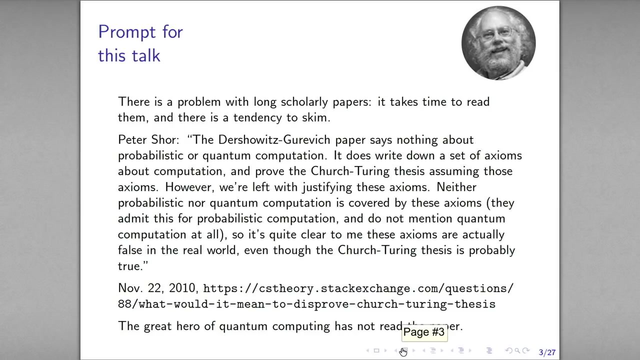 and so those traditional were known as sequential. Now you can generalize, and generalize, and generalize, and then it's not completely obvious why it should be even true, And so I had this argument implicit published two years ago. but, as you see, here is a prompt for today's talk. 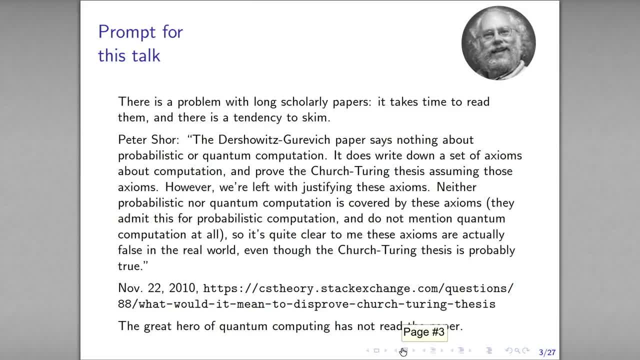 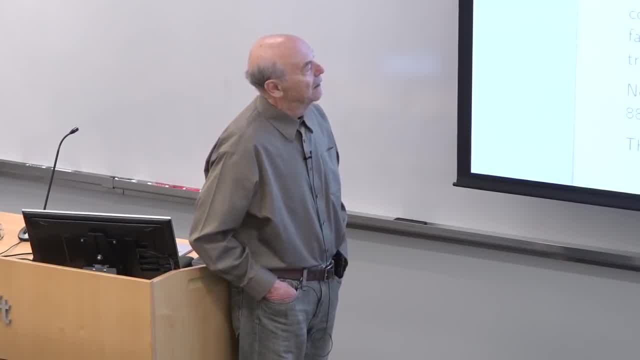 So let me read it. The Dershowitz-Gurevich paper says nothing about probabilistic or quantum computation. It does write down a set of axioms about computation and prove the Church-Turing thesis assuming those axioms. 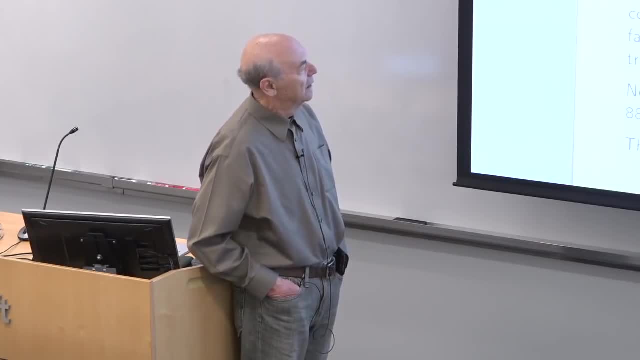 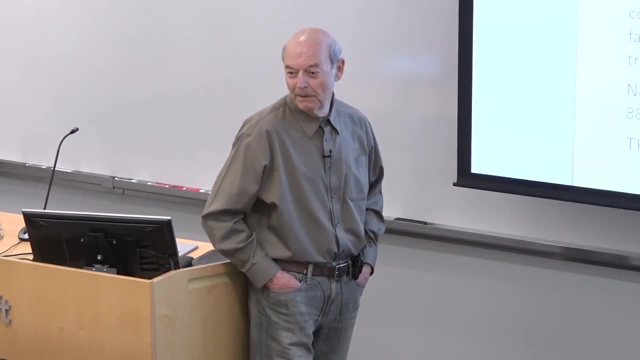 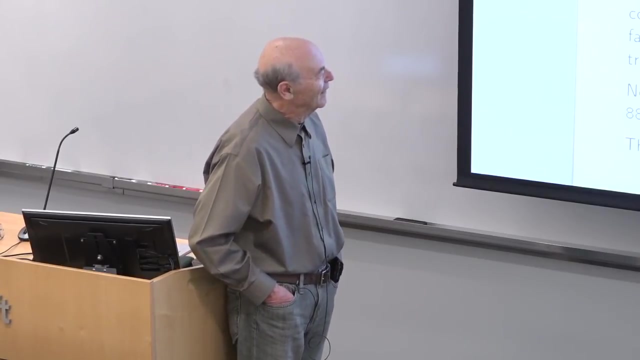 However, we are left with justifying these axioms. Neither probabilistic nor quantum computation is covered by these axioms. they admit this- those criminals For probabilistic computation- and do not mention quantum computation at all. So it's quite clear to me that these axioms are 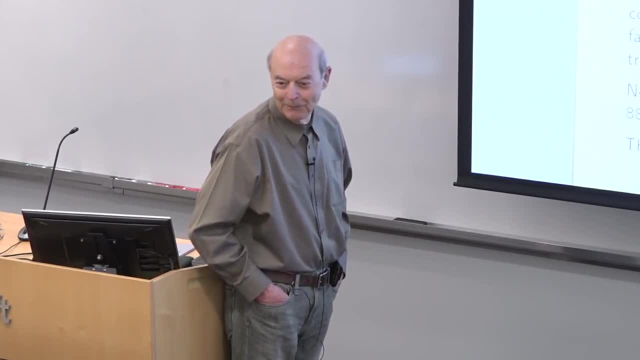 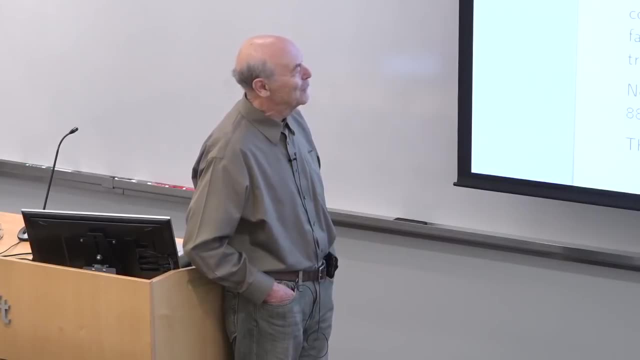 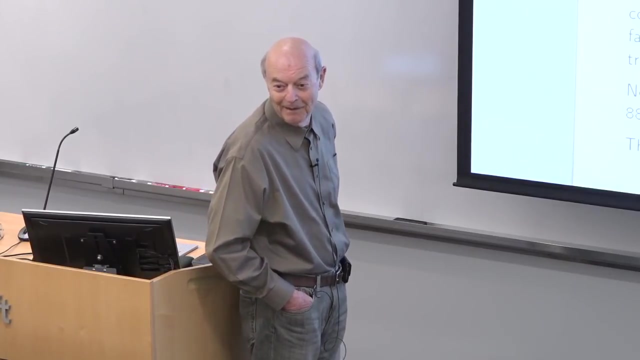 actually false in the real world, whatever it means For mathematical axioms to be false in the real world, even though the Church-Turing thesis is probably true. So there's a problem with scholarly papers: It takes time to read them. 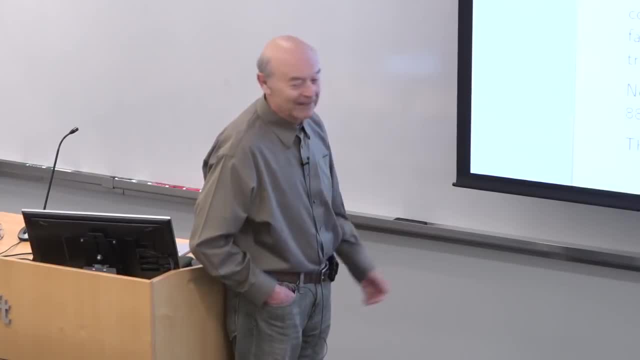 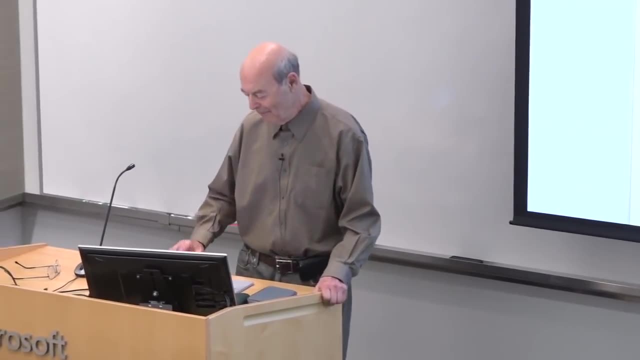 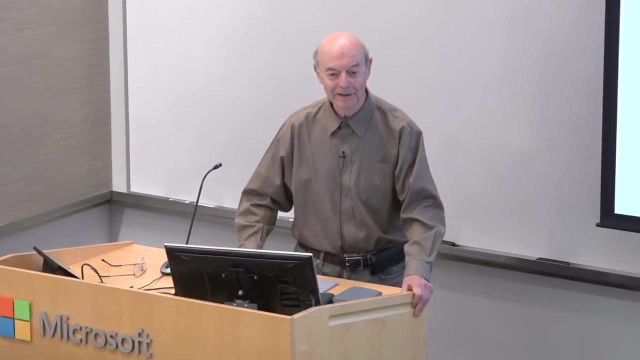 because scheme. So he definitely didn't read. He actually probably didn't read even the abstract, where it says that this is about classical algorithms. Of course it's a great hero of quantum computing, but that's how it is. So let me say what is Church's thesis? 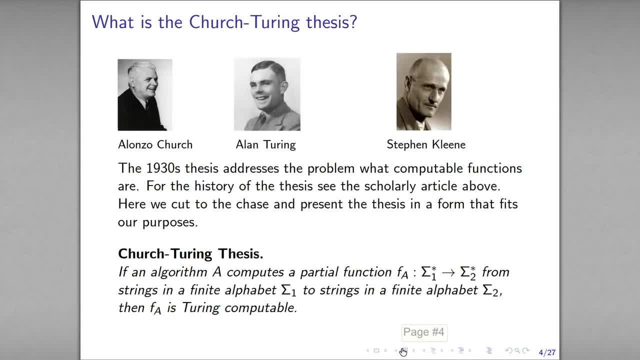 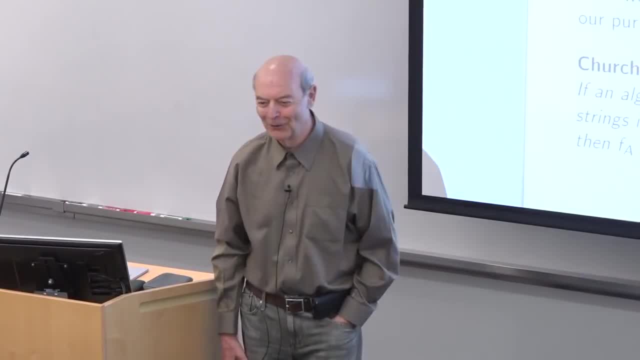 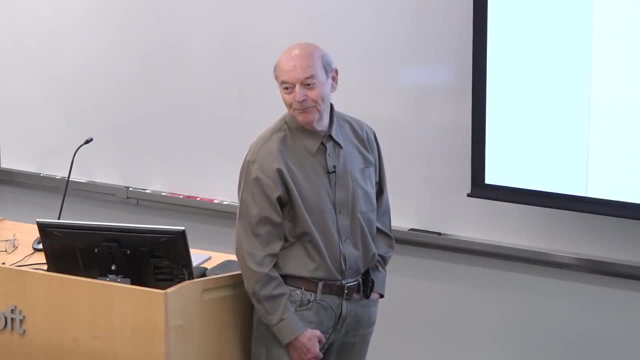 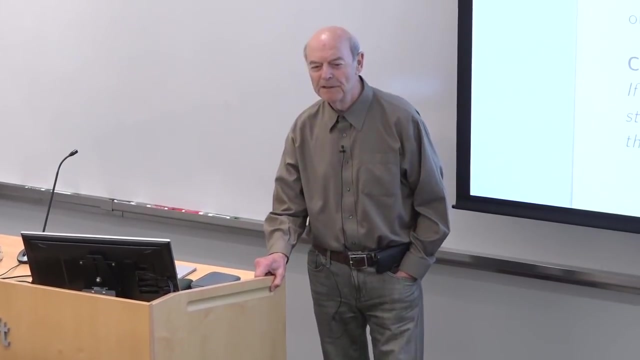 So the tone of the debate hasn't changed from the 1930s. Actually, this discussion was quite civil, It is for sure. There is another picture here of Stephen Kleene, By the way, which means in Dutch: small Klein would be German. 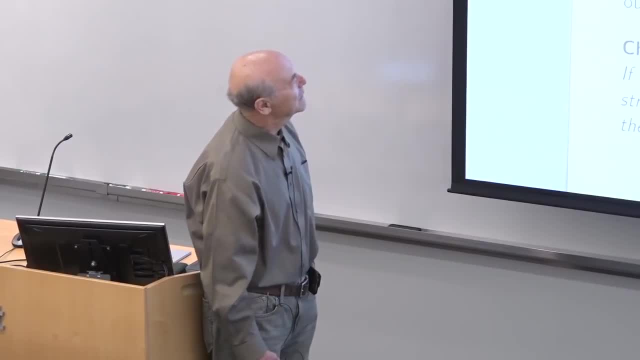 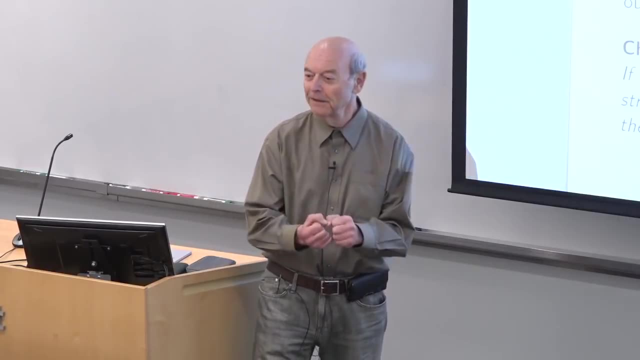 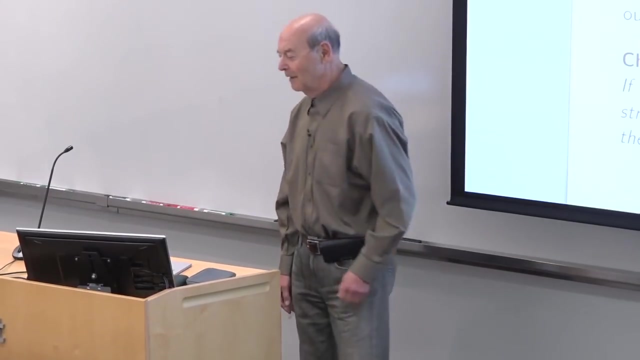 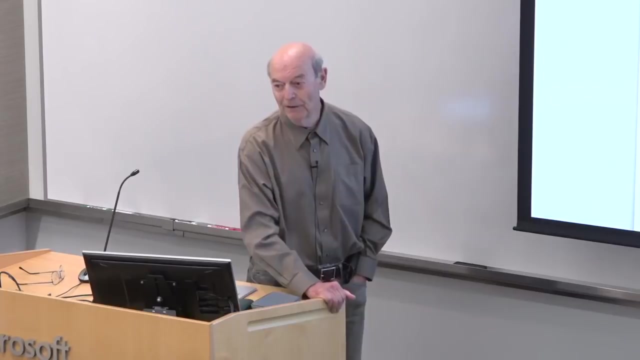 That's the meaning of his name. So he was a student of Church. He actually made the Church thesis what it is. He straightened it, called it thesis. Church himself called it conjecture and spoke only about total algorithms. The better place, the better version is the partial algorithms. 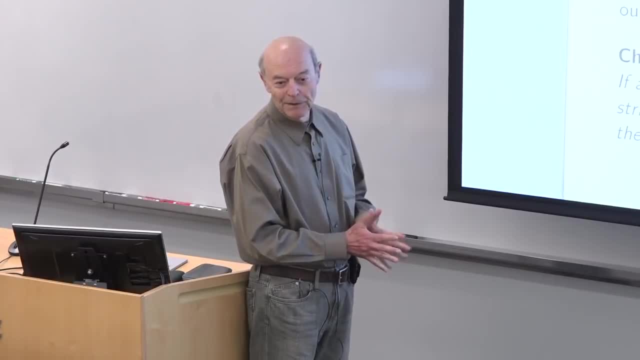 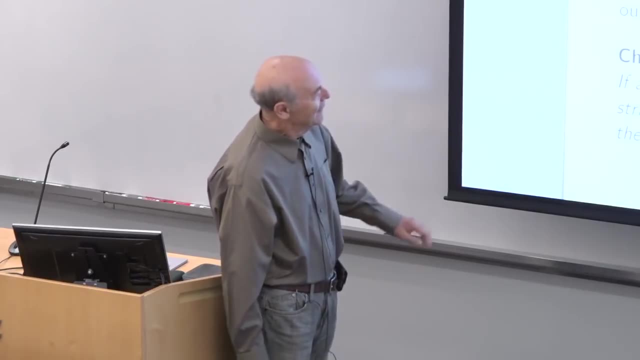 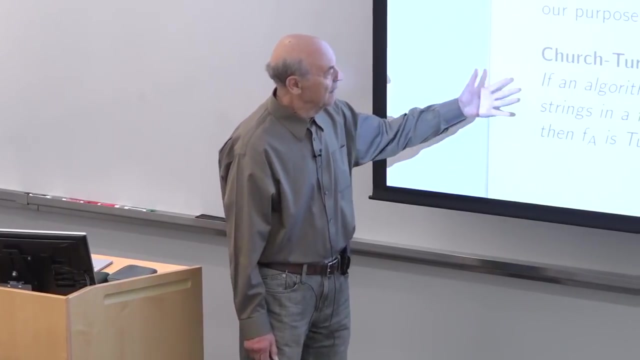 So if somebody interested in history and all the subtleties, I've sent you to our paper with Nahum Jeshowitz, Here I formulate a thesis. there are many forms you can formulate it. They are all essentially equivalent. So if you have an algorithm, 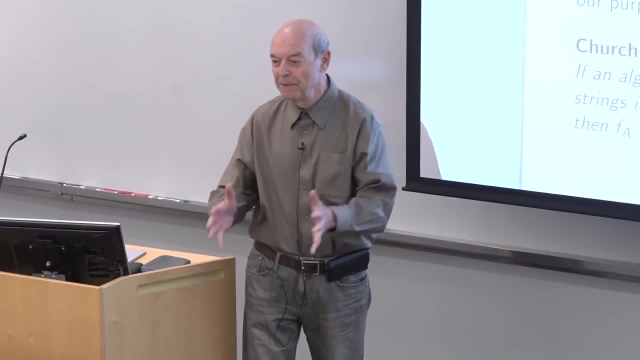 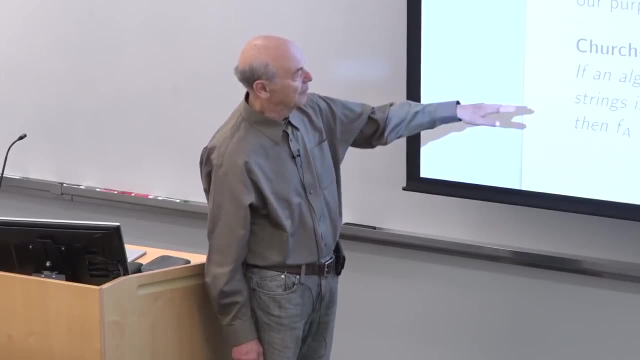 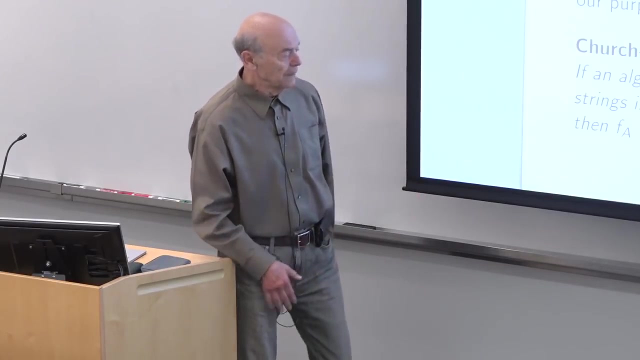 so none of them spoke about algorithm. they spoke about calculability. but there is something that make it calculable, So this is algorithm. So if an algorithm computes a partial function from strings to strings, then it is Turing computable. 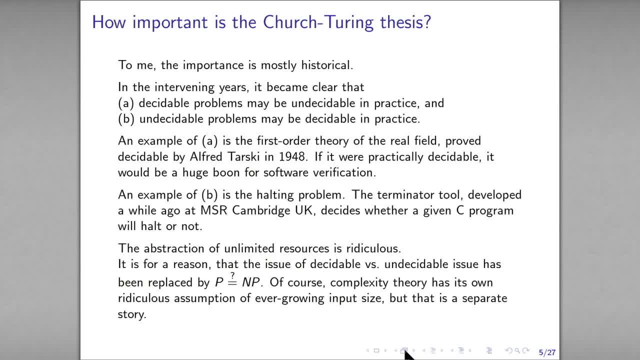 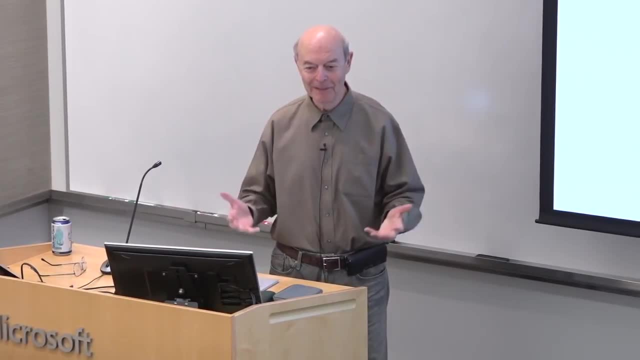 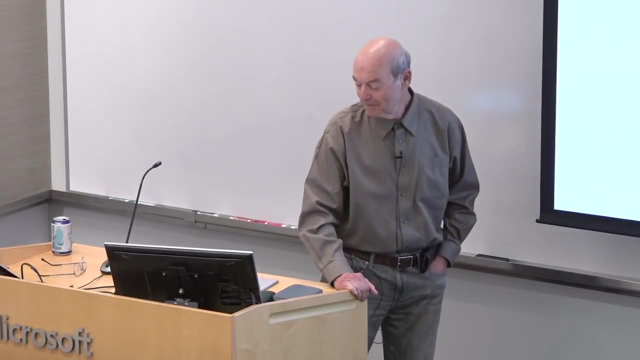 How important is the thesis? I personally think it's not very The importance, mostly historical, but that's how people are. Something historical seems to evoke a lot of interest. So these were much more naive times and decidable seem to be really. 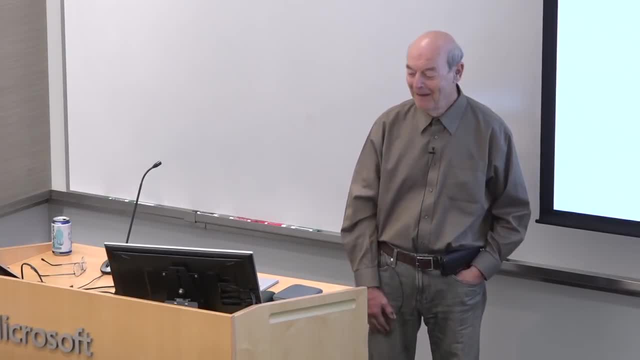 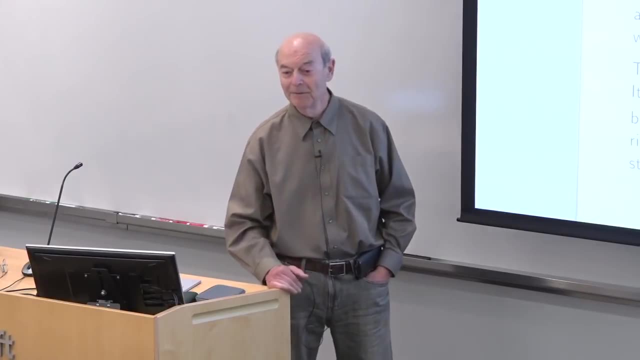 undecidable and undecidable, truly undecidable. But by now we know it doesn't work that way. Okay, So decidable problems may be practically undecidable. So a good example is the first order theory of real field. 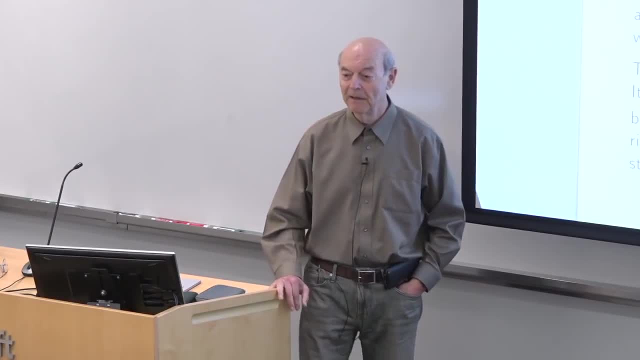 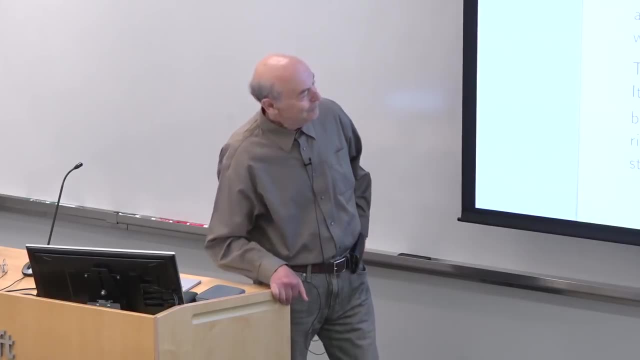 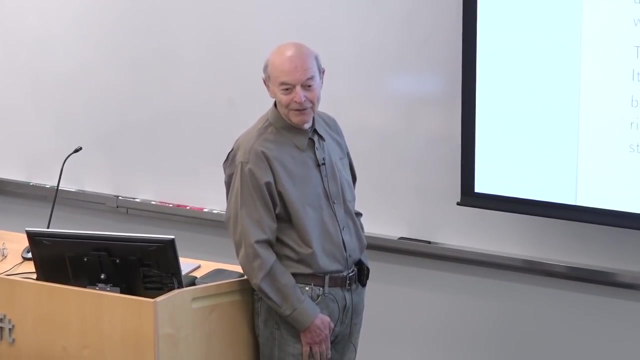 which proved decidable by Tarski in 1948. It's a wonderful result, except you can't use it much. So there are people here who tried. It would be a huge boon to software verification if there was a good procedure. 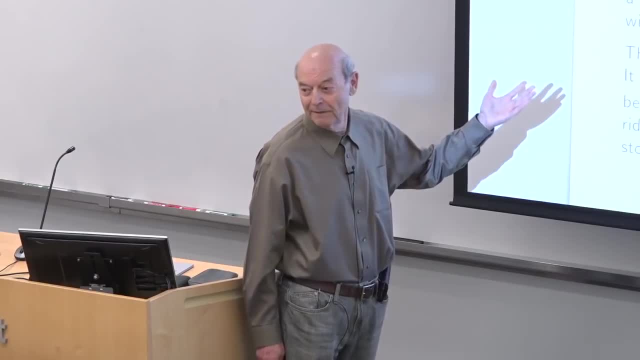 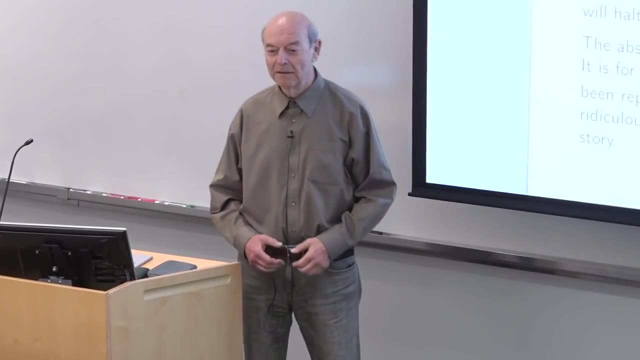 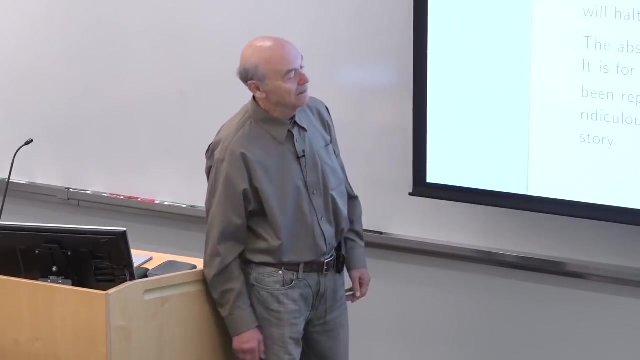 Also undecidable problems may be in reality decidable because these people were the worst case, So they may be decidable if there's a good probability distribution. on average they can be typically decidable. So the classical, the first. 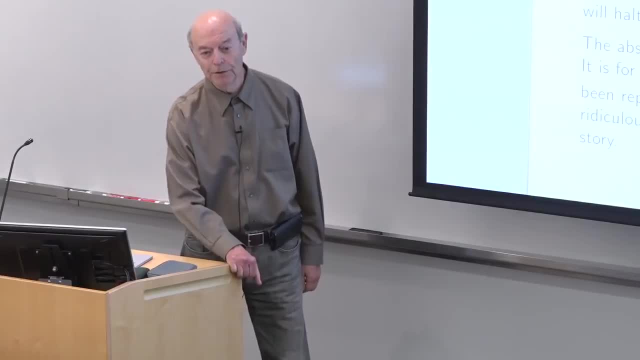 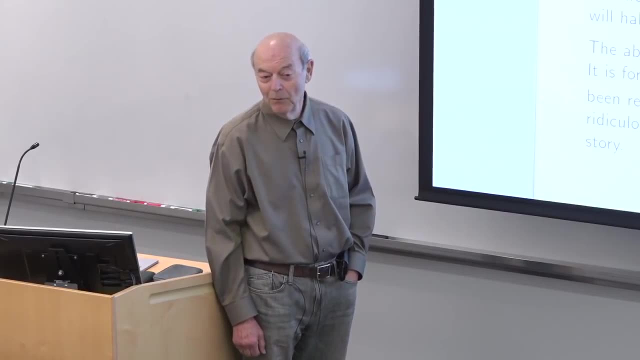 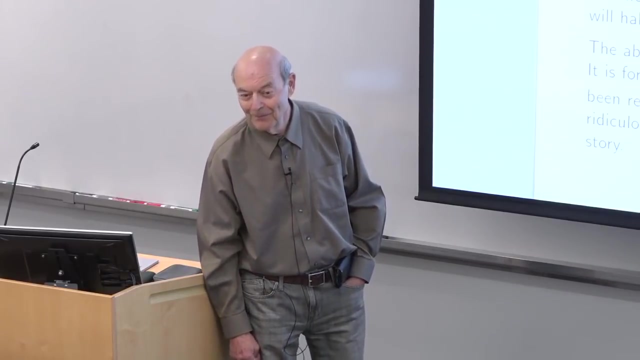 decidable problem was a halting problem. There is a tool called Terminator, which was developed at Masada, Cambridge UK, which worked with C programs. You bring a C program and it tells you whether it will halt or not. It worked pretty good, pretty well. 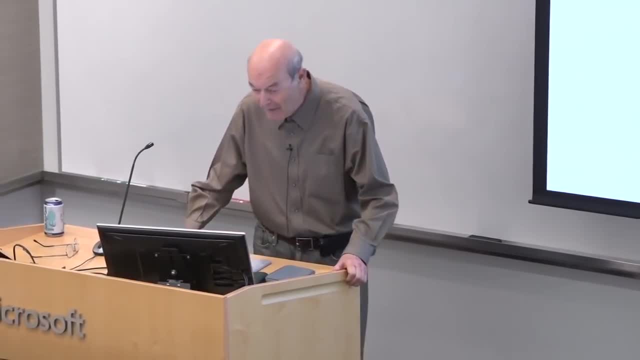 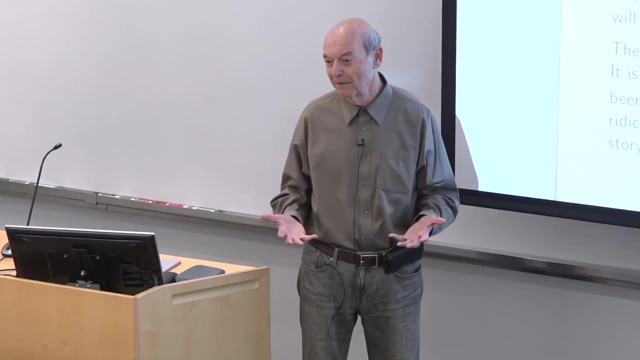 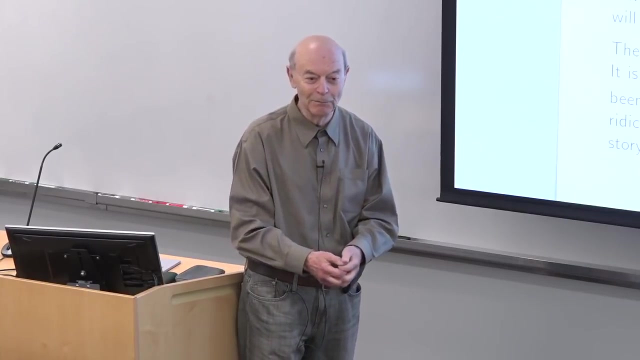 So it probably can be improved. but the whole thing is decidability. It has a ridiculous assumption that we have unlimited resources. Where else in the world do you make such assumptions? Why physicists are interested is beyond me. Physicists are very strange things. 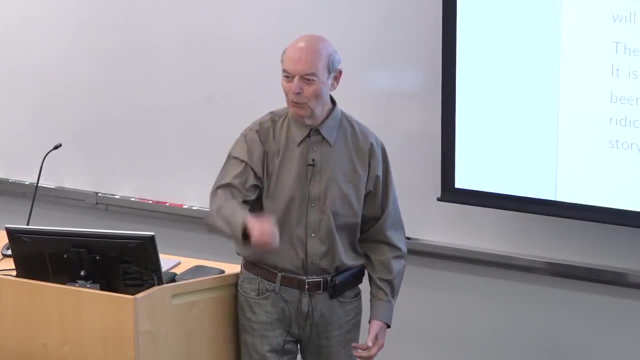 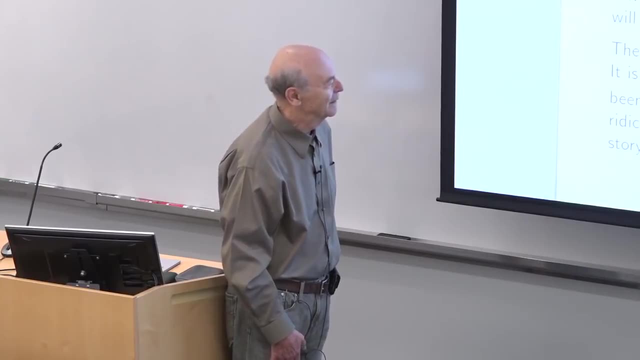 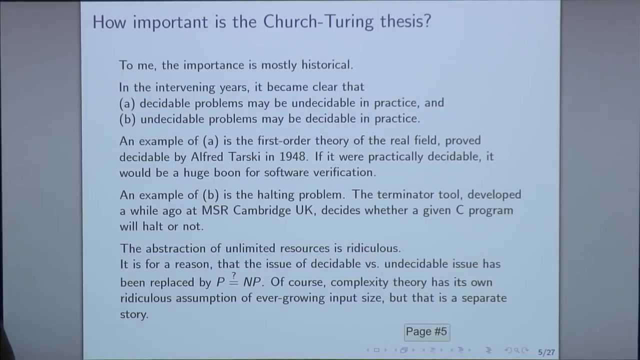 They tend to make huge pronouncement Where there are little reservations here and there, which needs to be made, but are not Anyway. so complexity theory replaced all practical purposes, this decidable, undecidable thing. Complex theory has its own problem. 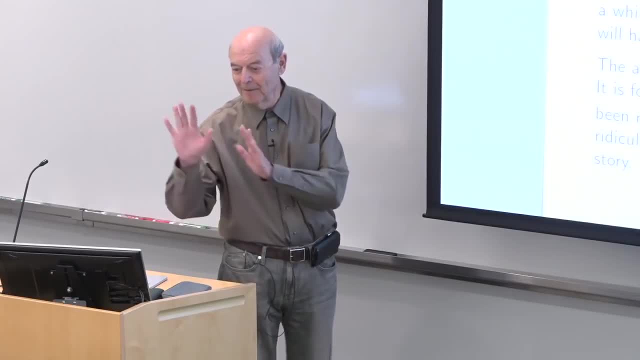 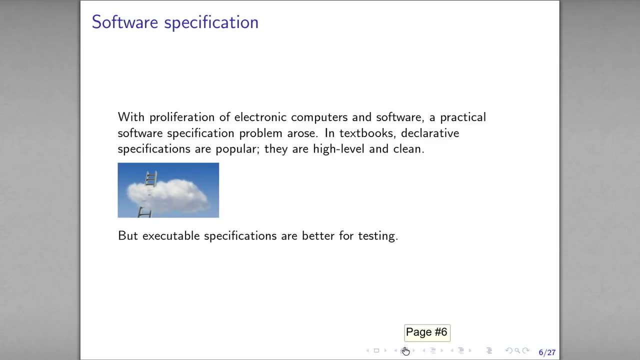 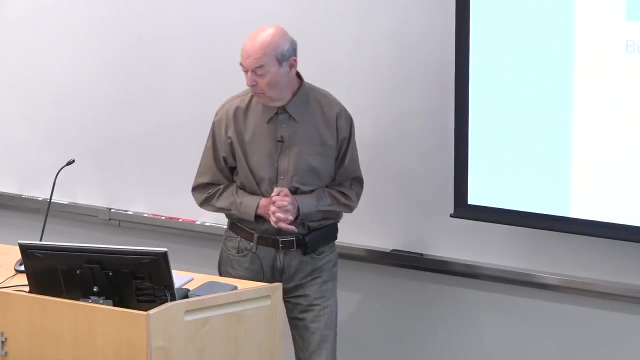 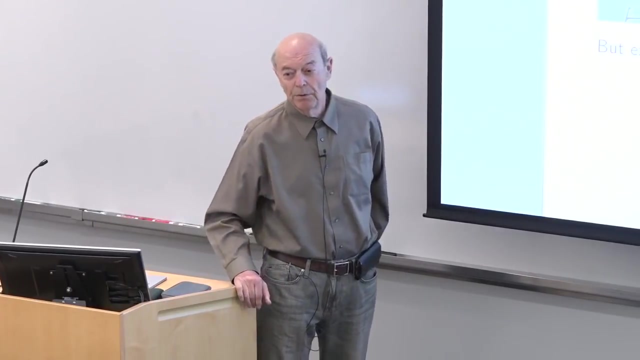 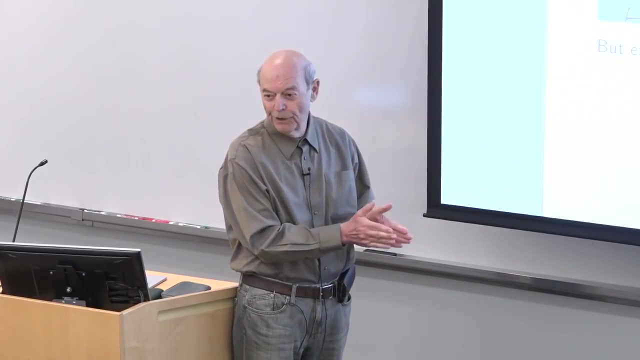 It is asymptotic, but that's a different story. So there are something much more real: software specifications. So I came to this, So I came to computing in 1982, when I sort of moved culture from mathematics to computer science. 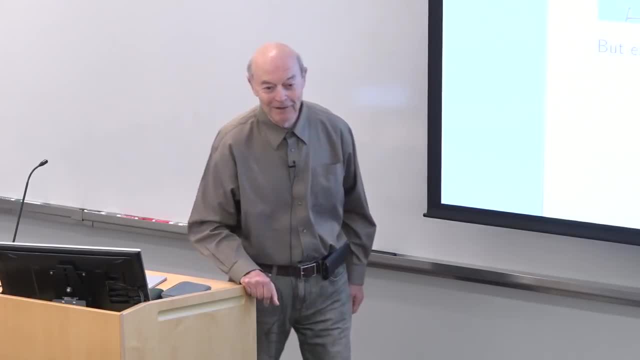 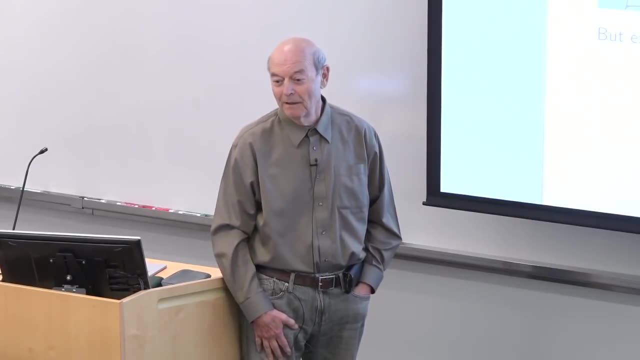 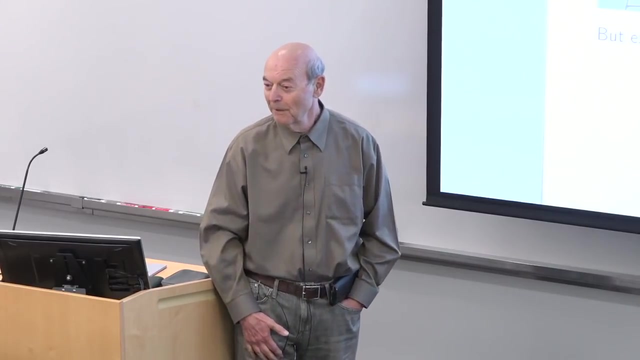 wanted to understand what do they do there? So I volunteered to teach programming and my chairman said no. I said why not? He said we have enough people to teach programming. we don't have anybody to teach theory. Those were the times. 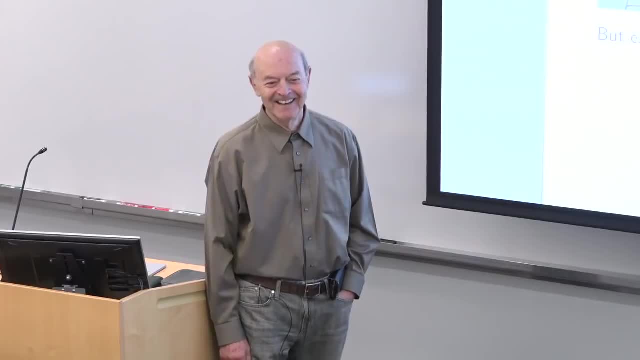 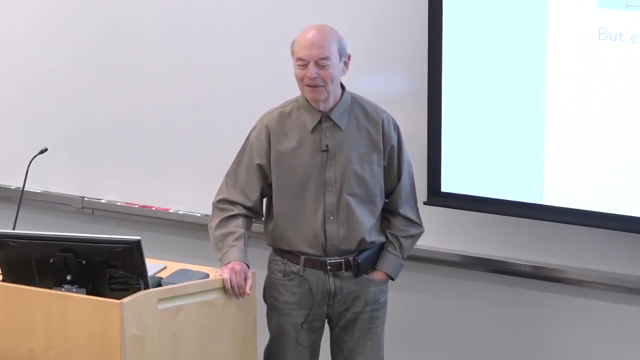 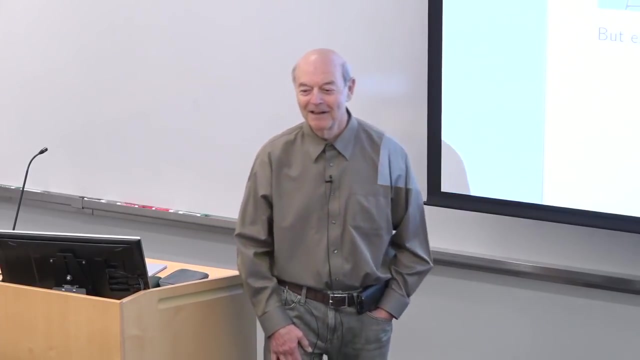 not enough theorists in computer science. I said: but if I always stick to theory, I will never learn much about computing. He thought a little and says: okay, once You teach it once. So I taught essentially Pascal and then I discovered that I have 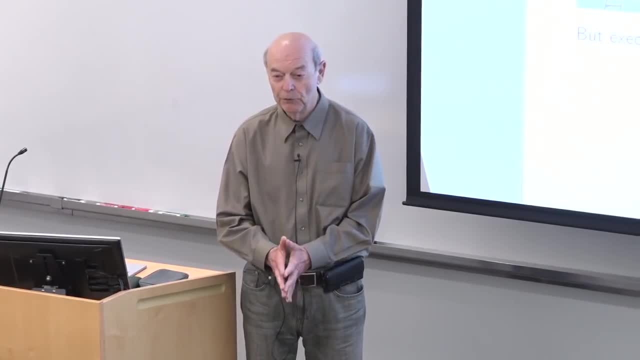 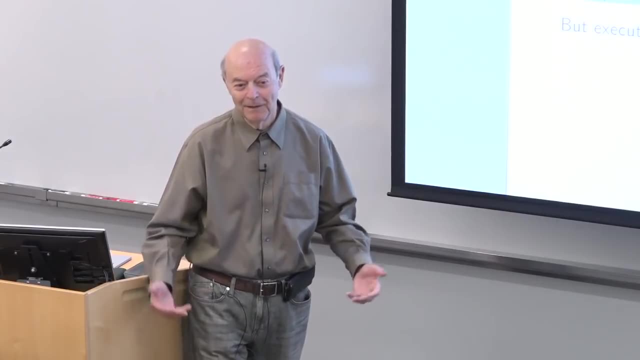 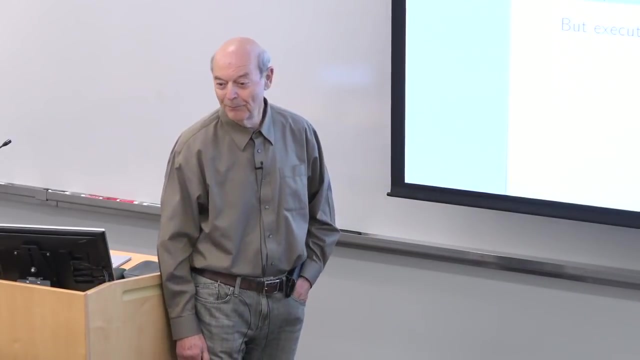 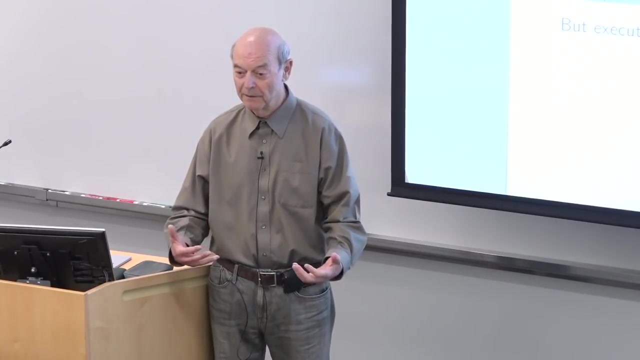 my little Macintosh and University of Michigan had a huge mainframe. They actually competed with IBM. There was seven, eight universities around the globe that adapted this Michigan Terminal System. So in any way, as far as I'm concerned, there was just two compilers. 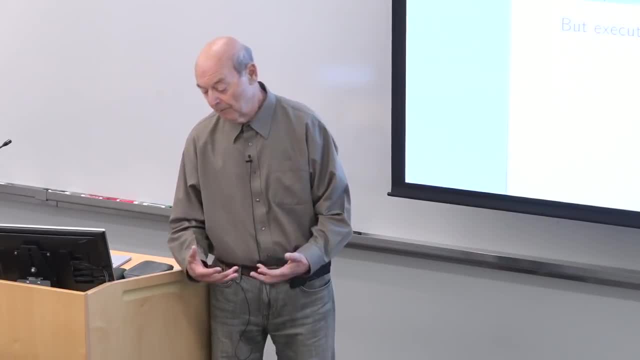 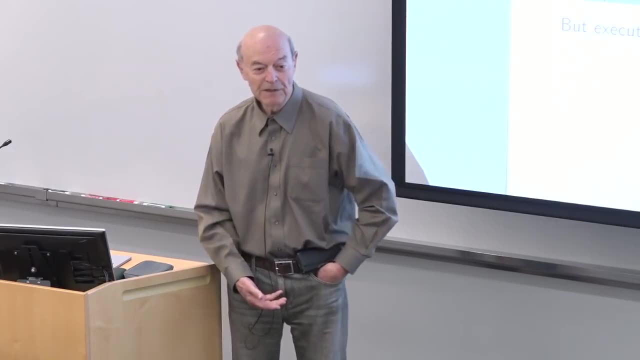 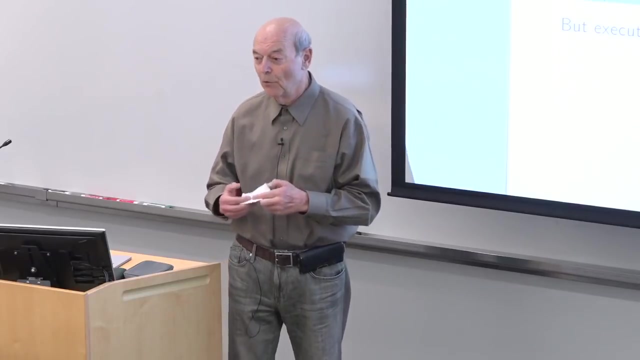 one interpreter, one compiler for Pascal and they disagreed: What, What's Pascal? I'm a mathematician. you teach something, but what it is you don't know. There is no. nobody knows what Pascal is. There is no canon, there is no definition. 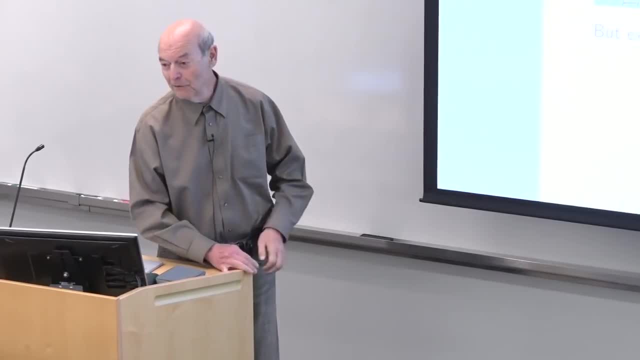 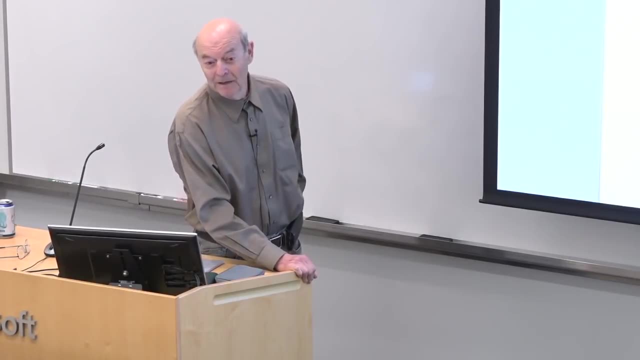 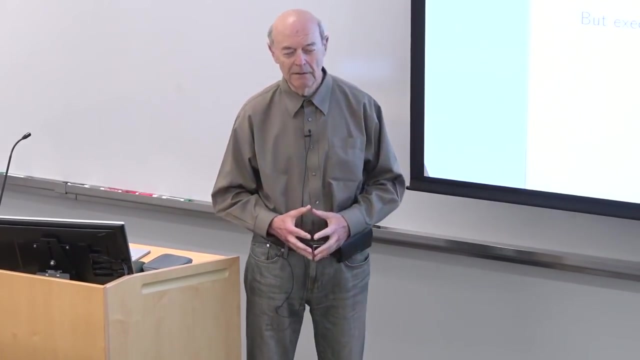 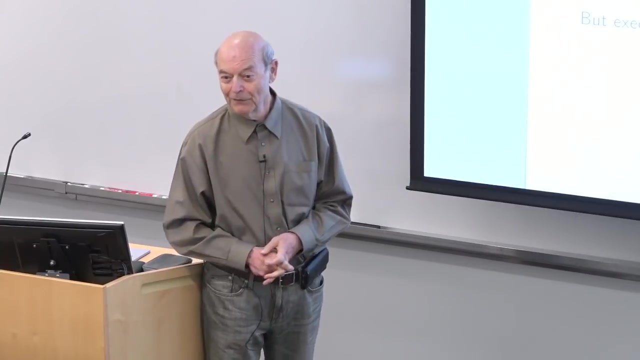 So that arose my interest to all these things, especially to specifications. and then I discovered that everybody among the theorists likes this declarative approach. So I knew these people, like Dana Scott and others. I knew they are not good programmers. 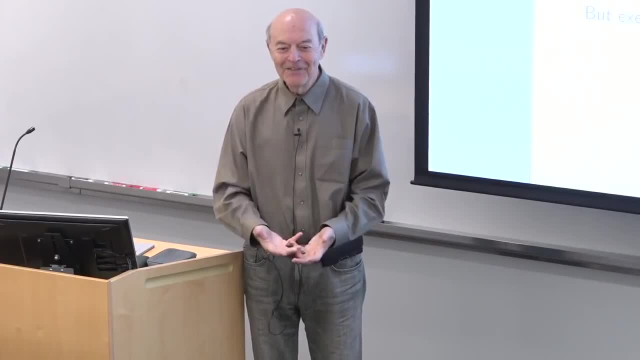 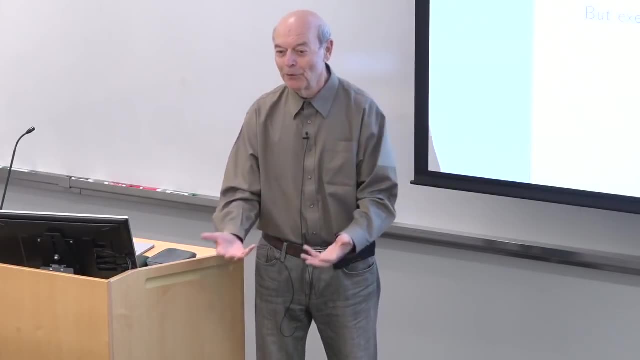 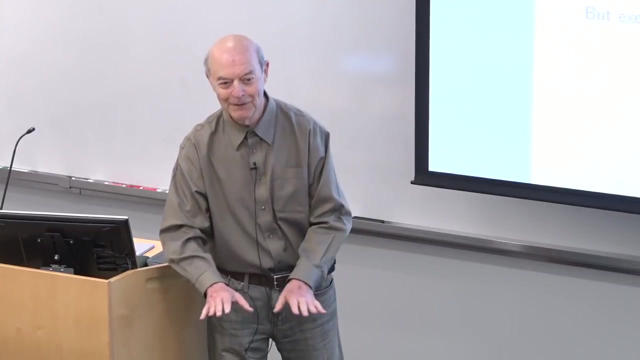 So how can they teach? There is this population of programmers, engineers, who actually brought all those positions that feed us, and now you tell them: no, no, no, you're all doing wrong. Everything should be declarative, clean, high-level. 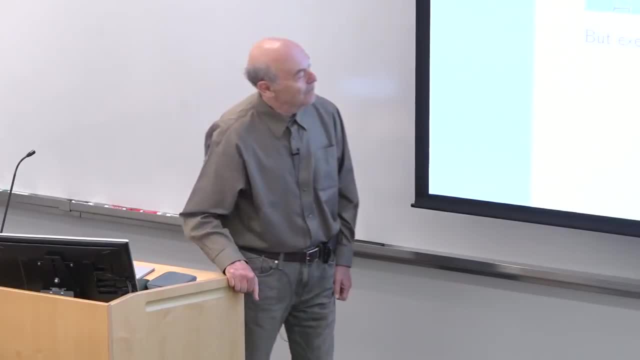 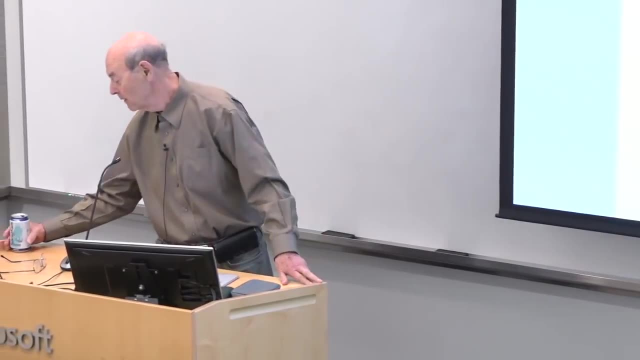 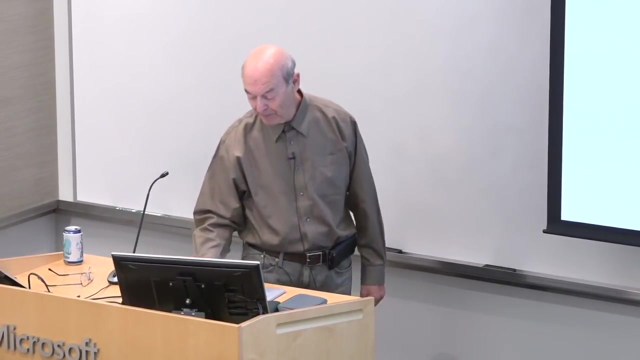 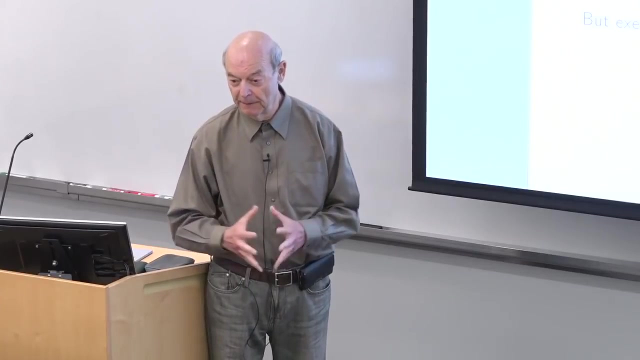 so my impression is that executable specifications are the way to go. which- and I was actually laughed at by theorists- Can you define executable? You can execute. So there are companies like Zed, So you can invite there. you say: here is my software. 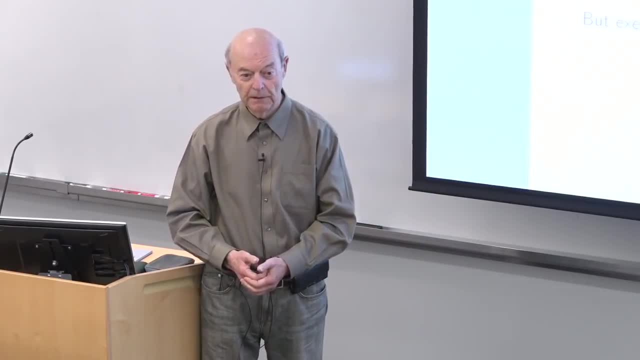 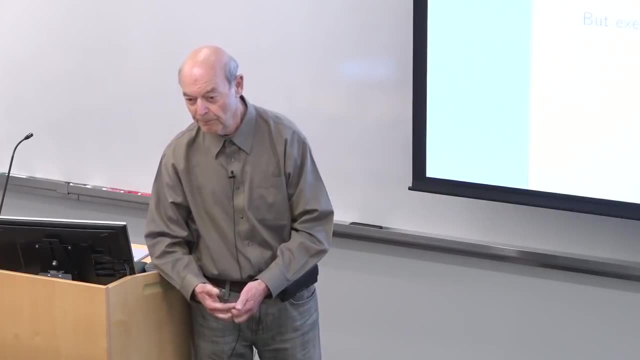 software I'm doing. the experts come and take a few months and they write a book. and they bring you a book. Now, nobody in your company can read this book In the meantime. software it's like organism: it doesn't stay in place. 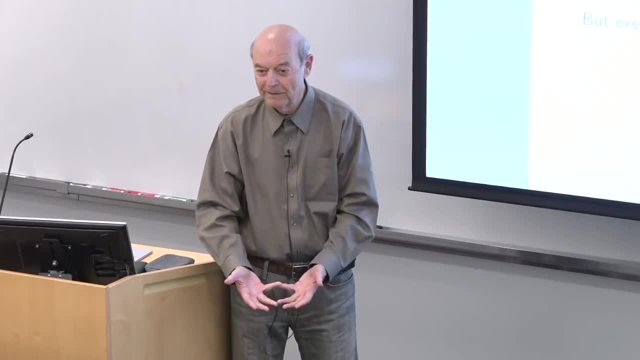 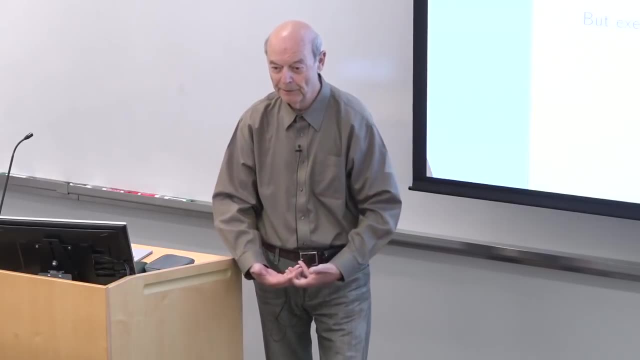 It's developed. whether this book was ever reflecting the right thing, we don't know. It's useful Often. it's useful to read it because you see their way to how they understood and they're often very clever, good people. but you cannot. 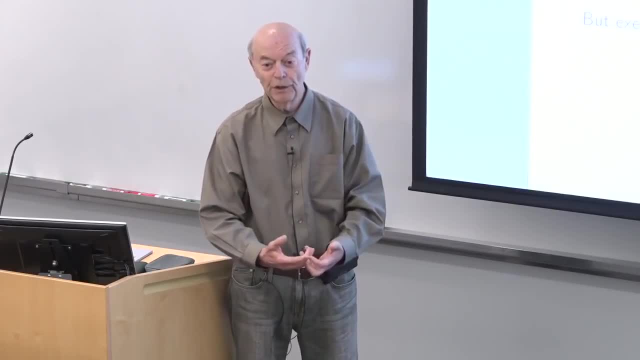 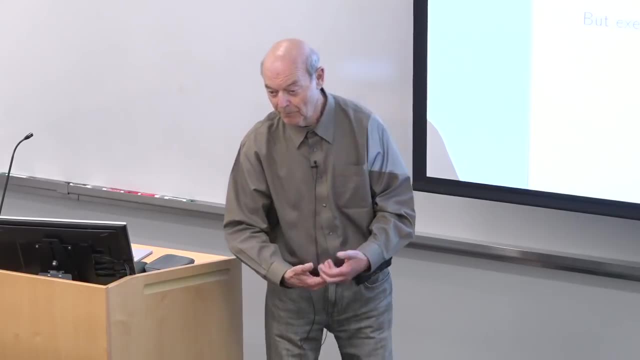 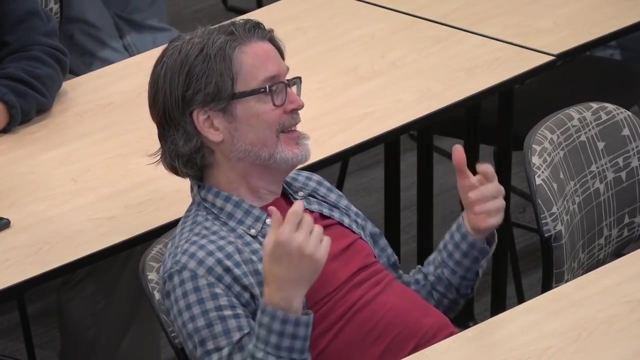 test against the book. So what you want to have, you want to have a specification which you can run and compare. Yeah, I'm just asking what is the meaning of run? Is program executable? At what level of complexity do you call it executable? 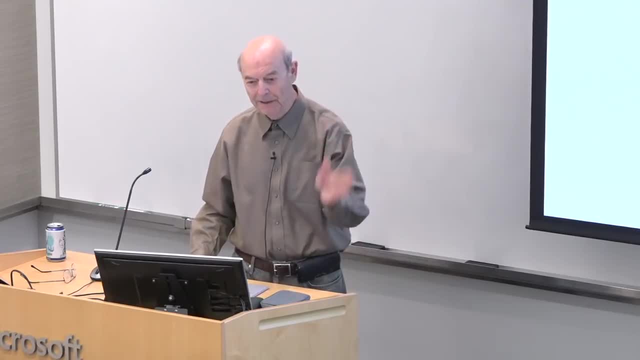 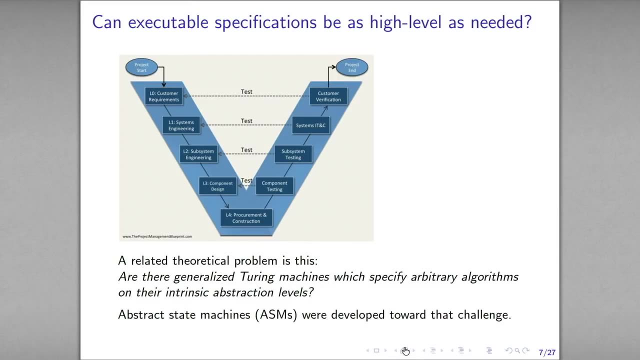 Well, that has state, state evolves. at the end you have fun. Just normal run, anything which runs. So a written prescriptive: Operational, Operational- yes, Operational is executable for me, synonyms Okay. So this is a famous V-diagram of software engineering. 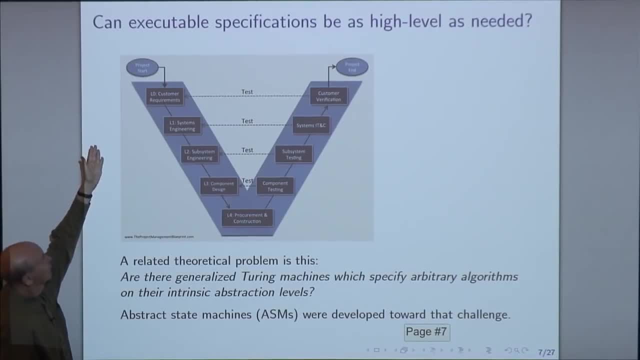 So you start from certain problem, you refine, refine, refine it go down in levels of abstraction, then you code and then you test- Component test, subsystem test, and so on go up. Okay, Now then 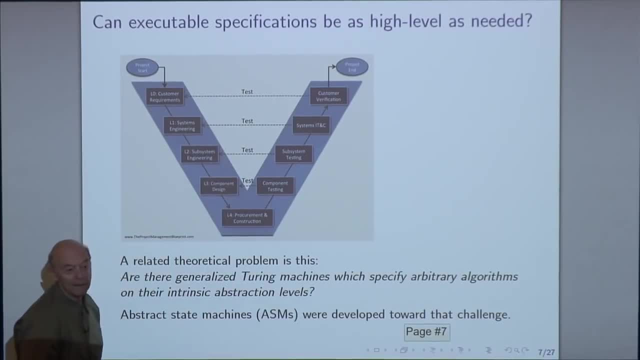 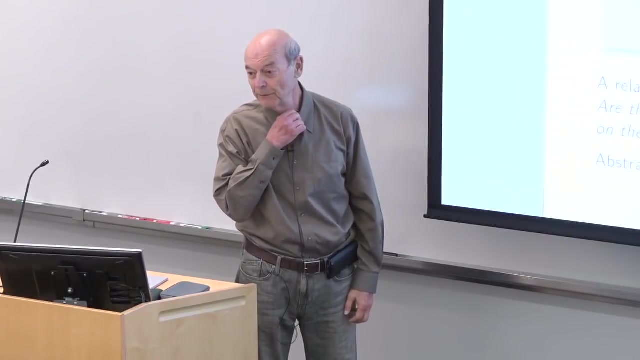 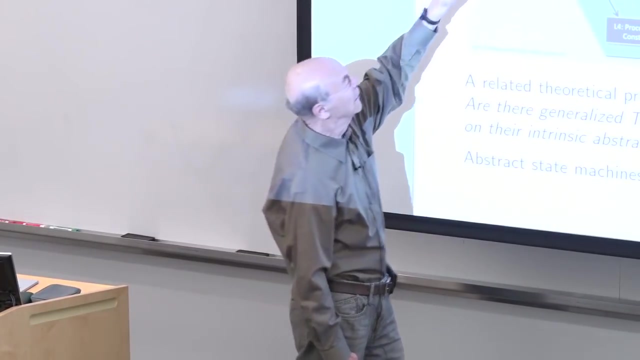 suppose you discover, say this test, it's wrong. In the meantime a lot of people did a lot of work until you discover this. So the obvious idea, which was around a lot, was to test in this horizontal ways on the same level of abstraction. 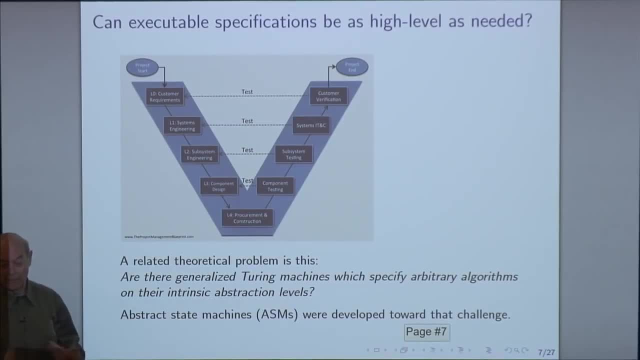 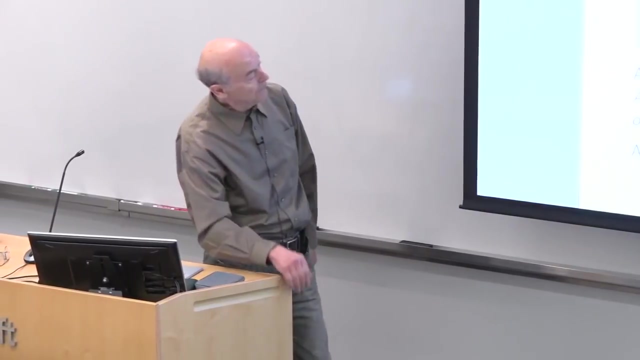 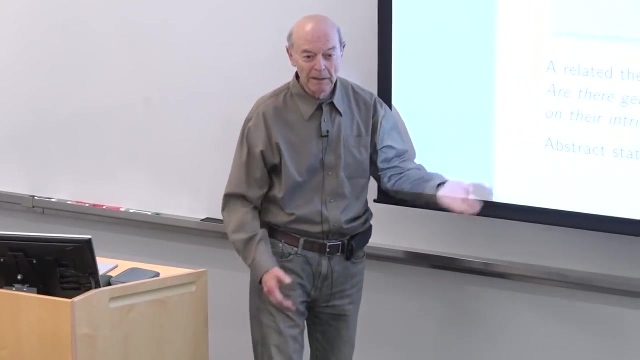 So, in order to test, from my point of view, all these should be, algorithms should be operational, executable programs, high-level, maybe not very efficient, But nevertheless. so I started to think how to approach it. in general, There is this theoretical problem. 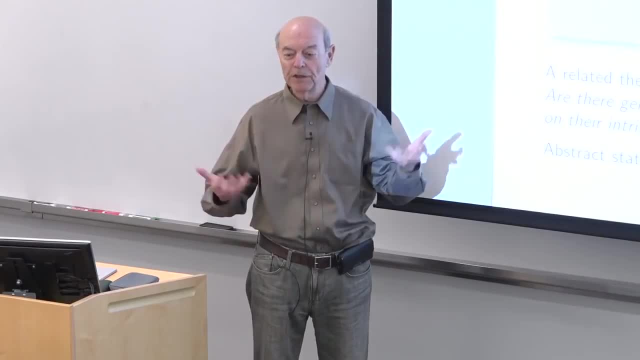 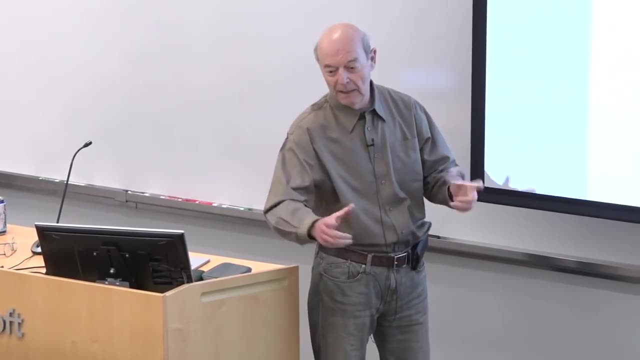 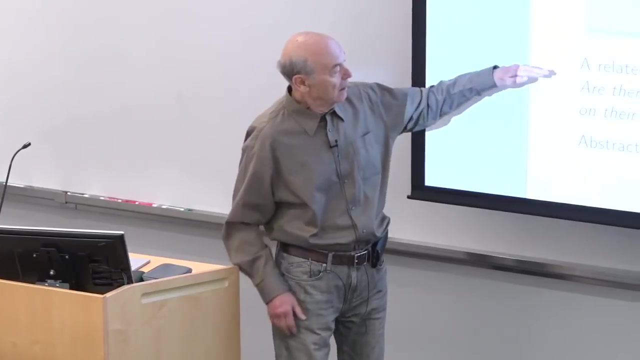 Can you have a more general kind of Turing machine? Of course Turing machine is ridiculously low level. It works with single bits, Yes, And one tape and so on. But can you have a very advanced, versatile computation model which is executable, operational? 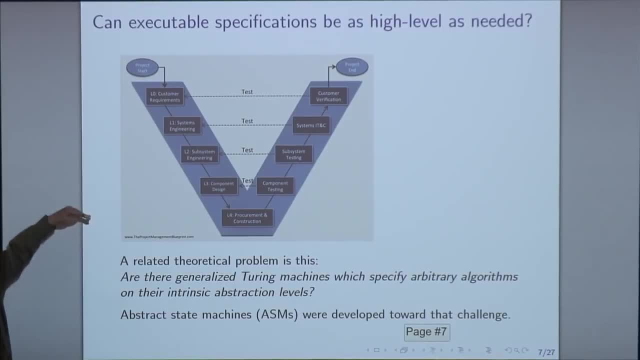 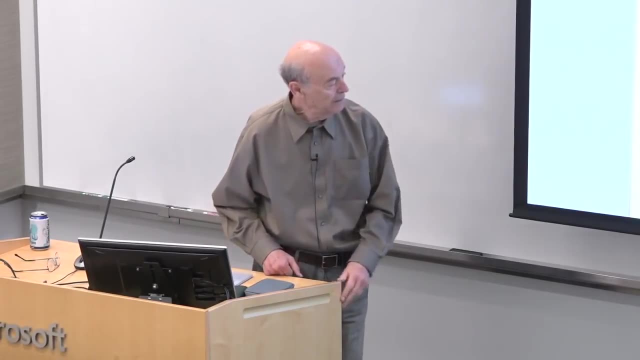 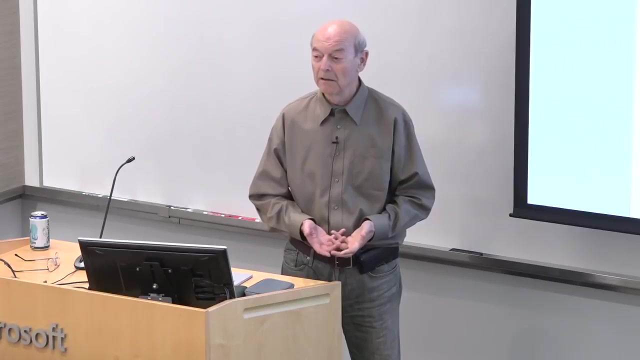 It's an algorithm. you can run it on any level of abstraction, So you can simulate on any level of abstraction, and abstract state machines were developed to meet this challenge. So my first thought was: now it can possibly work. 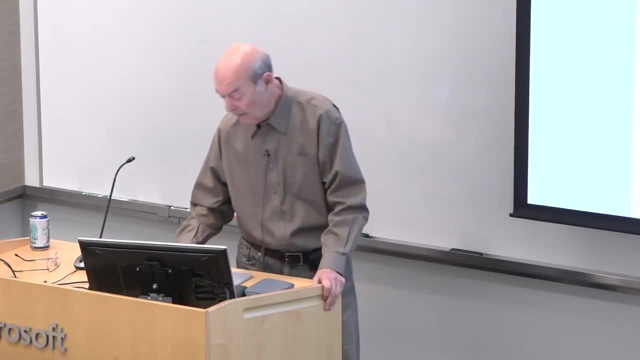 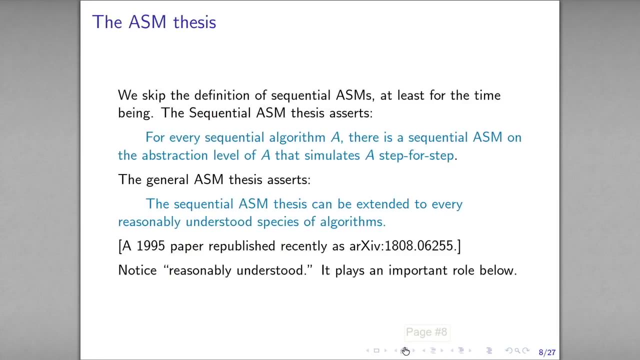 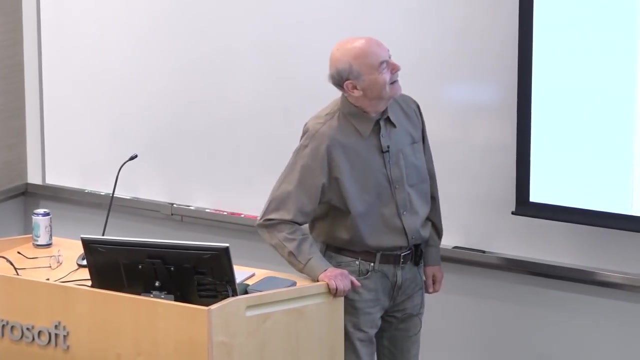 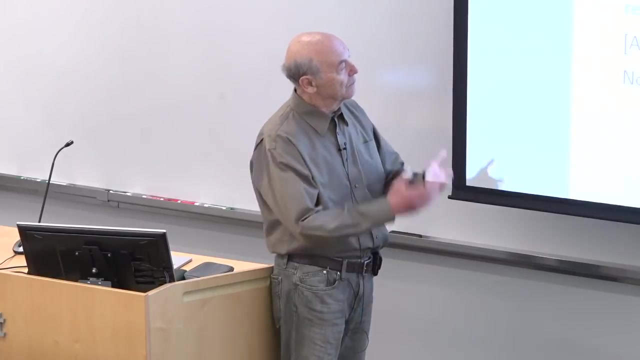 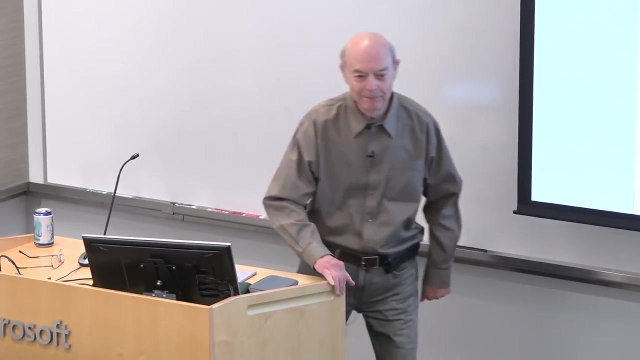 So I said: but nevertheless, let's try. So first I worked with sequential algorithms. In fact they're only algorithms I knew at the time. So I had these machines. I can't explain them again. but then I give me go with my story. 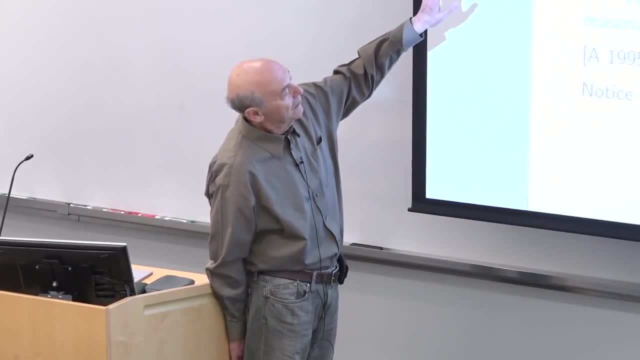 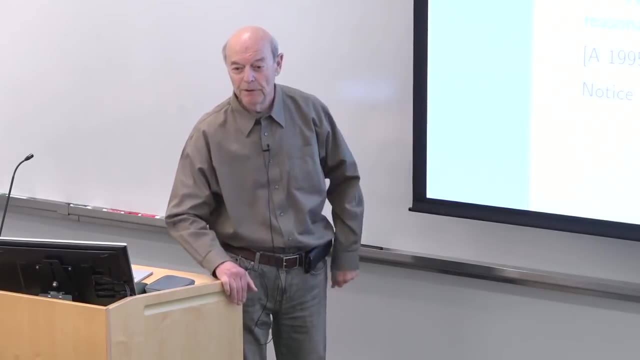 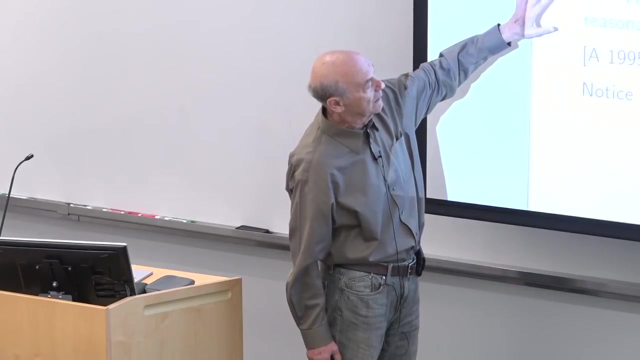 with somebody who wants to be happy to explain what they are. So there are some people who like the ideas. the ASM community has been formed here in Europe and other places. Then we pushed it to paralleled dual armies- Yes. 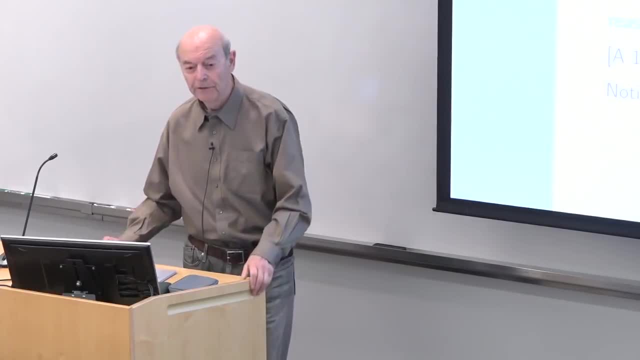 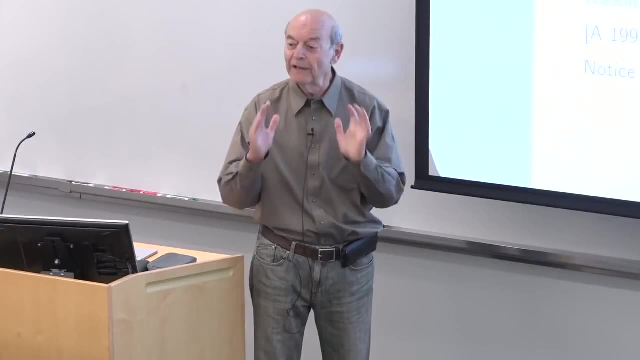 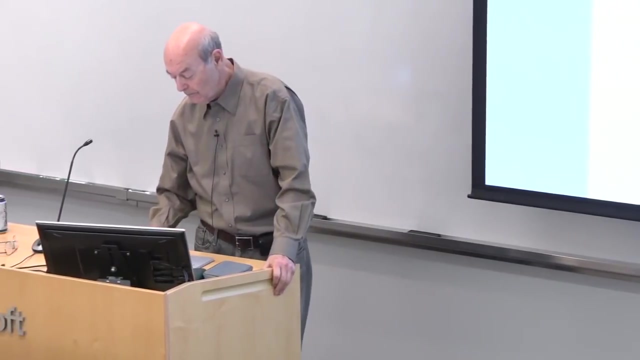 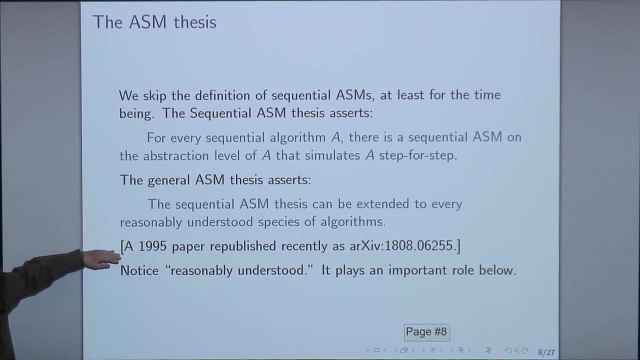 I understood that parallelism, parallelism algorithms to interactive algorithms, to all kind of number of classes, each time when things are well understood, not just to algorithms. So this is the general thesis from this paper. It's in some Oxford U press which is not available. 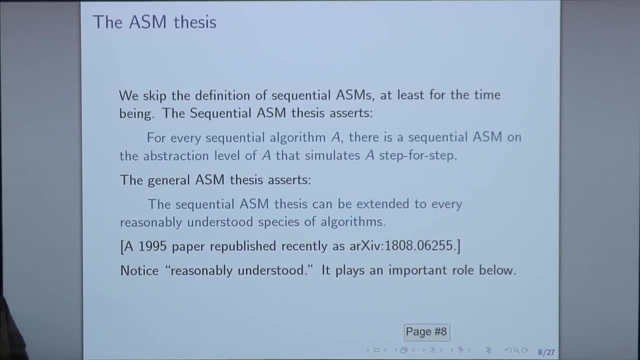 so I just when I thought about this talk, I went and made it or thought maybe I want to give this talk, So I made it in archive version. So this is a more general thesis that whenever you have a reasonably understood- okay, this is a thesis. 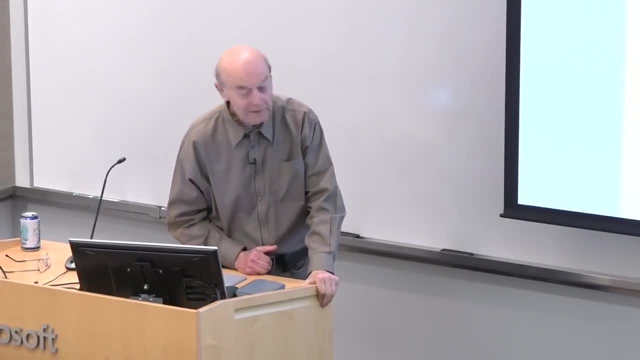 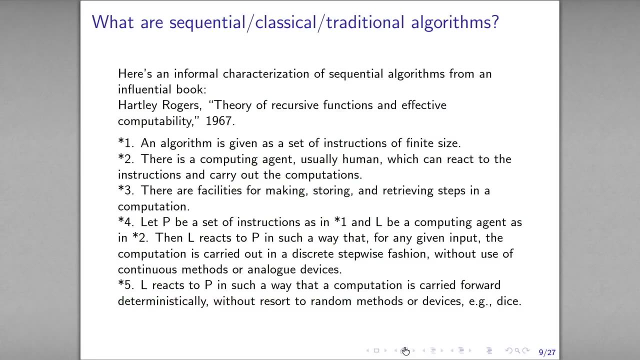 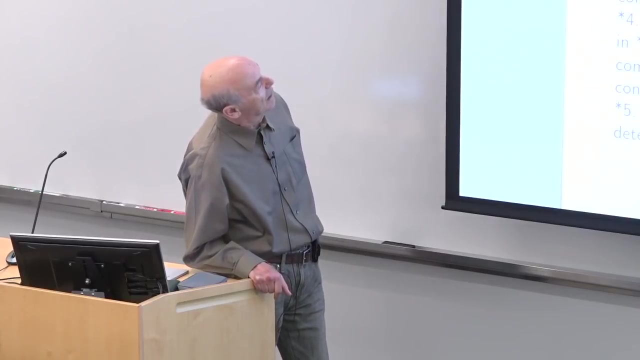 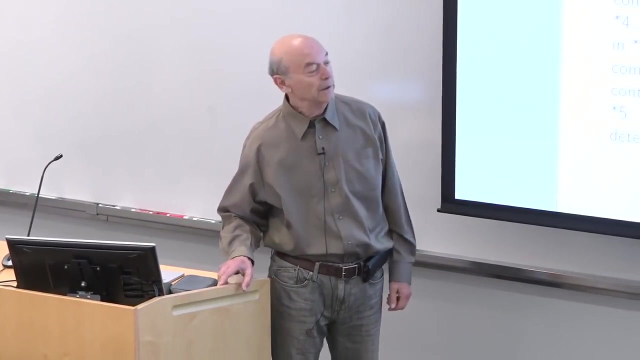 reasonably understood class of species of algorithms. you can extend this sequential thesis to this class. Now, what are sequential algorithms? So it's probably what you think they are, but here is a very influential book by Hartley Rogers, who taught logic in MIT. 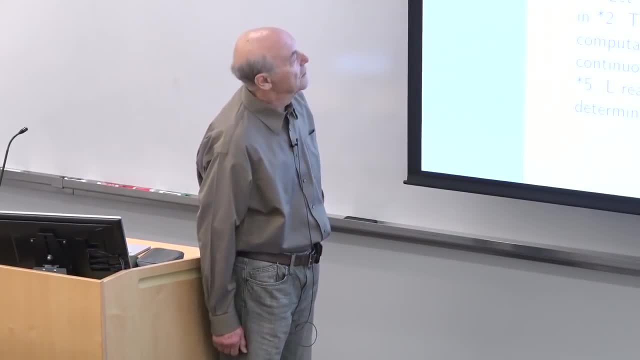 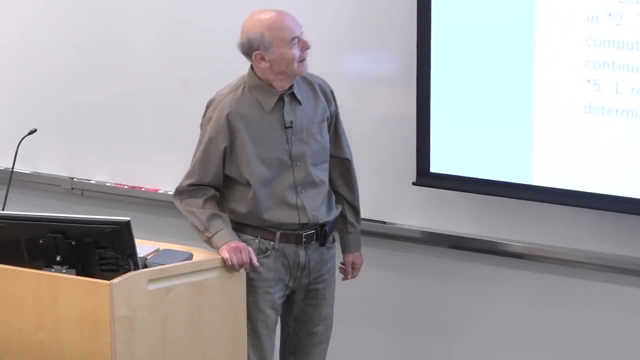 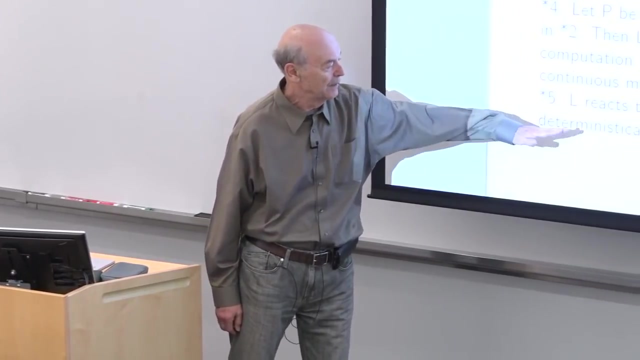 This is theory of recursive functions. the book In the area. So that's how he defined, and on page two of his book what he thinks informally. algorithms are So in particular, they are deterministic, without any resort to random methods or devices. 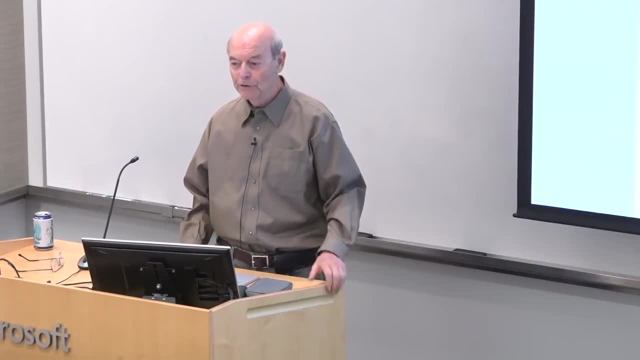 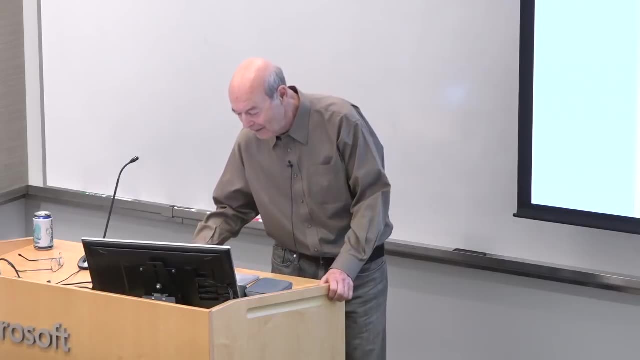 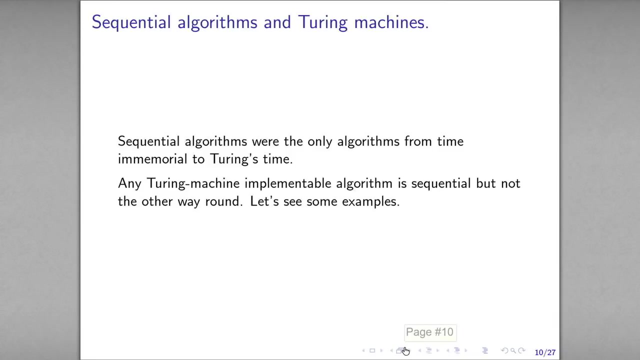 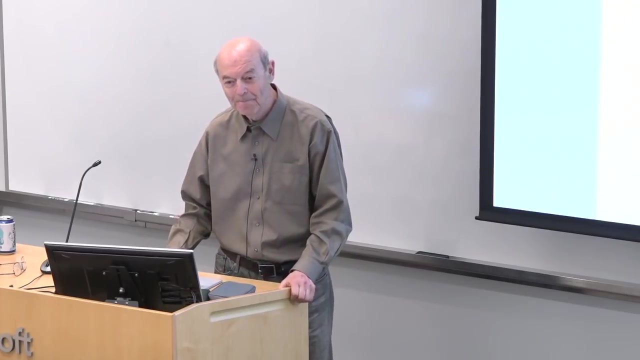 So it's not, as we acknowledge that we don't have probabilistic device in our algorithms. That's by definition. So there is often impression that Turing captured sequential algorithms, and that's not true. So I'll show you some very classical algorithms. 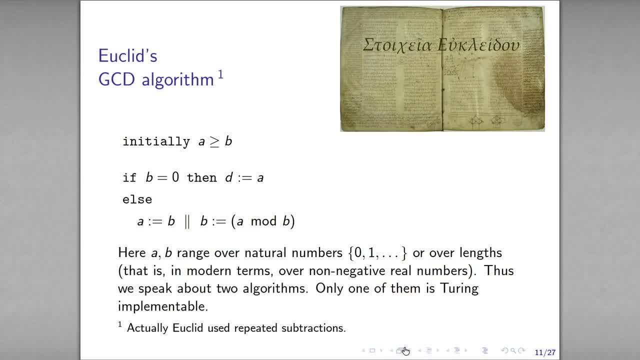 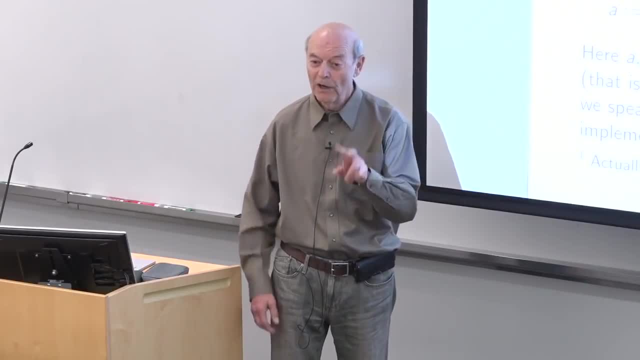 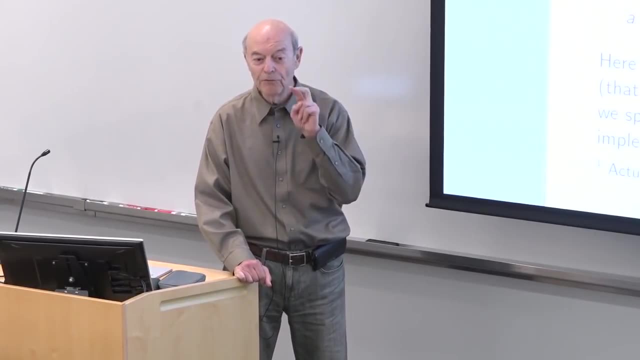 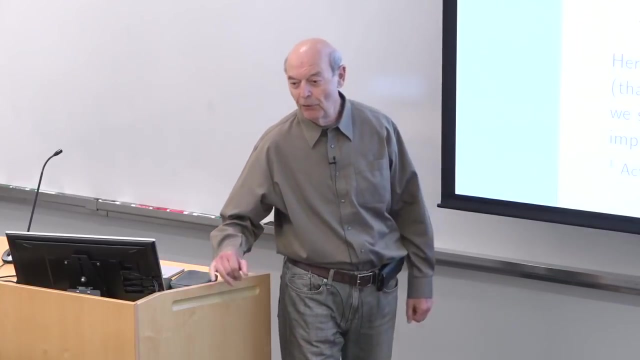 Here is Euclidean algorithms. That's the whole algorithm. But Euclid had two versions of it, One for natural numbers and another one for lengths. Today we would say non-negative or positive real numbers, but they didn't have the notion of real number. 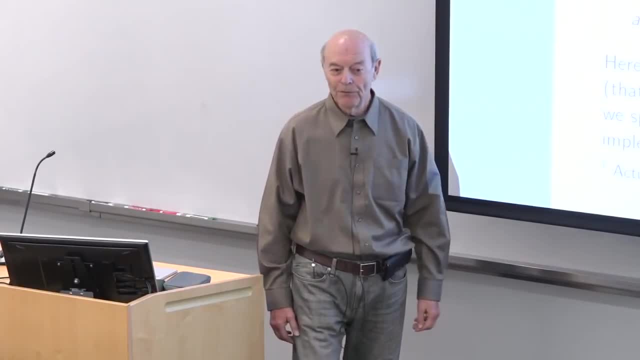 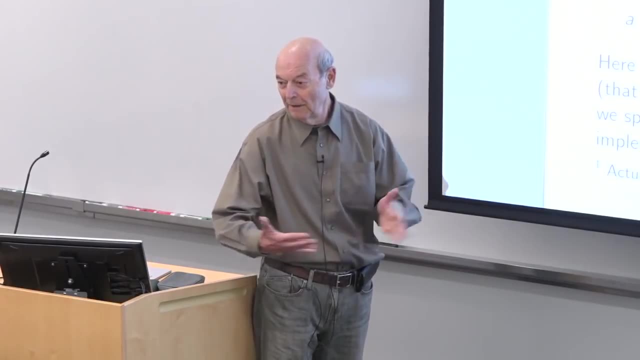 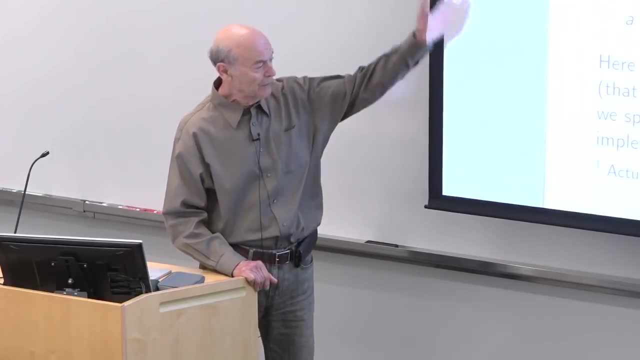 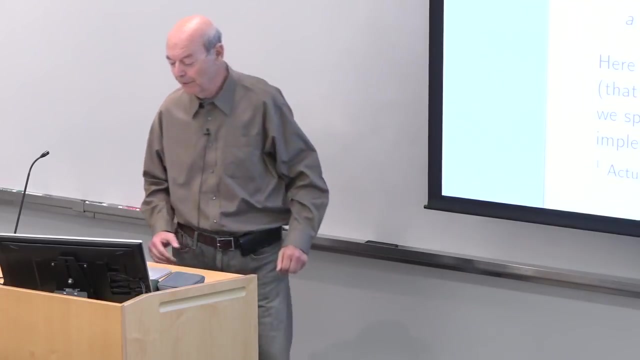 they had notion of length. So the version for numbers always converges. Version for length may not converge. It depends whether length A and B are commensurate, And only one of these two algorithms actually can be executed by Turing machine because it cannot deal with arbitrary length. 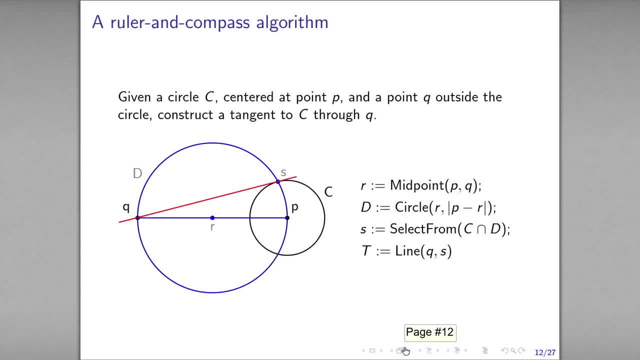 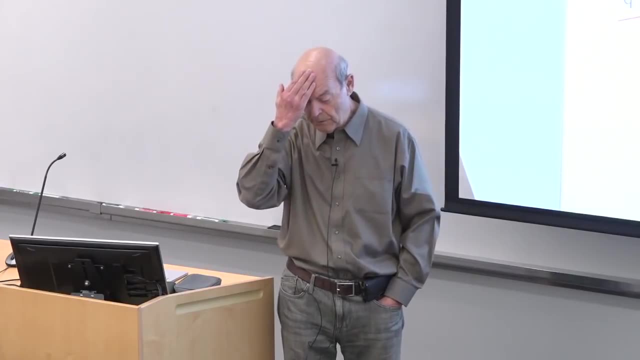 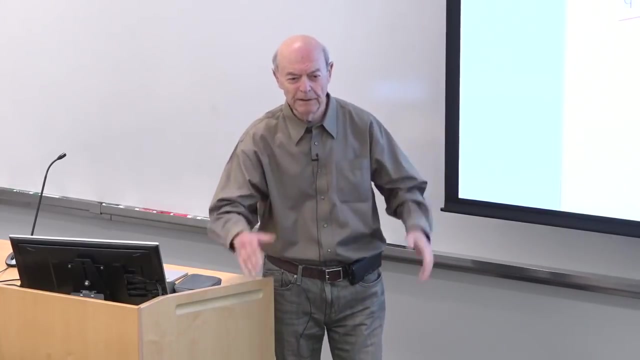 Here is a ruler and compass algorithm. Its picture comes courtesy of Wolfgang Rice, professor in Berlin. So he hair of Petri. maybe you know Petri Nets. He was the one who wrote a book on Petri Nets. For years he argued with me. 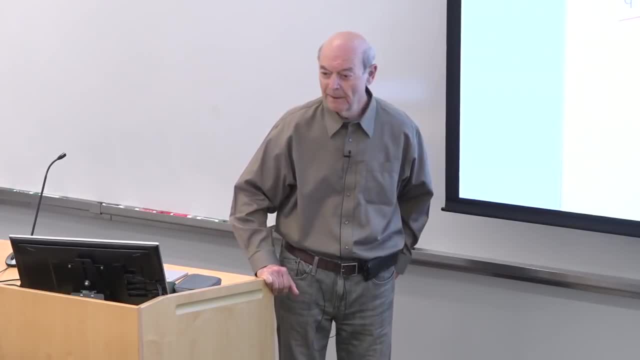 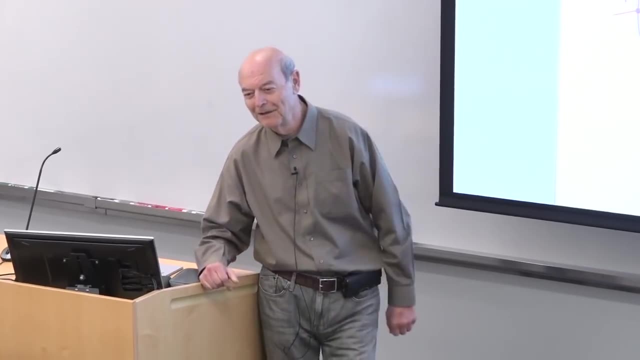 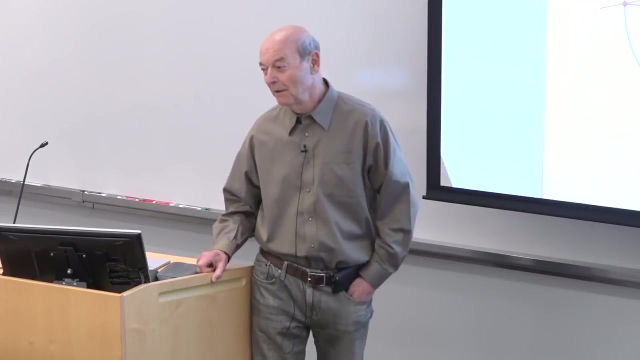 whatever you can do with abstract state machines, you can do with Petri Nets. Then at a certain point he started to write review and converted. He told me the story, one of the reasons for his conversion He said when he took a standard course where they 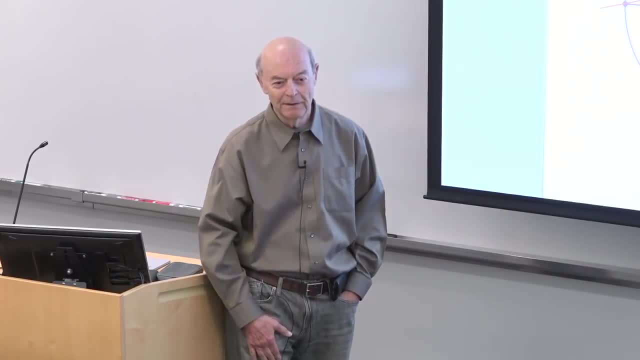 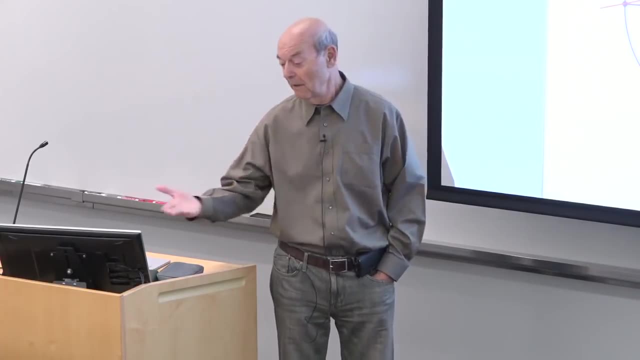 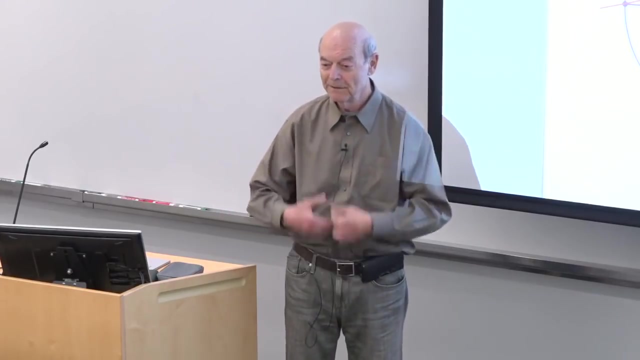 explain you regular languages and context-free languages in Turing machines. So the professor started with giving ruler and compass algorithm as an example of an algorithm. Then he went to finite machines, PDAs and Turing machines. He said I waited, He waited. 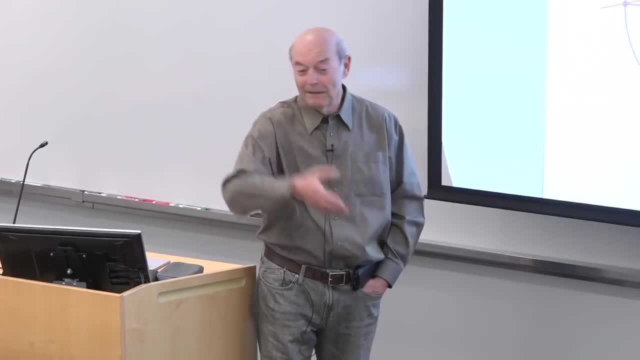 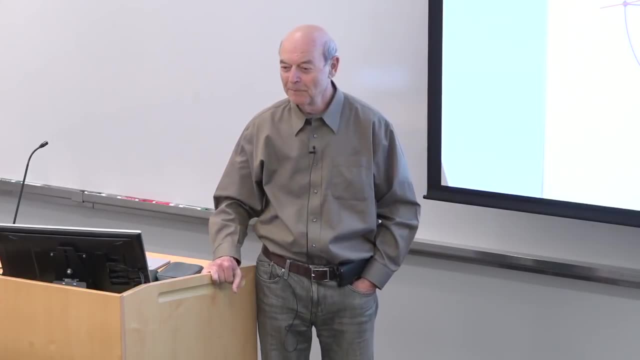 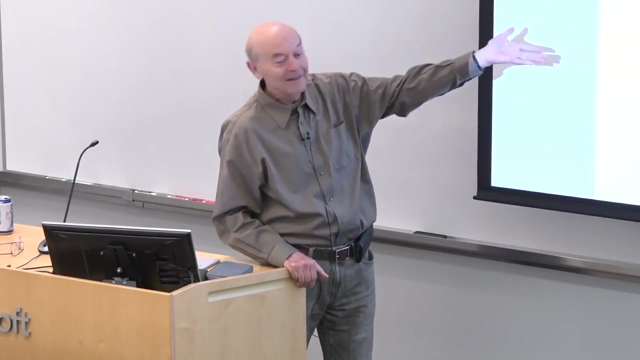 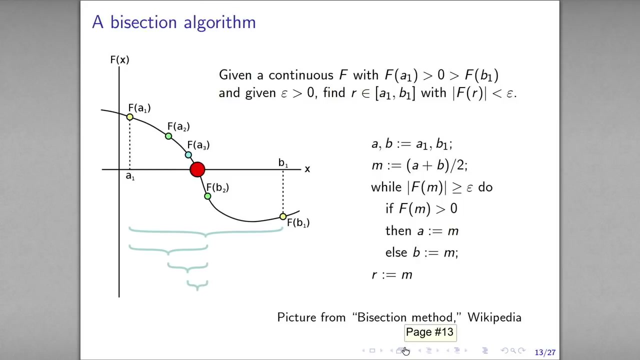 When he will return. So the last lecture he says. I raised my hand and asked professor, what about that ruler and compass algorithm? He said professor became very angry. So because you cannot put these things on Turing tape Bisection algorithm. or you can think: 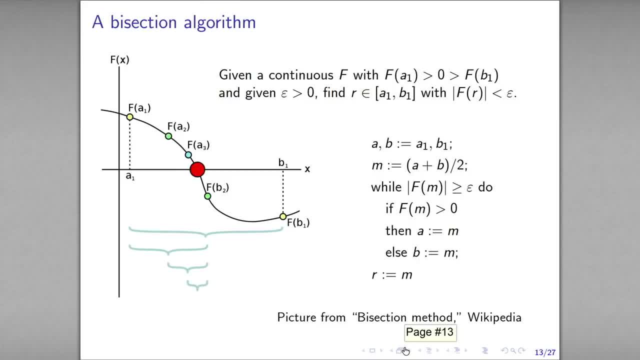 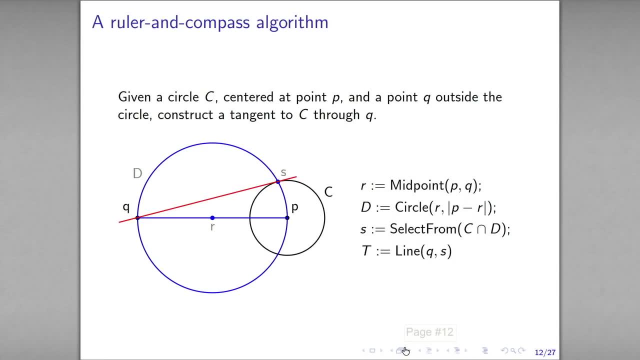 You can't put them on paper either, because there's noise, I don't know, but that's Arguably, I would say arguably. Turing had the right idea, because it captures the fact that you can't do this on paper. No, Okay, let me see. 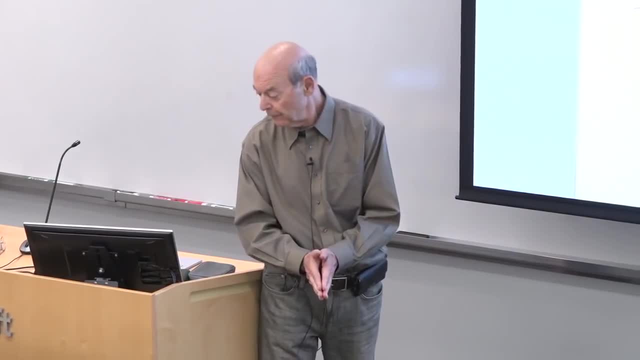 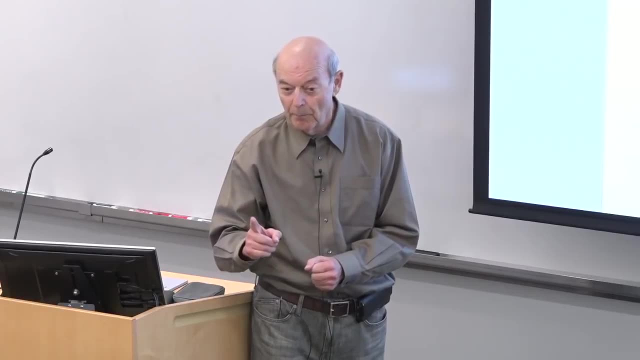 For the Greeks. when you look at Greeks, they always speak about ruler and compass. Why Didn't they realize that there are ellipsis and so on? They did, but ruler and compass was their computer, their computer. In their computer had noise. 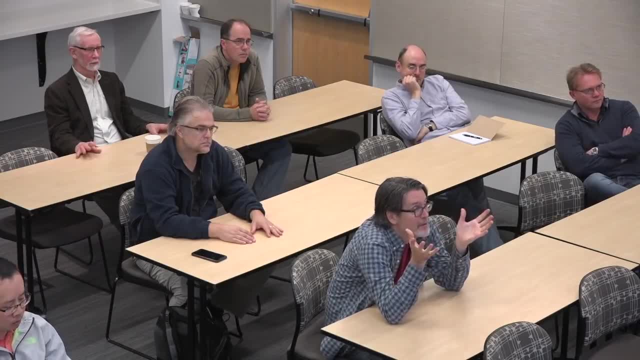 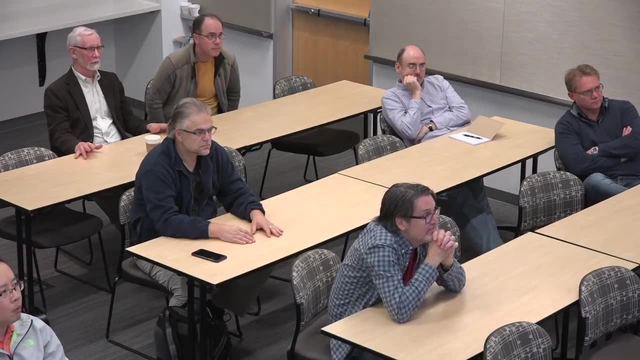 Yes. So if you think of the algorithm abstractly and mathematically, as dealing with real numbers, it's not true. That doesn't model the computer. Wait, wait, wait, We'll arrive to this. True, Any machine has noise. 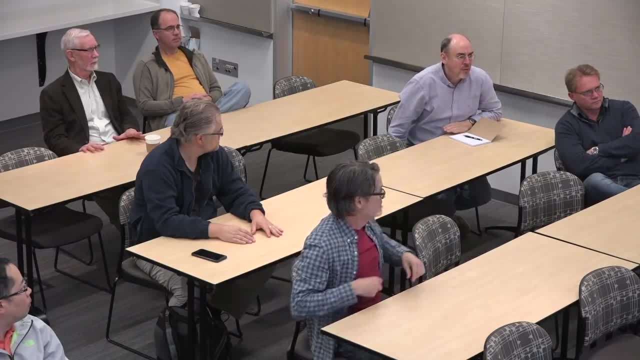 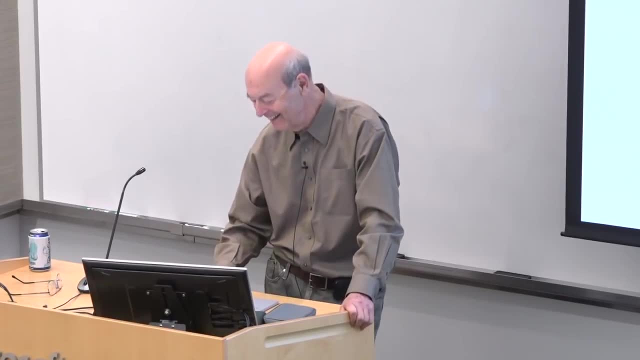 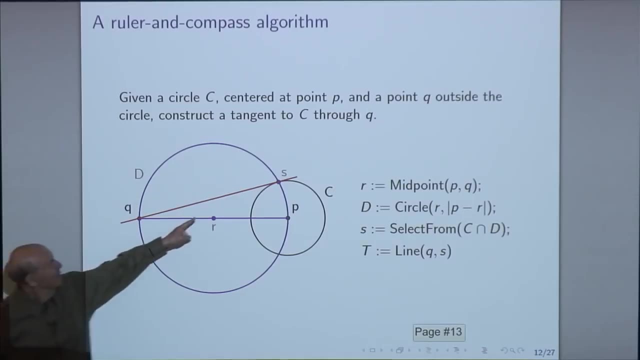 Another dimension is about non-determinism. Do you allow? Okay, I'll let you go, Yeah, Coming, There will be special slides. In fact, here there is a tiny non-determinism. There is a choice between this solution, that solution. 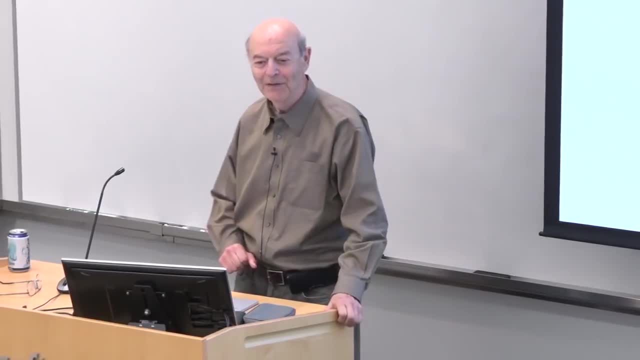 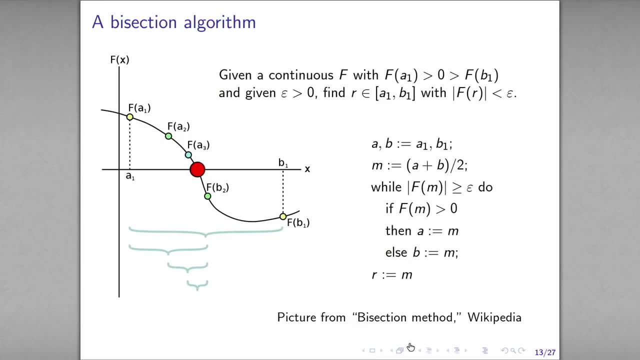 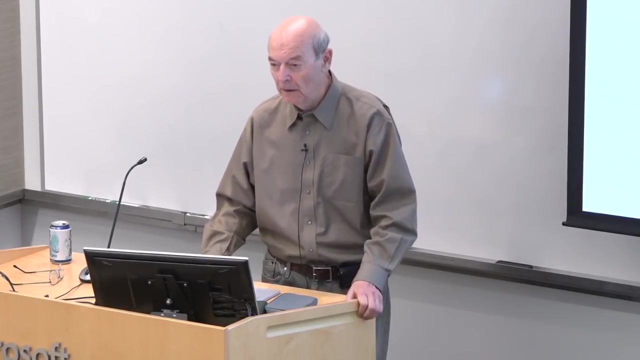 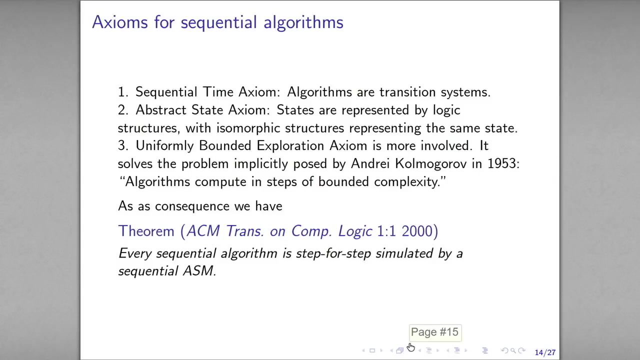 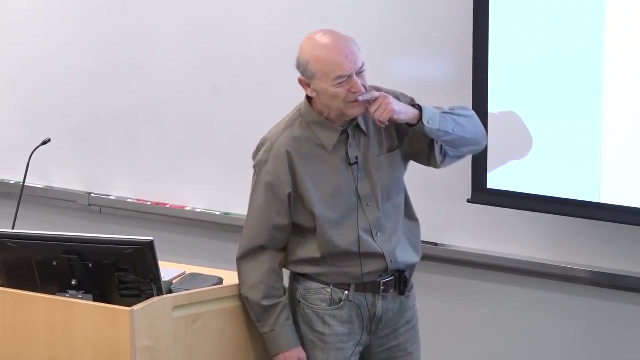 But in classical theory they just ignore that. So you can think bisection algorithm or Gauss elimination problem. Now you can approximate them with arithmetization, but you don't capture them as if faithfully as is. So it turns out that from my point of view 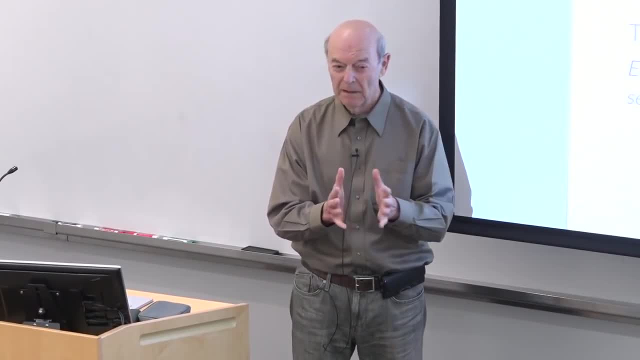 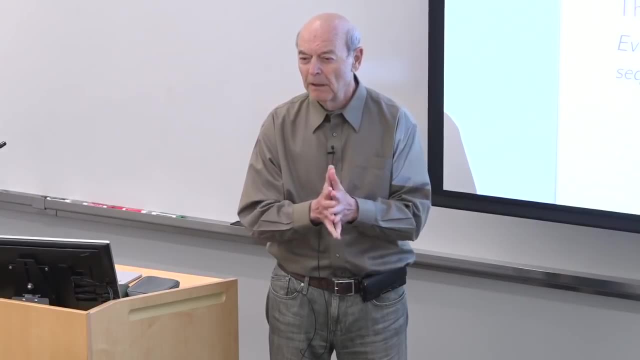 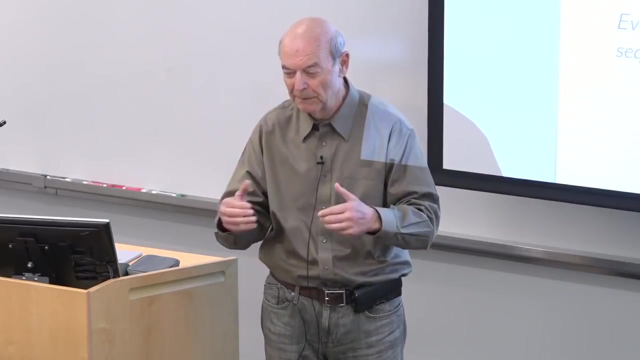 So the problem- how to axiomatize this, classical algorithms- was there from the beginning. So in his beautiful paper Turing does a lot of axioms. He doesn't think in terms of axioms but he says without loss of generality. 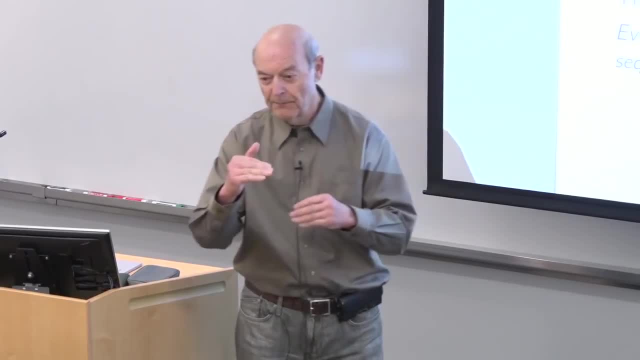 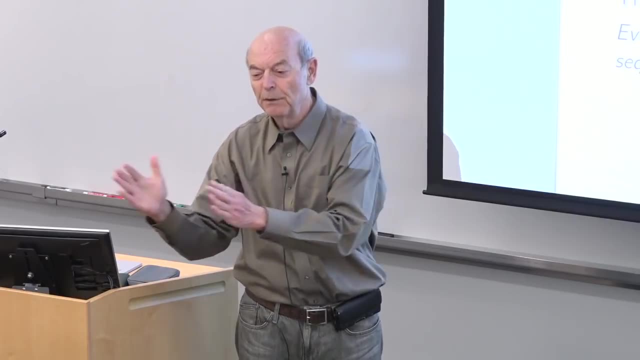 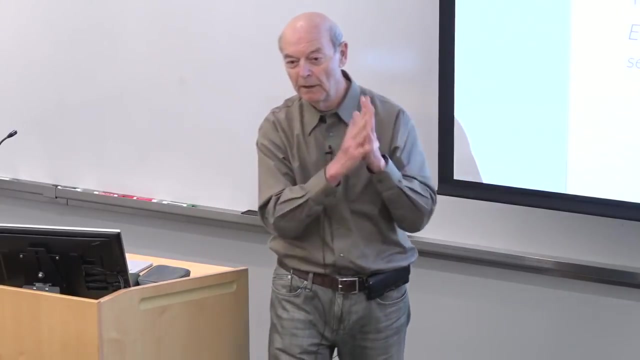 So, for example, the very first sentence in the key section is: we compute- I forgot exactly, but by pushing symbols around. So from very beginning he restricts the safety of symbolic algorithms, Ruling out, for example, rule and compass. 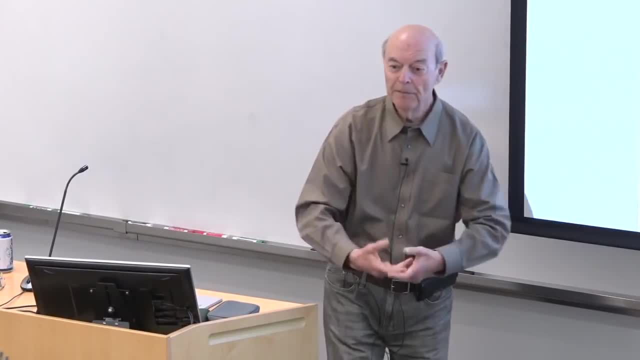 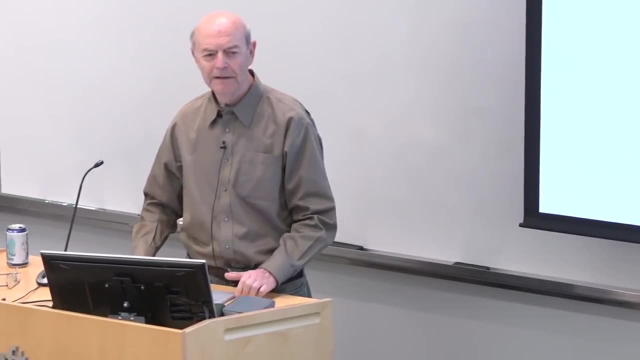 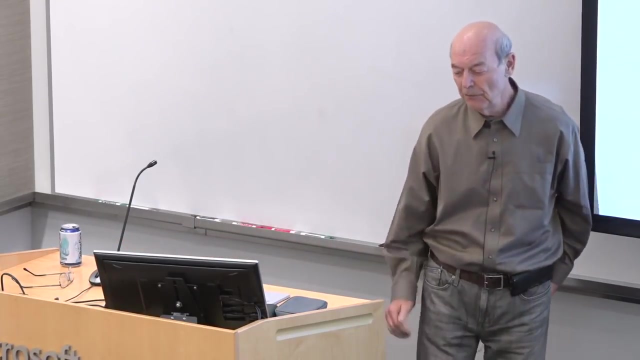 And as it goes he made, there's only finite part of the brain is involved. So he made strange things. They're all justifiable, but obviously too many of them. I think the problem was difficult because they didn't have a proper abstraction. 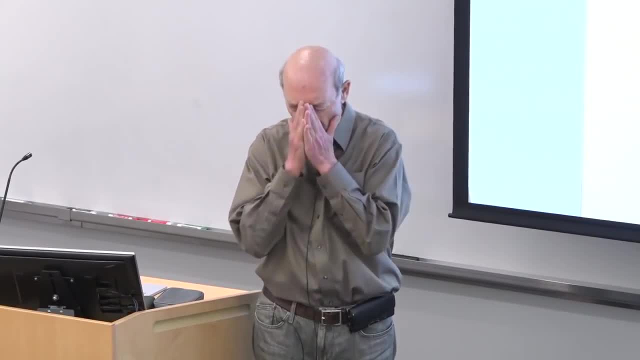 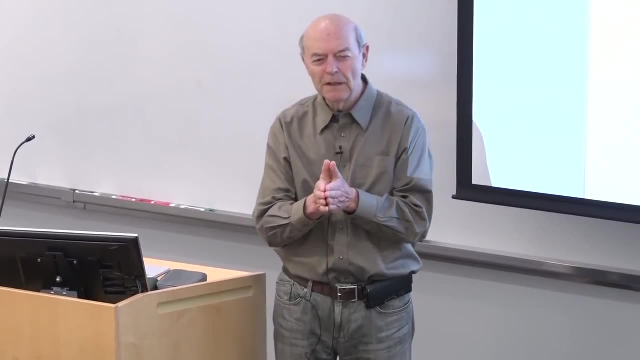 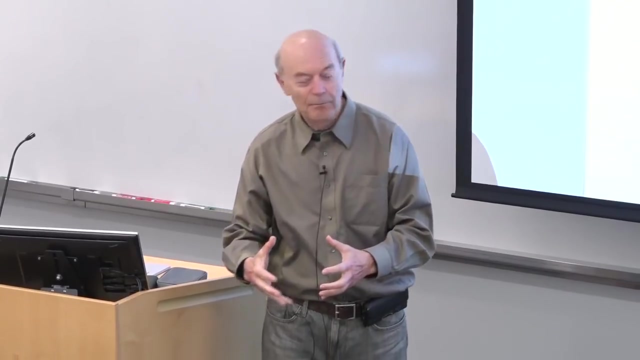 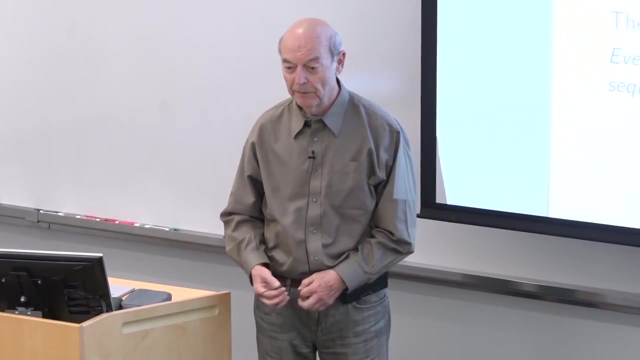 They were. that's actually relates to your point. They were thinking about algorithms which actually compute one way or another, something more or less real, But the simple axiomatization turns out to be on a much higher abstraction level when you deal with abstract structures. 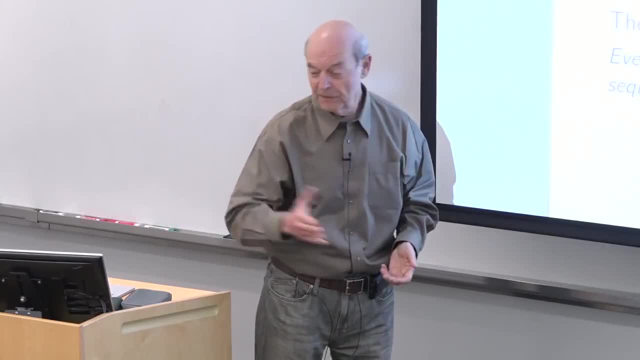 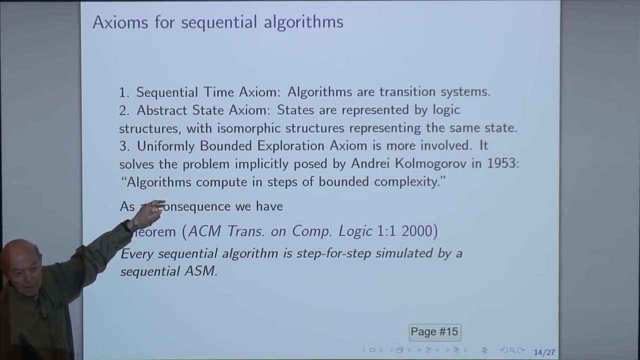 say abstract structure of the reals. okay, That's why you can deal with rule and compass, because so this is abstract state. So when I started to think about this problem- the first is trivial, second came to me sort of obvious. 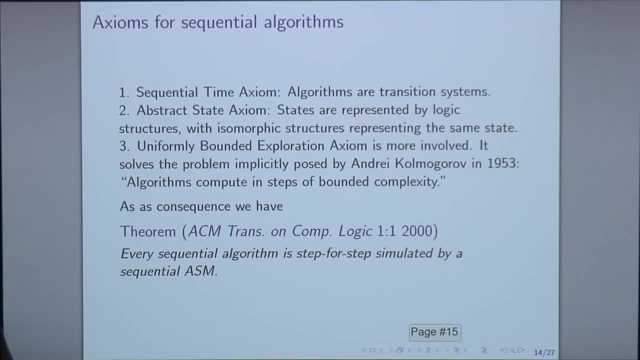 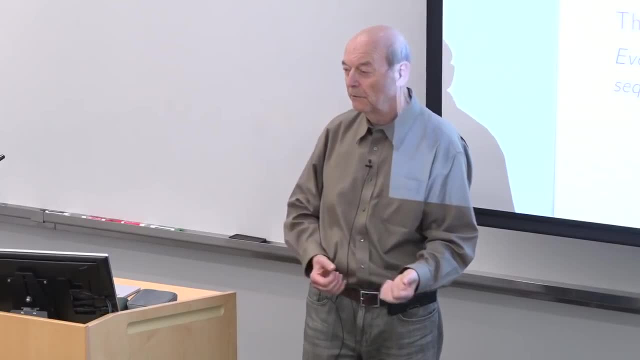 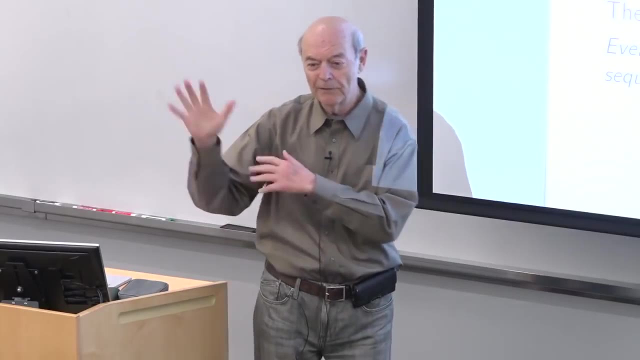 thanks to just being a logician. Any mathematical reality which is static is a kind of structure. So if you go to University of Washington, capture some mathematician and ask him what he is working on? some kind of structures, topology graphs. 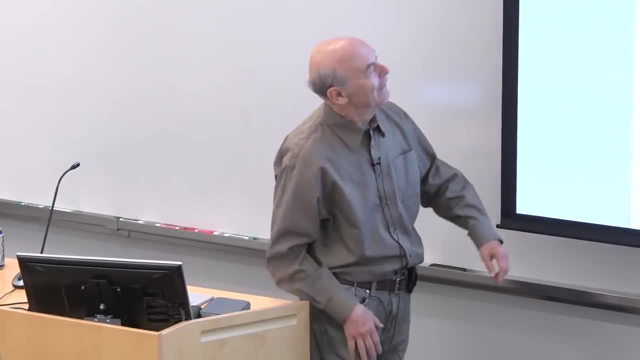 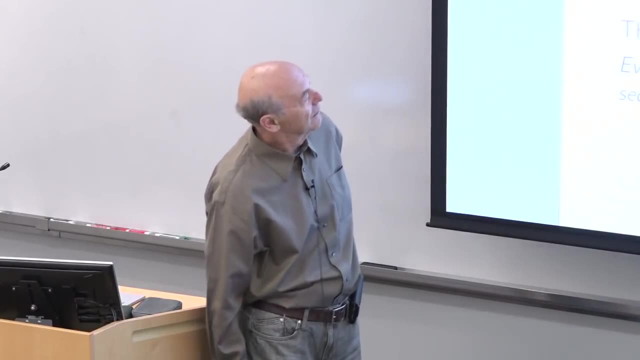 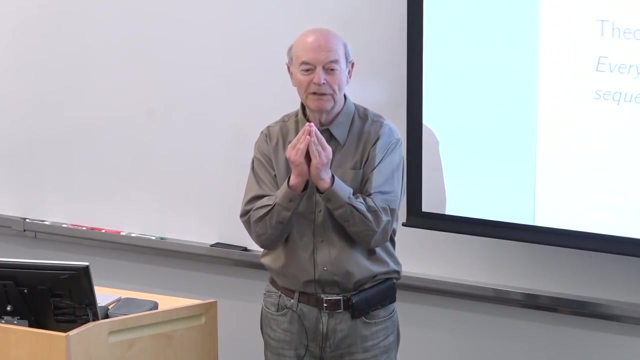 whatever, but some kind of structures, Okay. The third problem was difficult. It took me like 15 years, And so Kalmagorov thought about this, what he said, that steps should be of bounded complexity, Each step, not a number of steps. 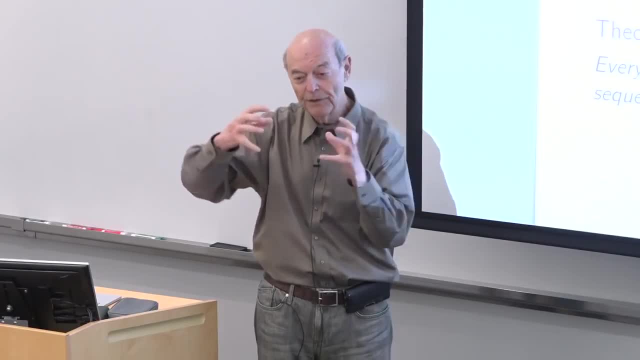 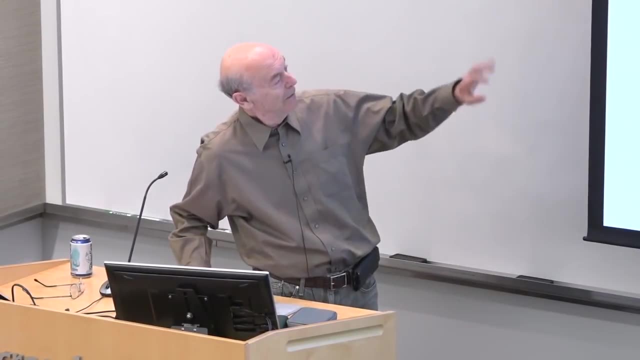 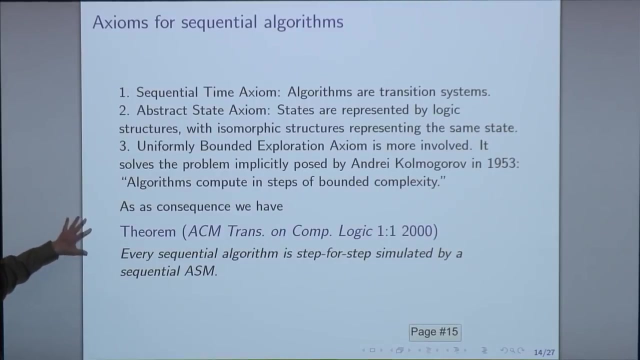 but there should be bound on the complexity of a single steps. So that was a challenge. So, if you wish, at the end I can explain the axioms. But so if you take this axioms, then every sequential algorithm is this: 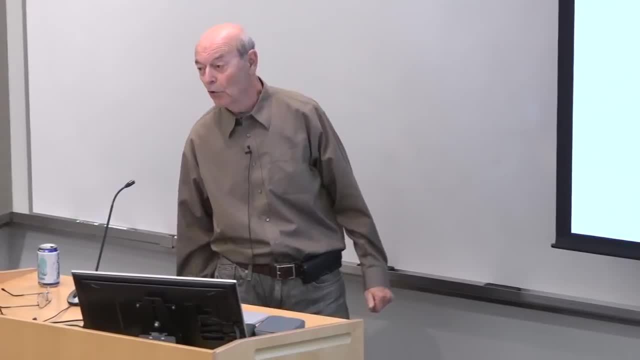 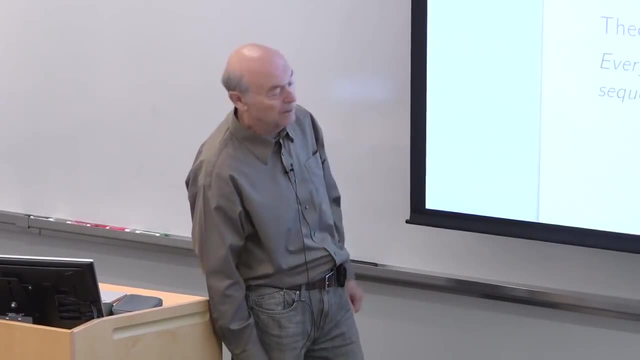 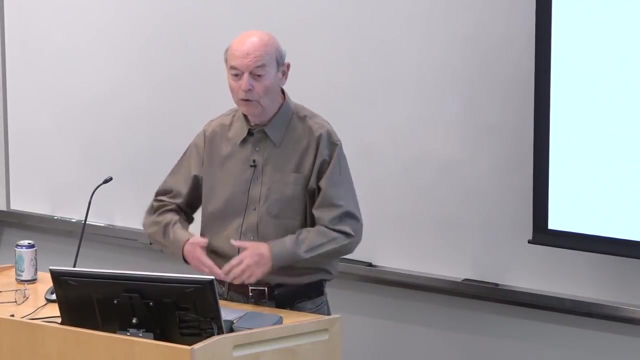 So Shor says that axioms probably are wrong. No, I don't know. but for all these years- 18 years, so there's quite now a substantial ASM community and they tried all kind of things And there are various people, from mathematicians to engineers. 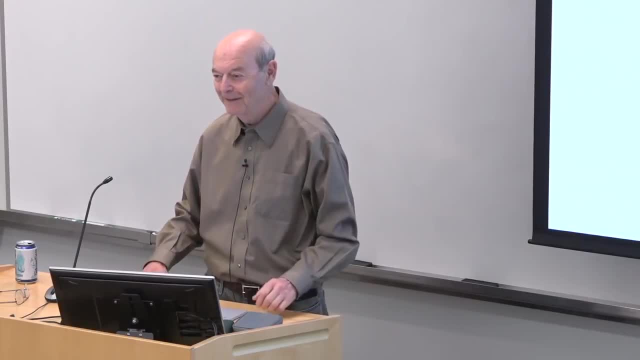 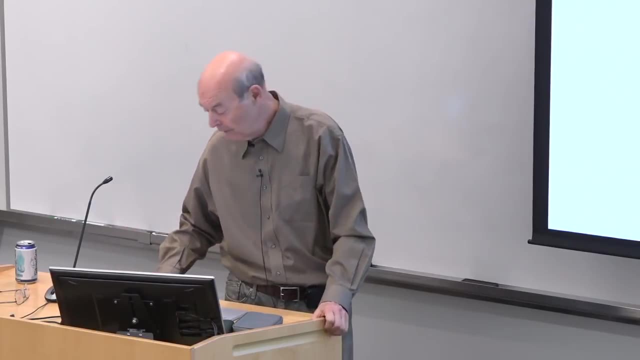 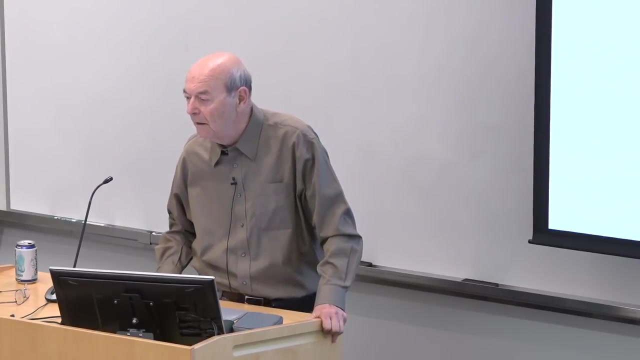 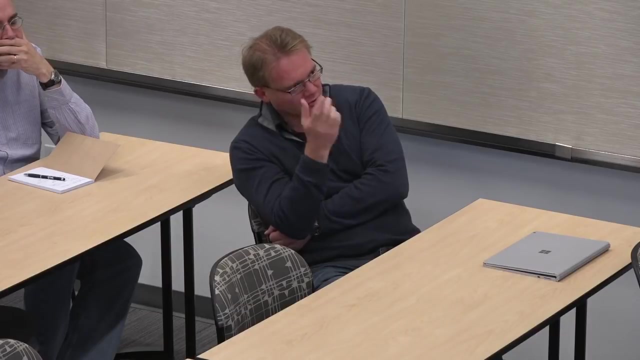 very engineering people, computer scientists, And so nobody came across an algorithm which wouldn't, whether it's very high-level or low-level. So Rogers had the axiom of not using continuous functions. Yes, Yes, Yes, Is some precursor or it's a weaker statement than-. 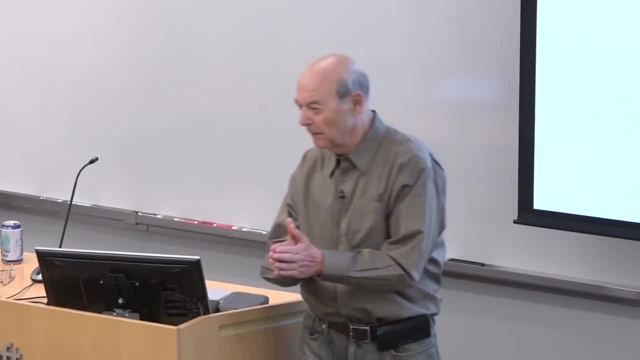 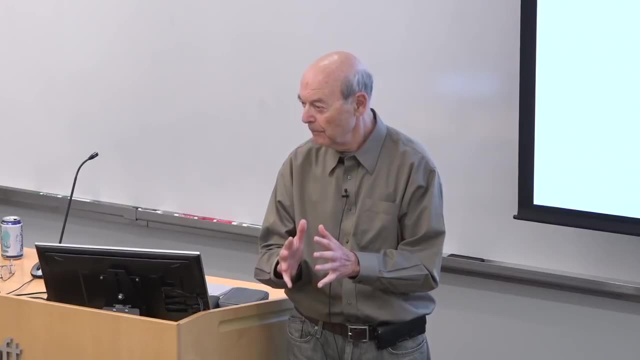 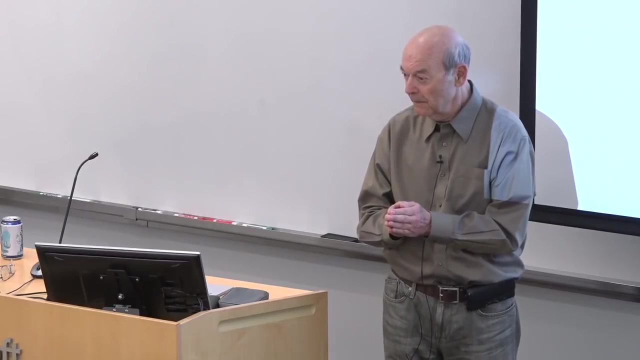 Yes, Yes, Because they all thought- let me give another example much more So. there was a school of mathematics called constructivists, And constructivists said that only computable numbers exist, And they started to develop mathematics, alternative mathematics. 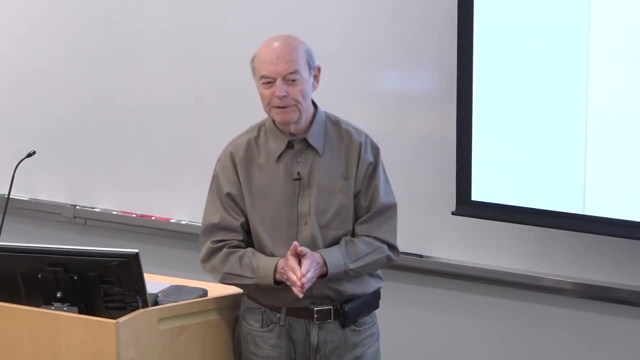 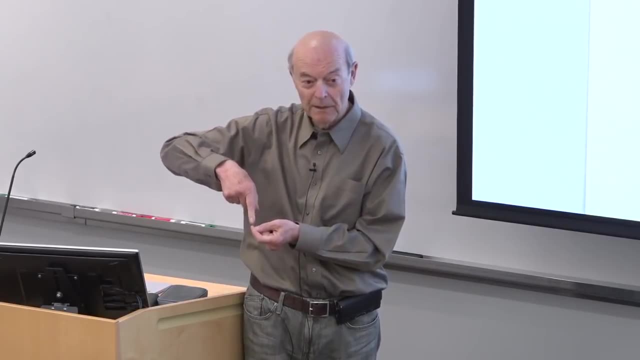 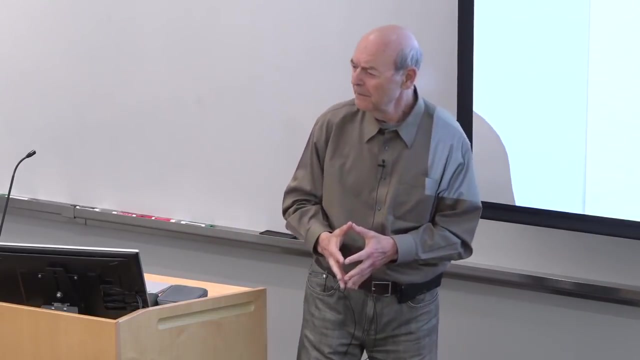 Certain theories were false because you say that always there exists a maximum, say the Bayer-Strauss theorem, But this maximum may be reached in a non-computable real And in their world this theorem fail. Okay, There's a very interesting. 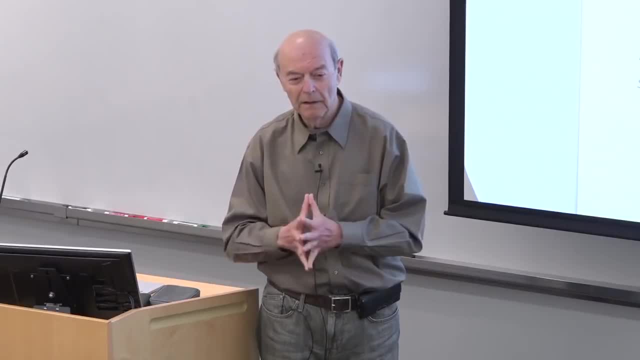 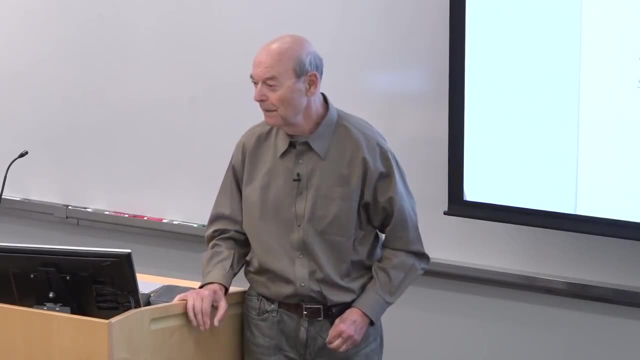 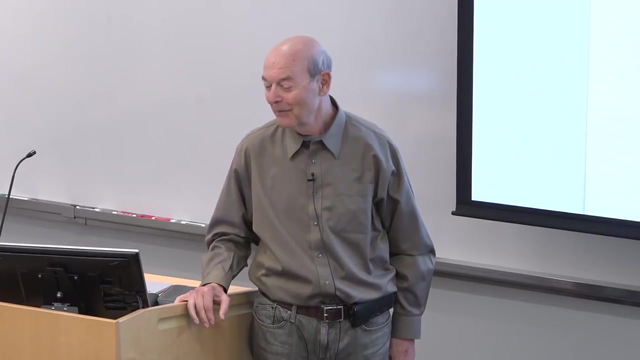 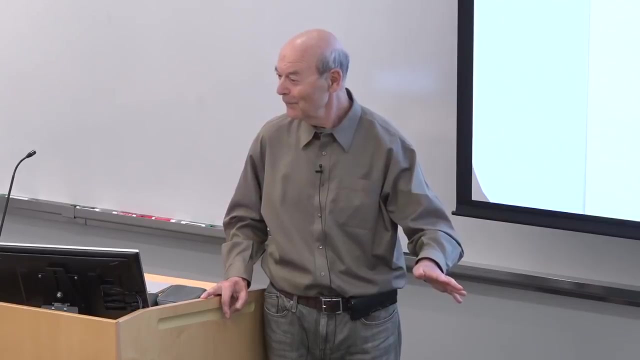 our famous whale. Herman Whale, the hero of quantum world, was a constructivist in his young years And he had a bet with Polya. So he predicted that in 20 years the Bayer-Strauss theorem will be false. 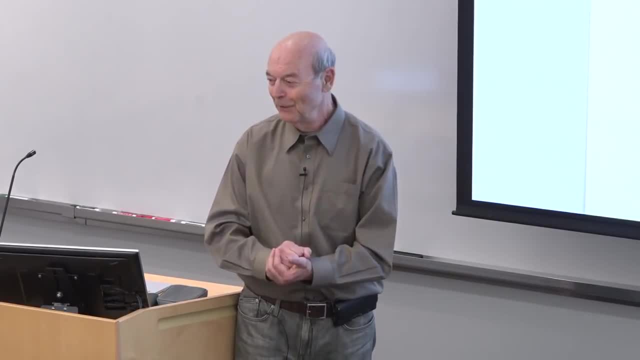 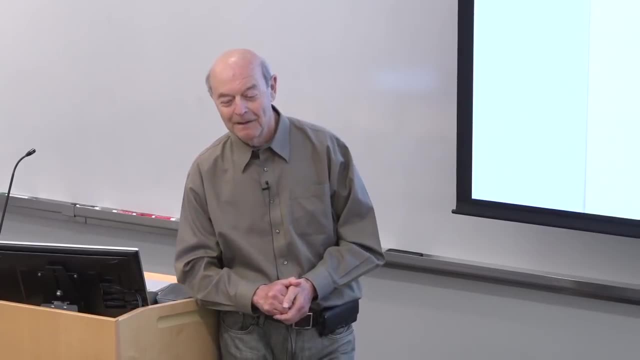 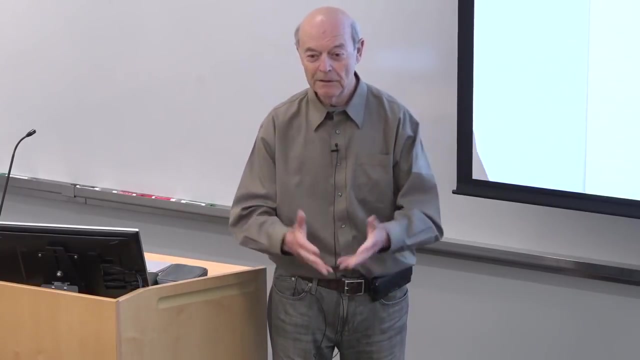 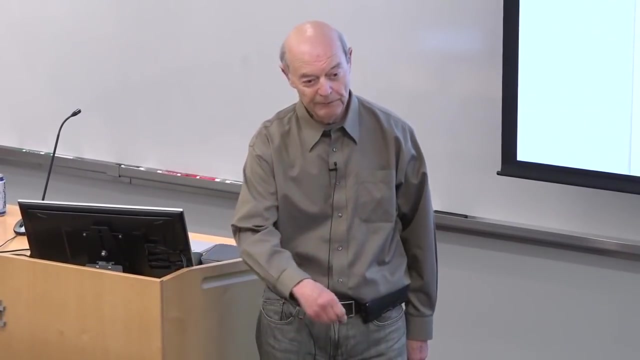 And so this bet was done at the high university in Zurich, ETH, And so very famous people signed it. So I can tell the story. I was in ETH visiting a colleague and I see something in German on his table And I see many famous signatures. 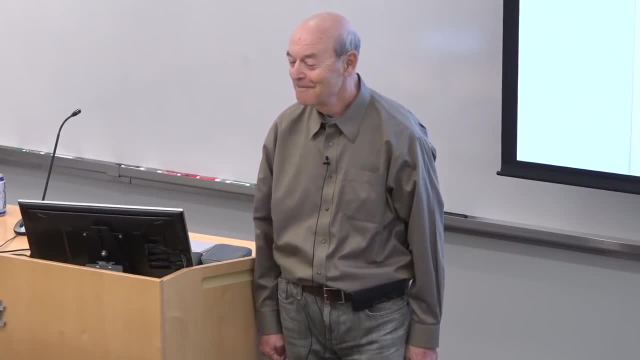 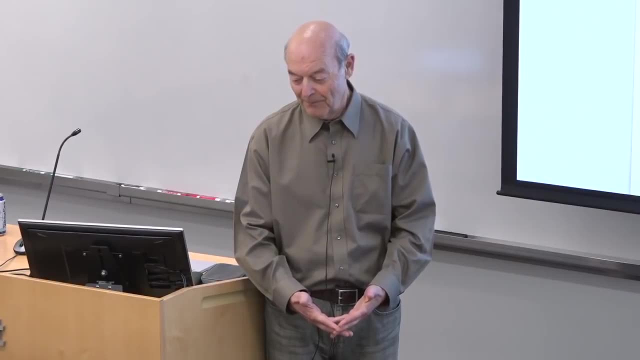 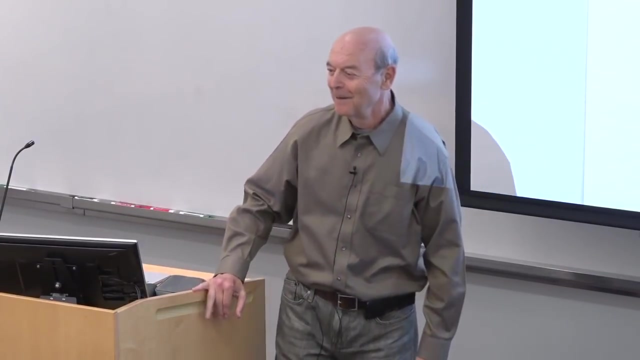 I say: what's that? He said that's the bet. So he tells me the story And I decided to. I wrote a little. I have a column in some journals where I wrote an article about this. asked somebody to make a good translation. 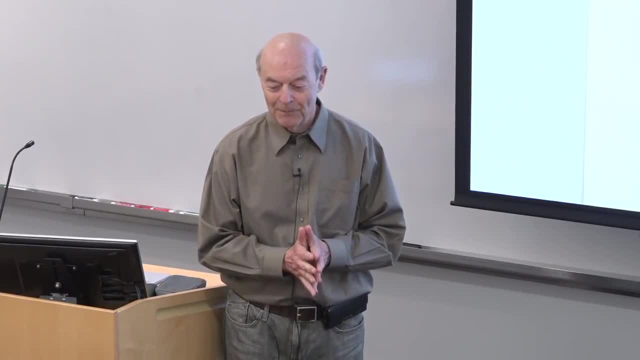 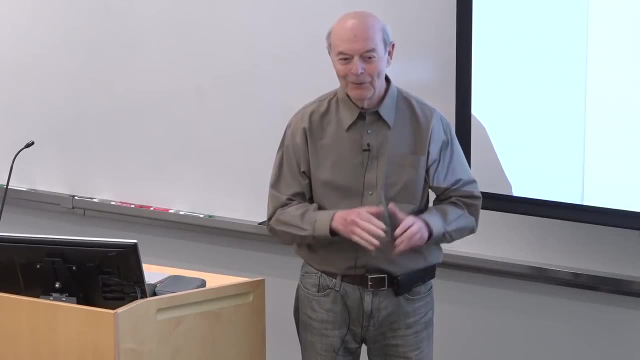 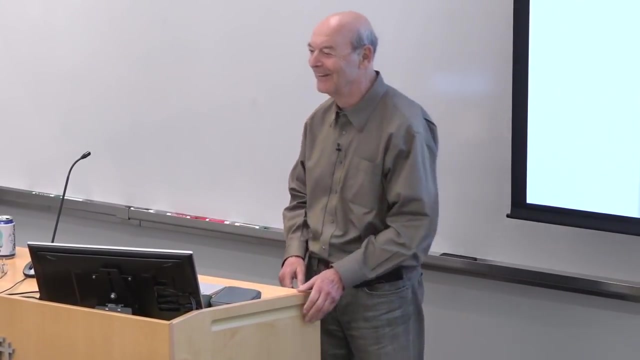 Then after 20 years it was close to war, I think in 1938 or already with the war. So Herman Whale came to Polya and said: let's just forget about, or something like that. So according to the bet, 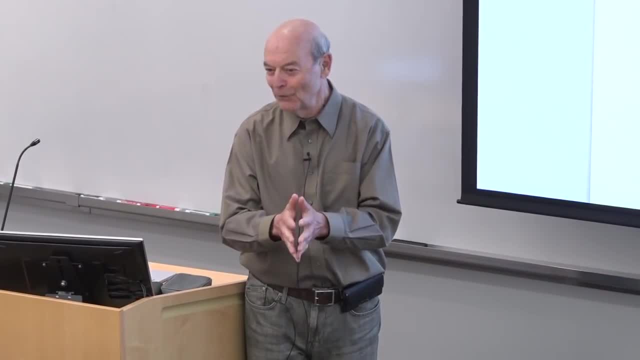 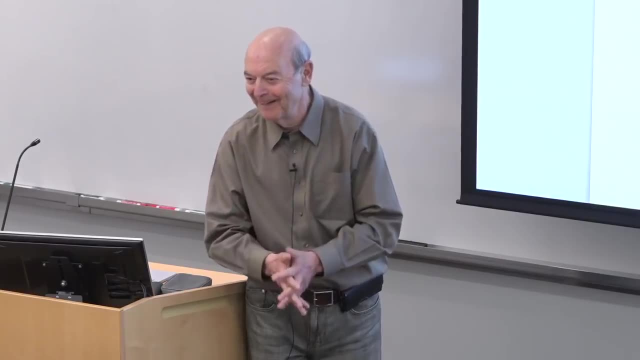 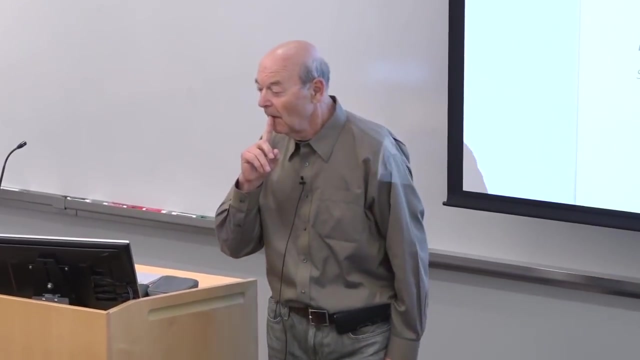 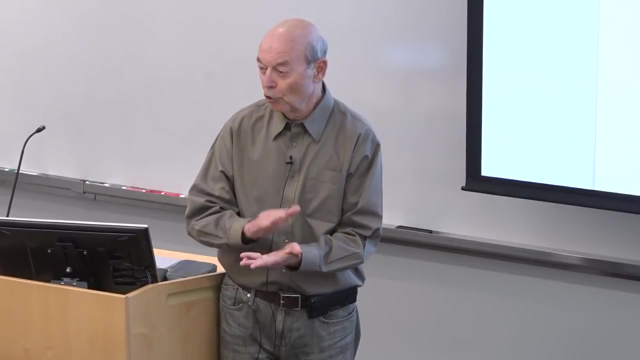 he was supposed to publish. the one who lost was supposed to publish in one of the best mathematical journals acknowledgement that he lost the bet, But this never happened. Okay, So what was the problem? So I have another article. I say why constructivism is wrong. 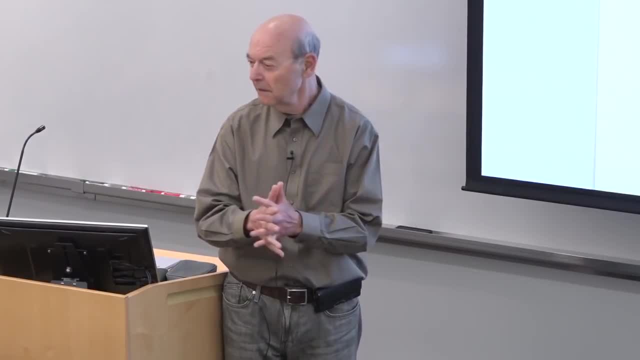 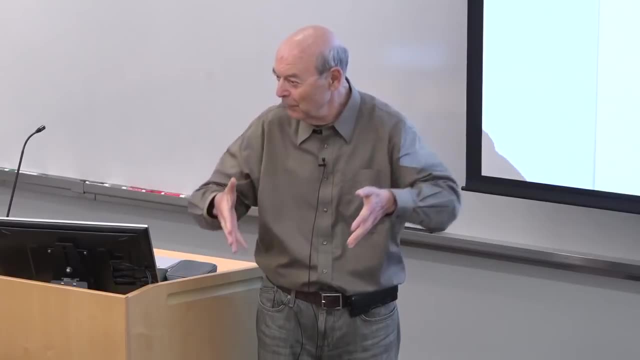 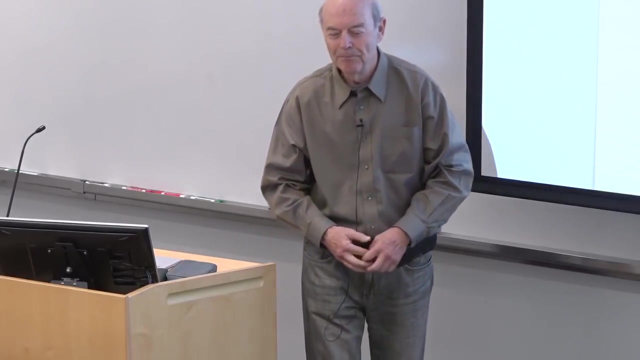 It's not another respectable approach to mathematics, but it's just wrong. Why it's wrong? Because they were fascinated by this recursivity, by Turing computability. But the real world is different. So they made some beautiful theorems. 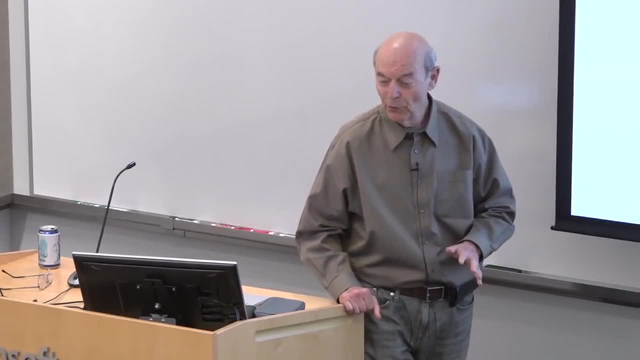 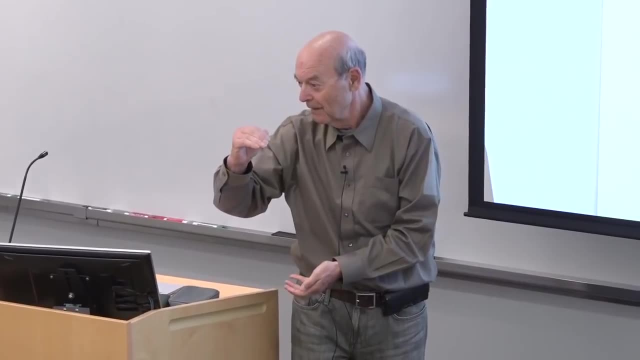 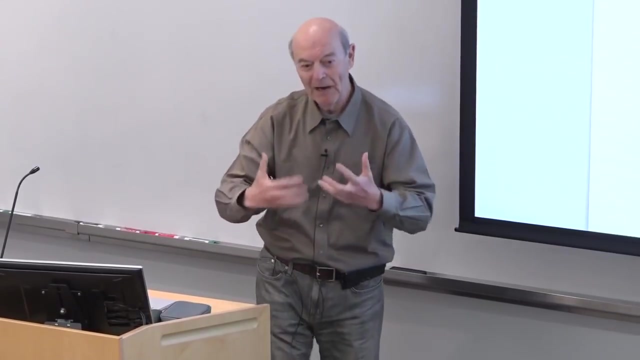 They were there much before complexity theory and knew a lot, but they were not interested. They were fascinated by this level and that's the level where Rogers is. So in the beginning they all were fascinated with this working on this level where everything is somehow feasibly. 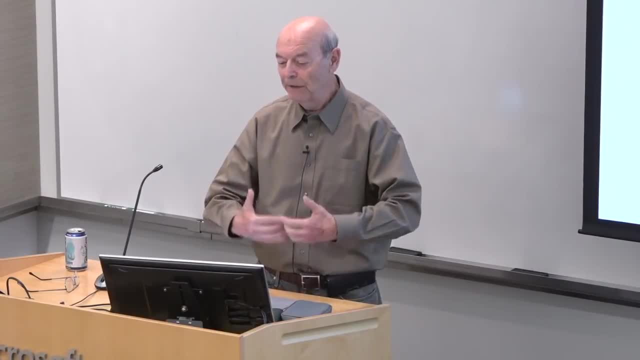 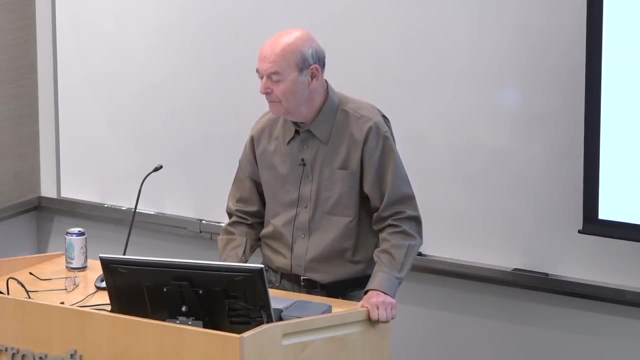 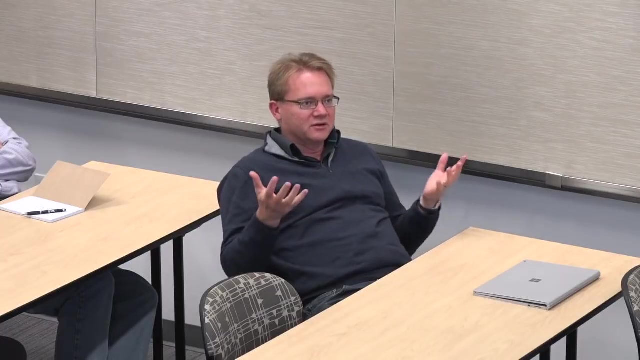 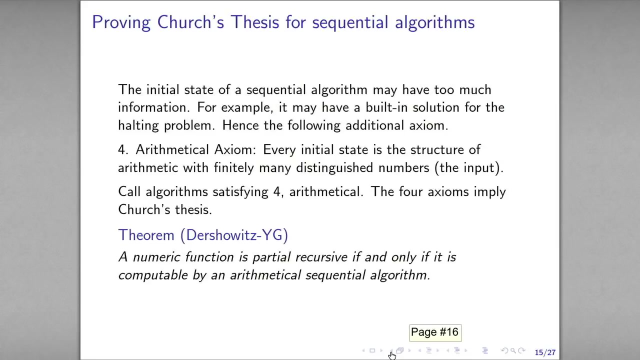 not feasibly. feasibly in the sense that you can execute steps in a feasible way. Does it make sense? Sure, But I mean, my take away is that it's a general statement to make about these, whether it's continuous computation. So there is no obvious contradiction. 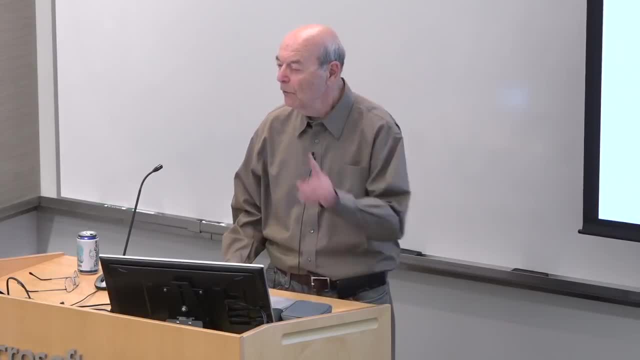 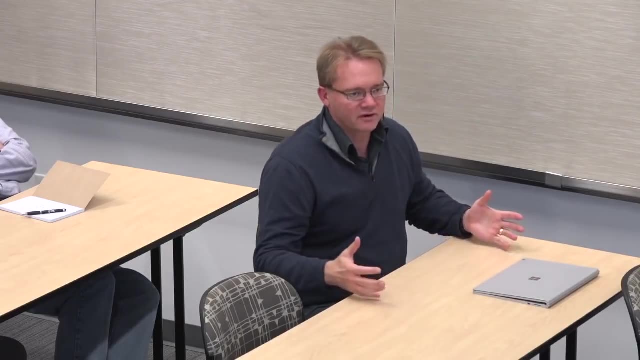 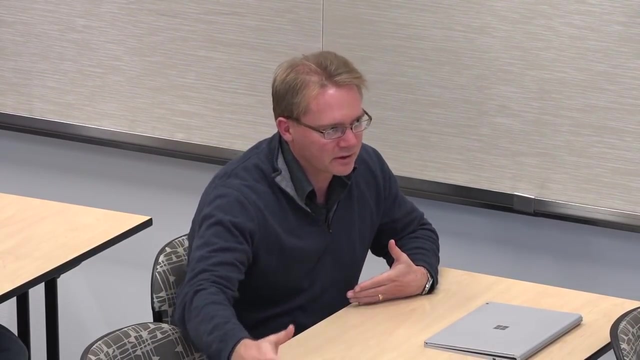 it depends what's continuous. So what he was ruling out, okay, Well, you're ruling out making an infinite number of changes in one step or a growing number- Yes, Unbounded number- growing number of changes across steps. So essentially ruling out analog algorithms. 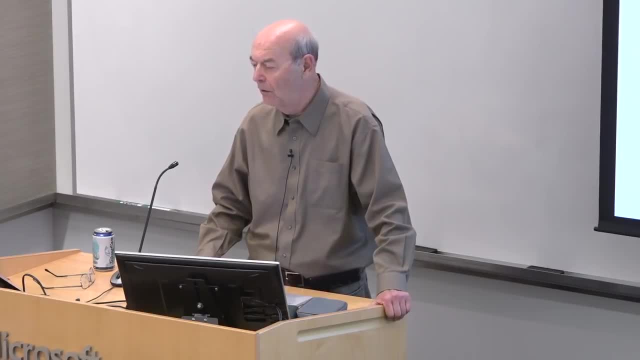 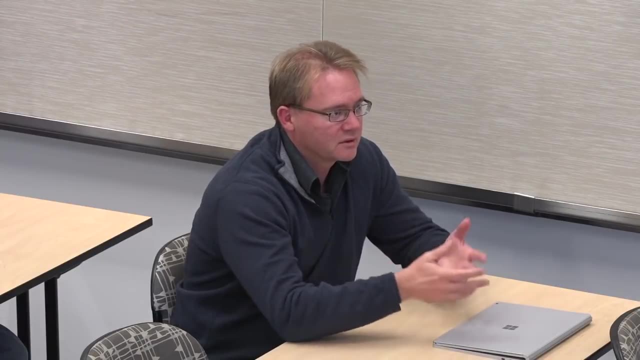 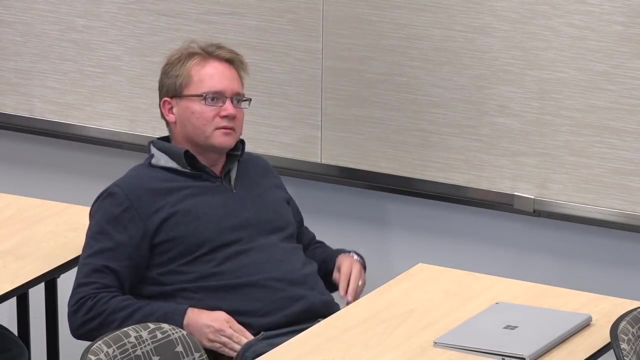 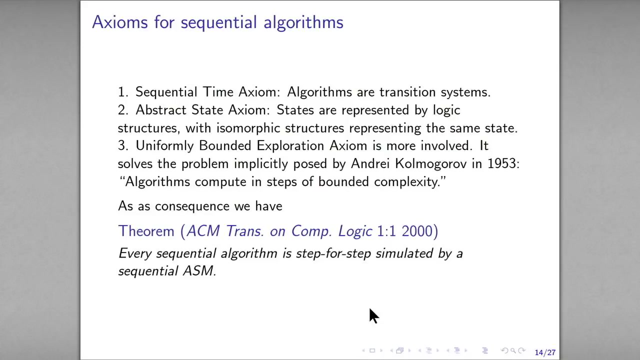 That was his goal. Yes, but number three rules out not only analog, but by the general statement I mean so, all right. So I didn't understand. what do you say? The starting point for my comment was that number three is: 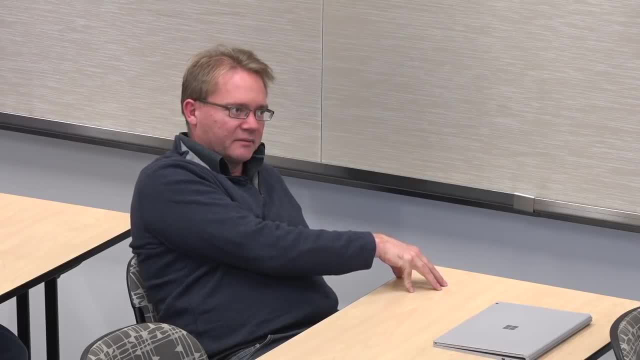 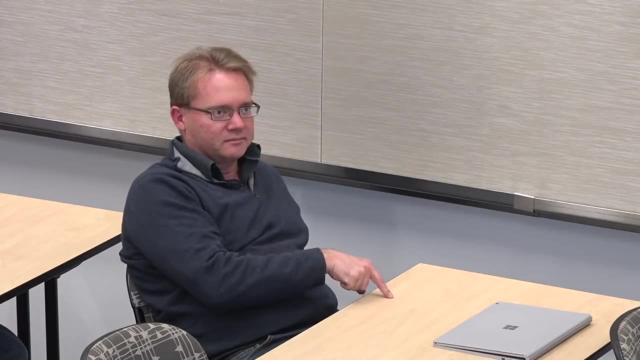 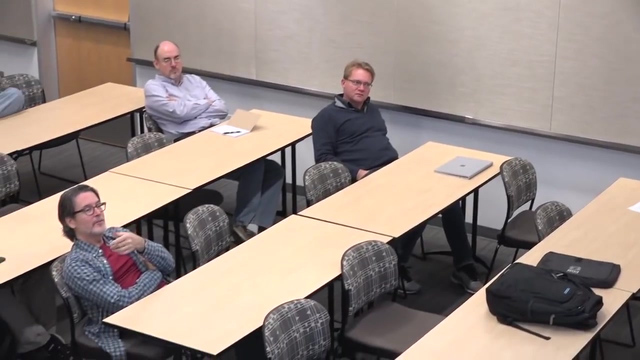 a generalization of Rogers and number four, where it was sort of analog and continuous functions, Probably Mm-hm. So what is the definition of bounded complexity? I mean, I read the term complexity and usually to me that depends on a model of computation. 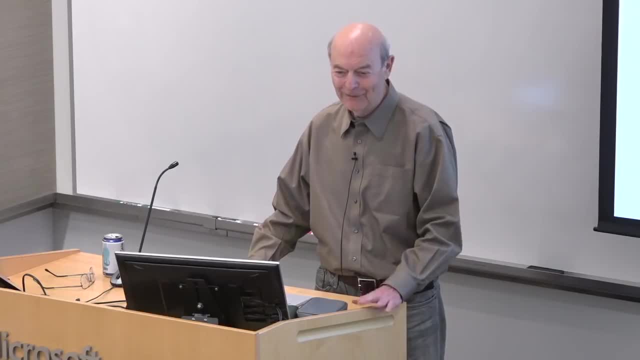 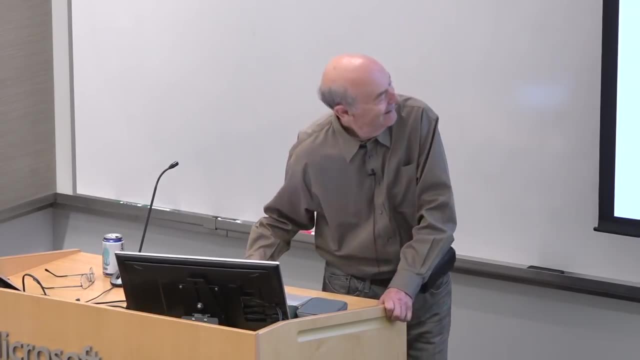 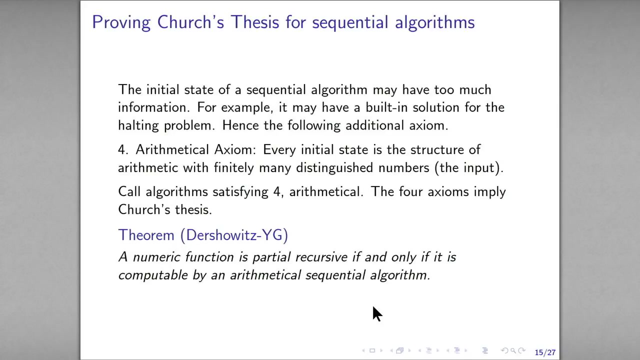 So what does complexity mean? Let me leave it after I come to bottom line, because otherwise I will now finish. I'm sorry, I'm happy to talk about it, but so let me see. So Nahum became one of the most active people. 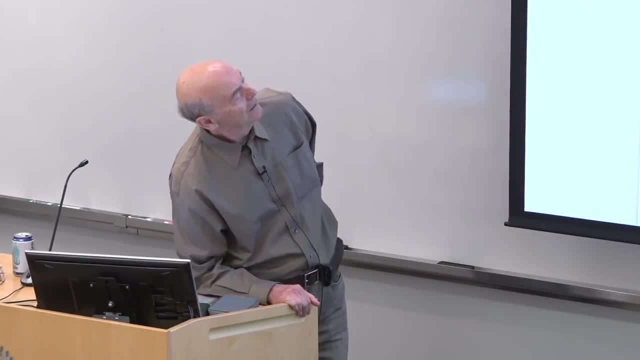 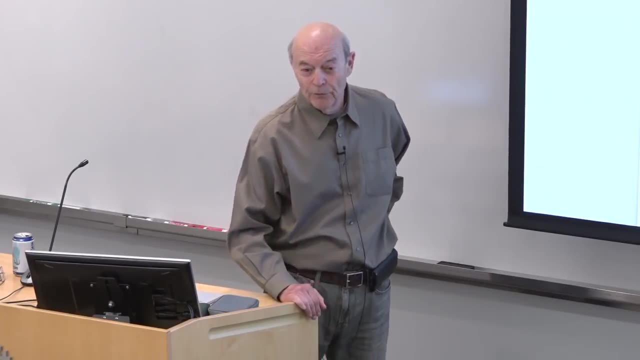 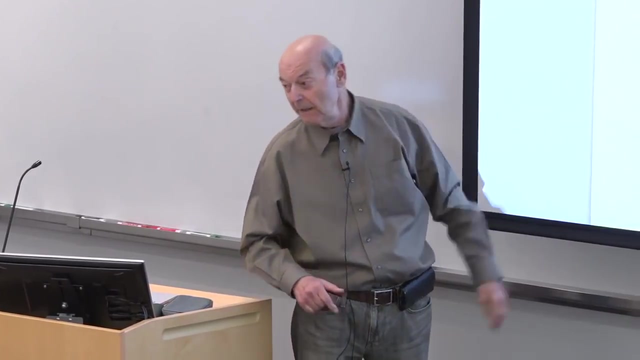 in abstract state machine community and he was interested in proving Church-Turing Thesis. and in order to prove Church-Turing Thesis we had to go back somehow to the initial state. in our case could be very rich. We rule no initial states out. 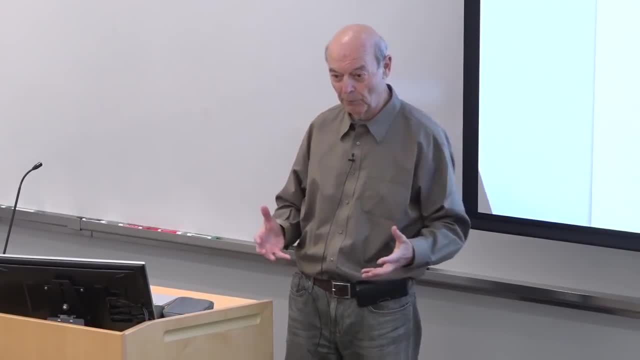 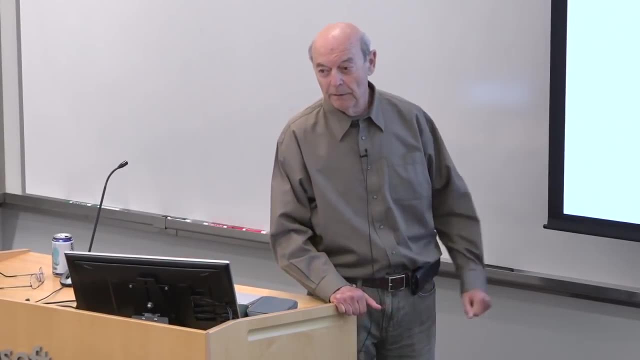 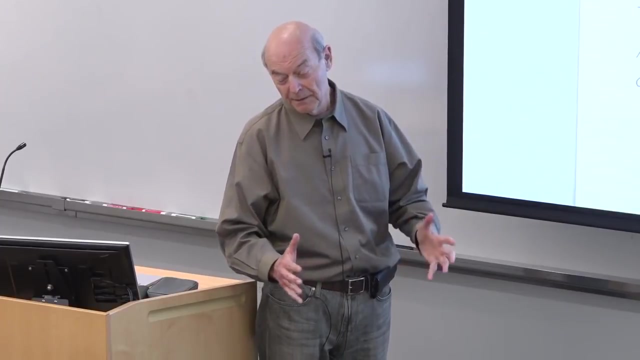 So, for example, initial states may have a solution to the halting problem or whatever. So, and then, of course, there is no chance for you to compute only during computable functions, So you need to somehow cut it down, and this cutting down is relatively easy. 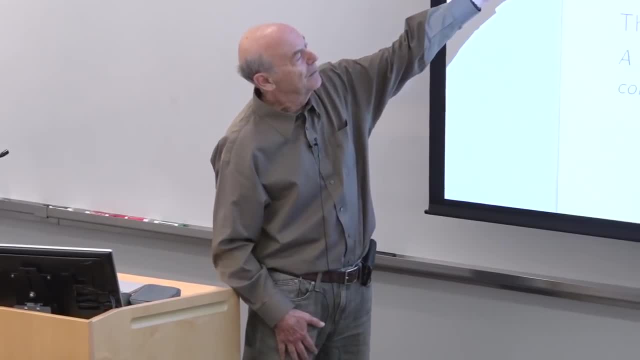 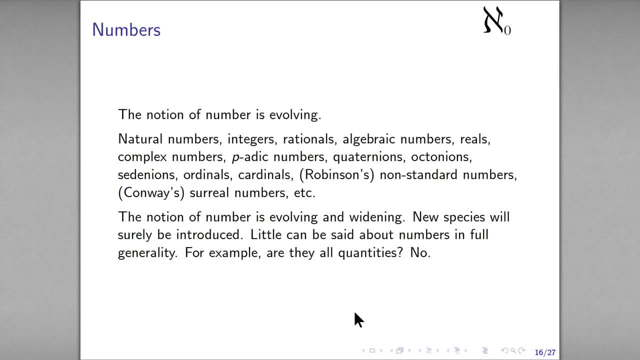 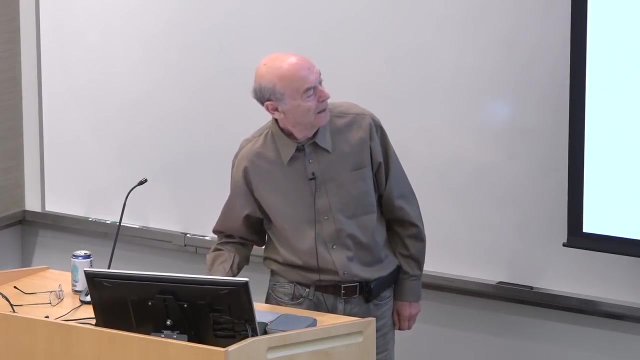 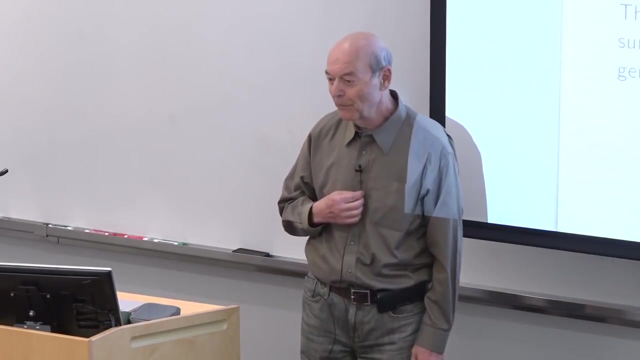 There are some technical details, but so we formulated the arithmetical axiom Similarly. we could instead formulate string kind of axioms. This is to improve, oops, sorry, Oop, improve that. Okay. Now let me for a moment speak about numbers. 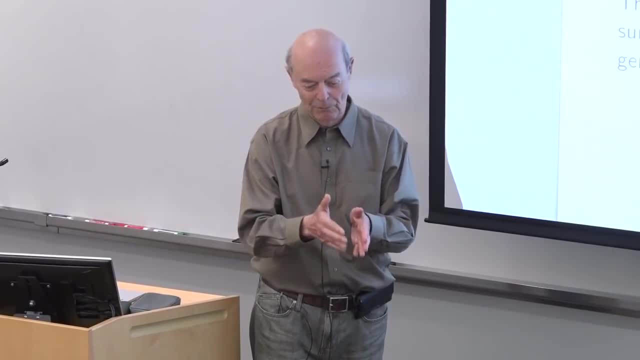 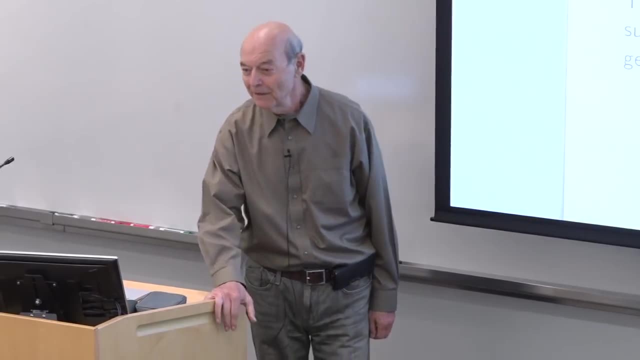 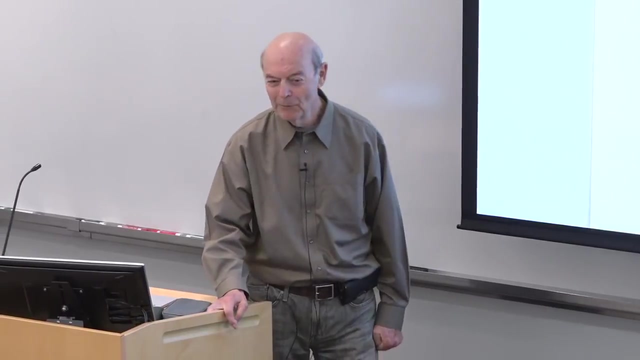 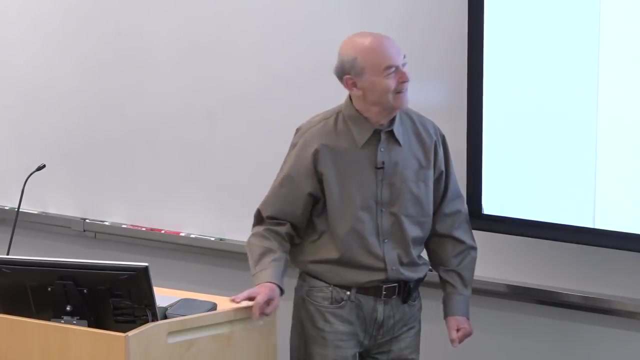 What are numbers? Originally they were just one, two, three. Then negative numbers appeared. Rationals zero actually came about very late. That's why we have one DC and one BC and there is no year zero. Okay, But by now 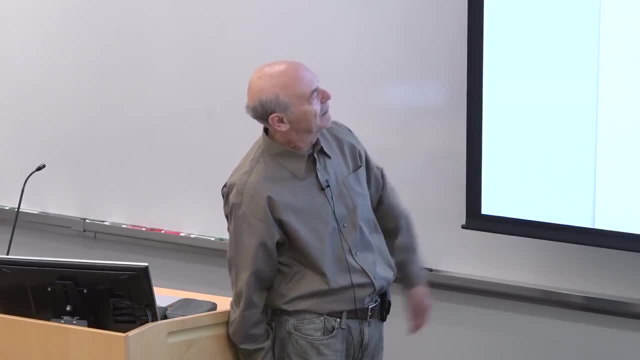 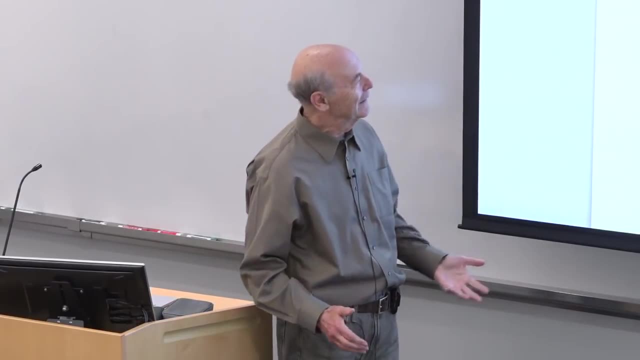 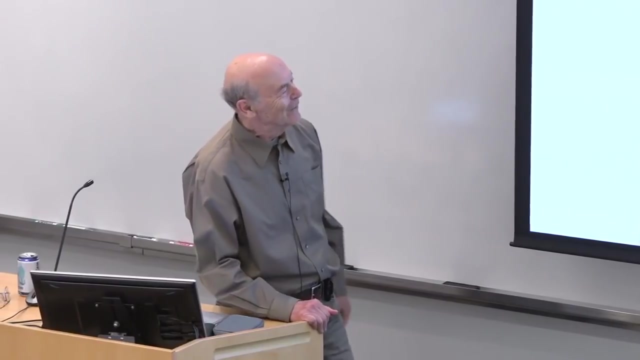 we have algebraic numbers and reals and complex numbers and periodic, So it's not about quantities anymore and we keep going. Okay, That's quite an interesting surreal numbers. So the notion of number is evolving and widening. 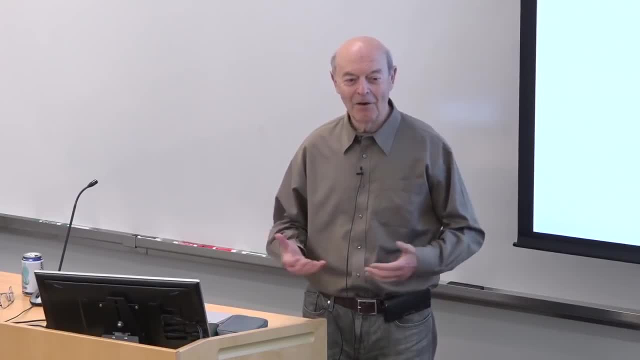 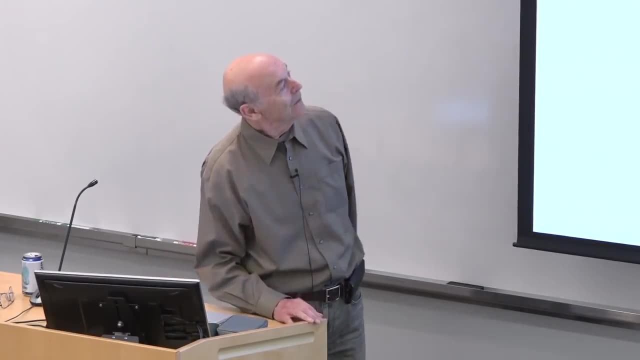 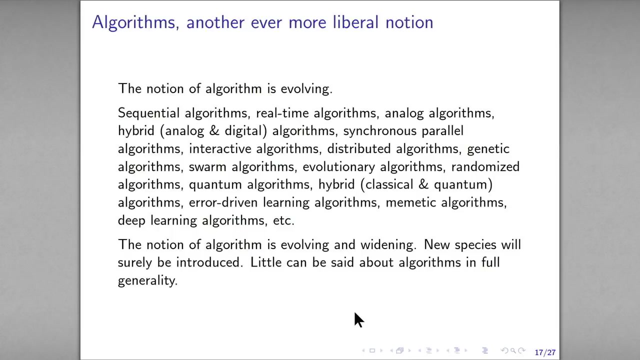 So there's not much you can say: All numbers are such and such. It's just analogy, because it's a familiar notion. So same happened to algorithms. So when Church and Turing wrote, the notion of algorithm was relatively robust. 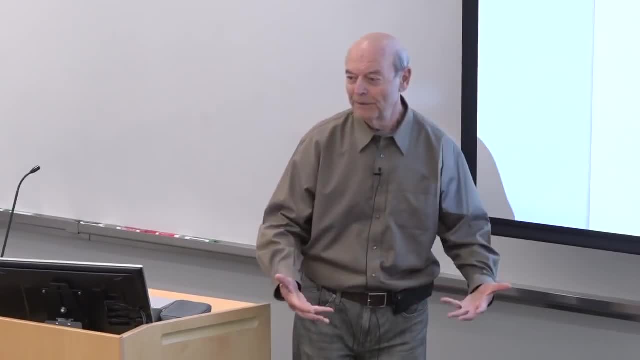 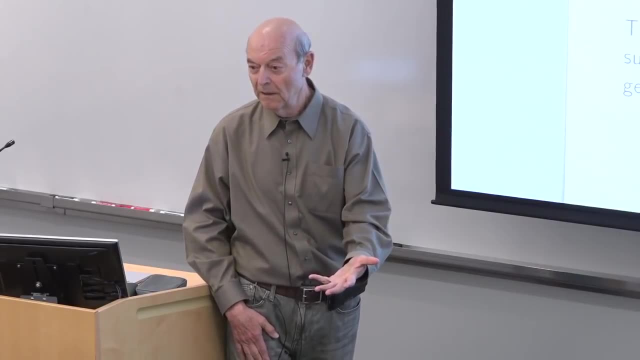 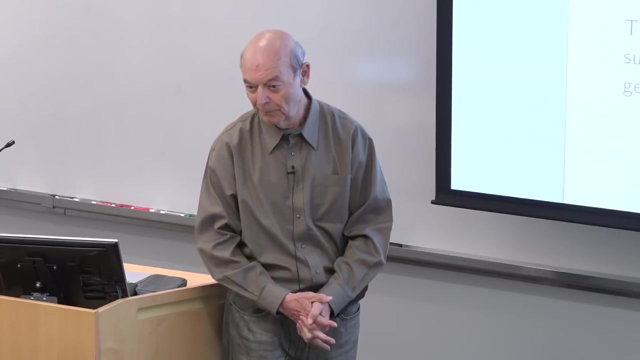 Everybody agreed, more or less, what are examples? So, in a way, when you see it, everybody knew what's an algorithm, what's not algorithm. I don't know any single example that people will argue: oh no, this is not algorithm. 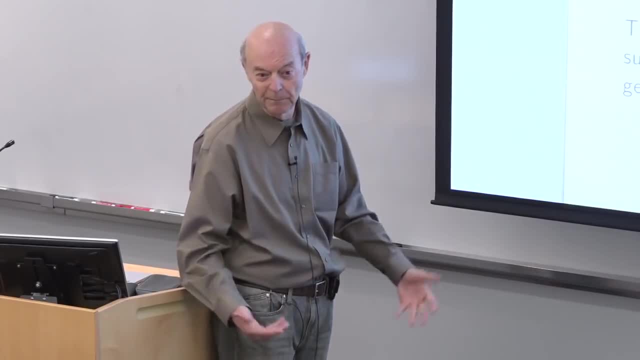 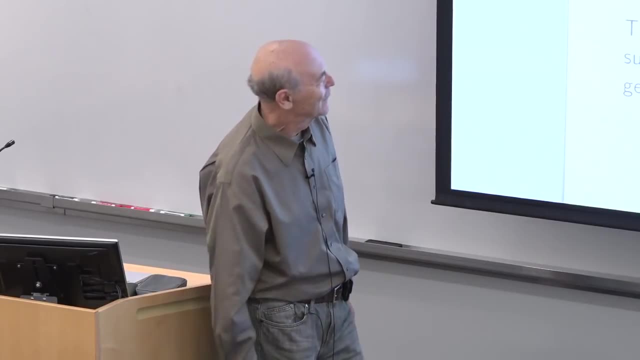 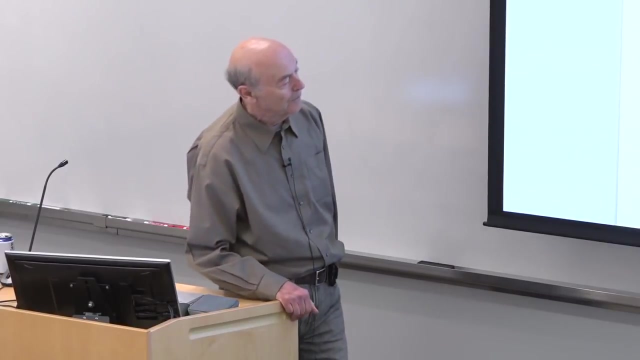 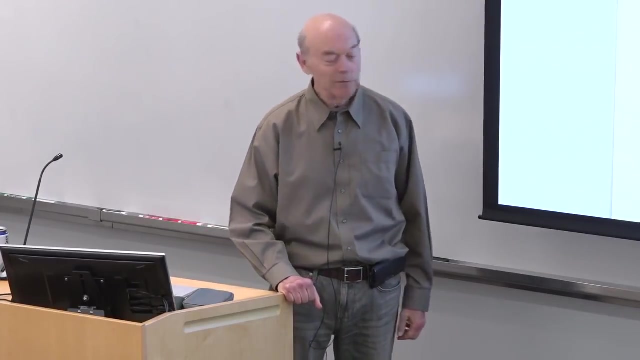 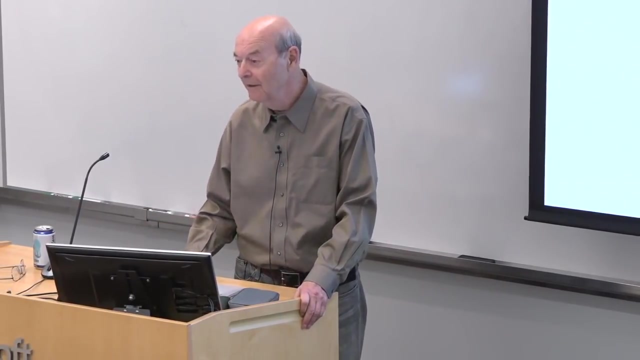 So it was quite a robust notion, not formalized, but robust. Now, where does it end? So the notion of algorithm is evolving and widening and getting ever more liberal. Surely new species will be introduced. So not much can be said about algorithms in full generality. 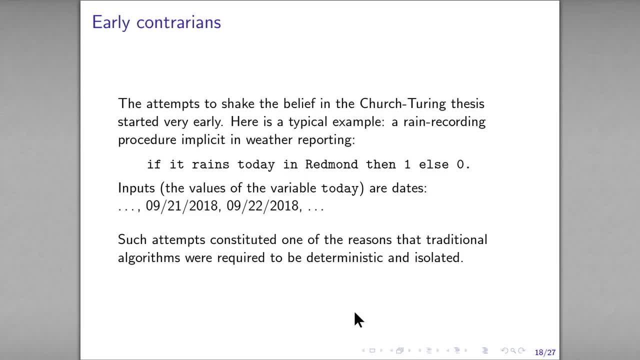 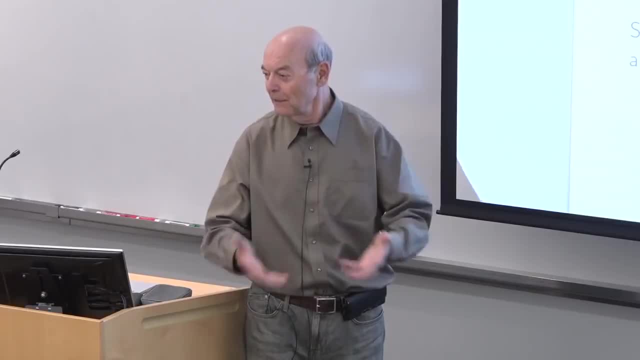 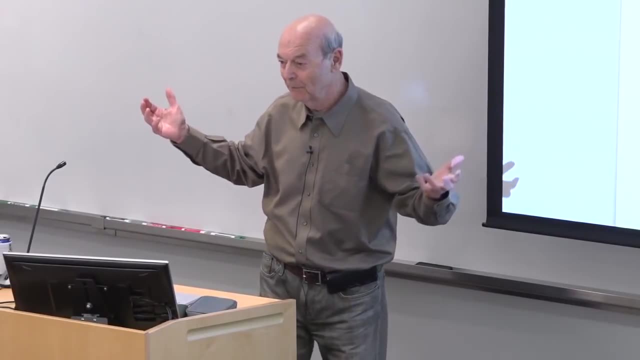 So that was my original argument. Why this not Turing thesis, but this over-generalized version of it: all algorithms? why should it be true? Because it would say something about all algorithms which is very unlikely, seems to me. 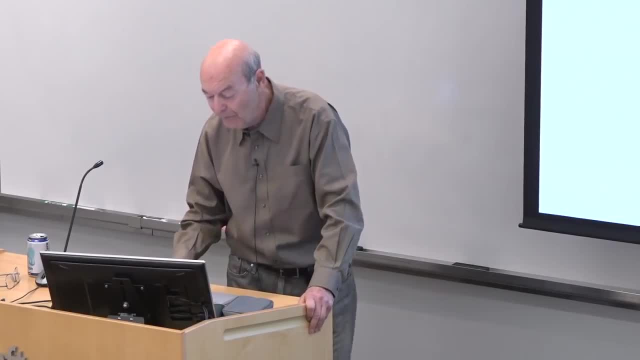 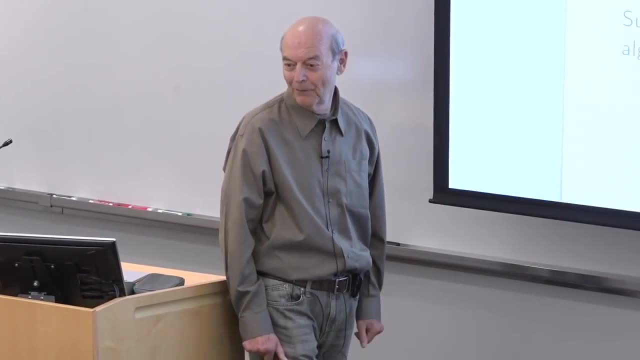 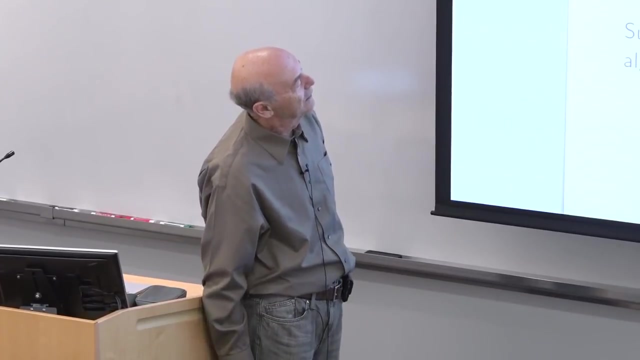 So there was some contrarians very early. I asked Andreas, whose example Andreas Blas, many people here know He thought it's from Kalmar but I couldn't check, So it's one of the very early examples of algorithms. 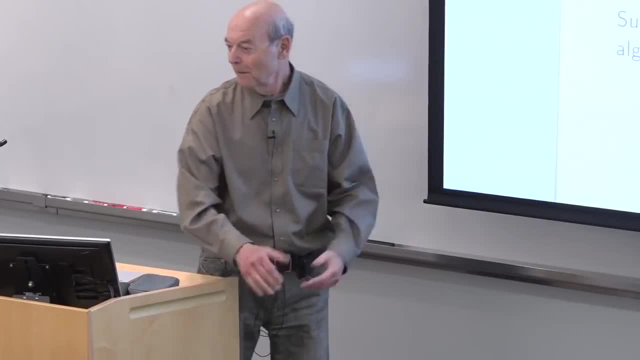 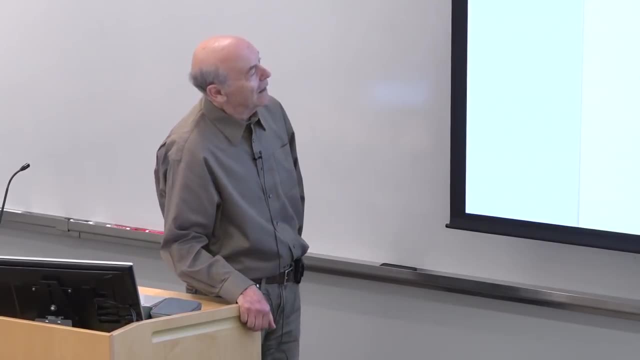 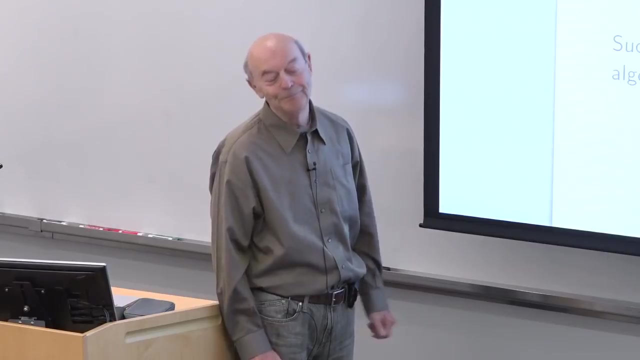 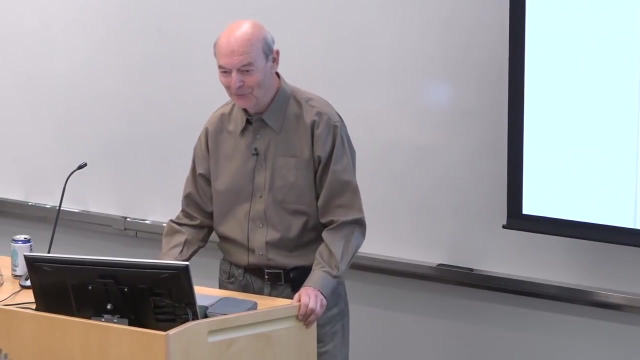 algorithm looks algorithmic and obviously doesn't compute Turing computable recursive function, But- Depending on whether the universe is Turing computable right? Yes, Right, We don't really know. Yeah, It could be all finite and therefore it's all. 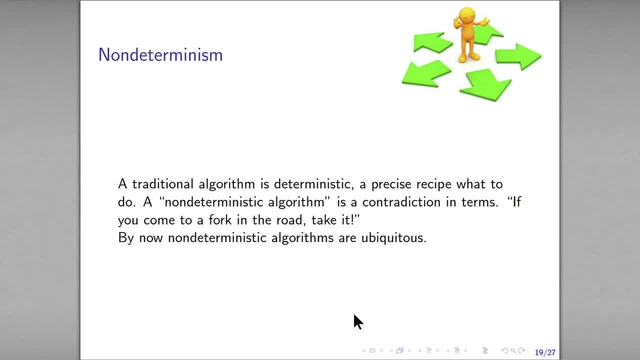 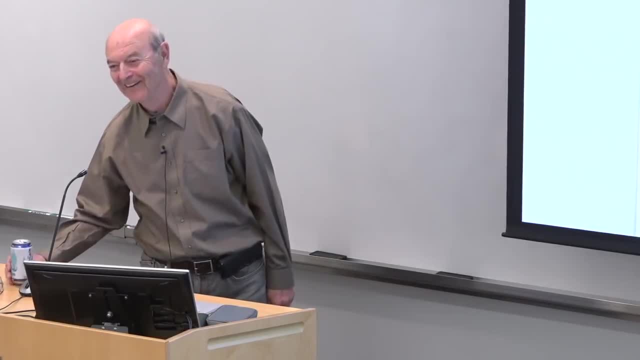 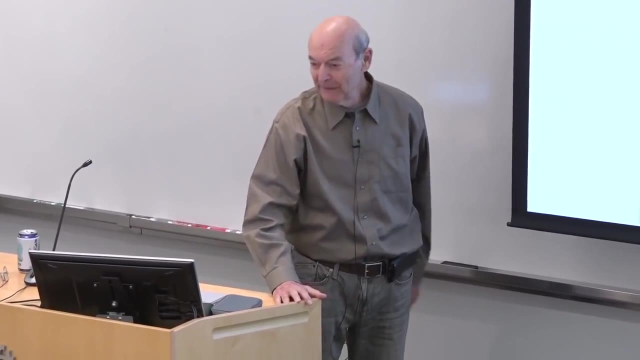 Wait a second, So touchy. So now to non-. I didn't know that Redmond played such a big role in this debate. It wasn't Redmond in the original example, Might have been Brooklyn. So non-determinism. 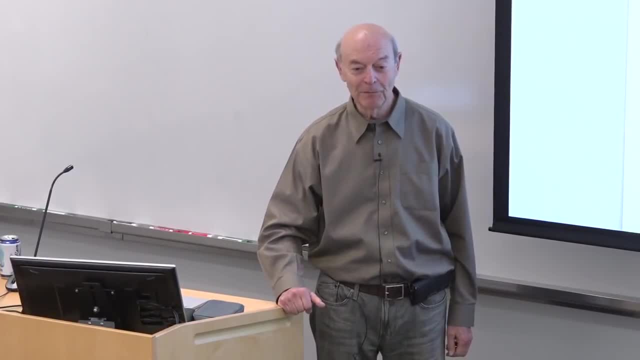 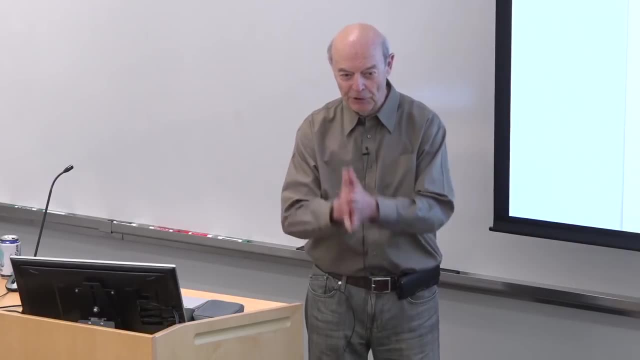 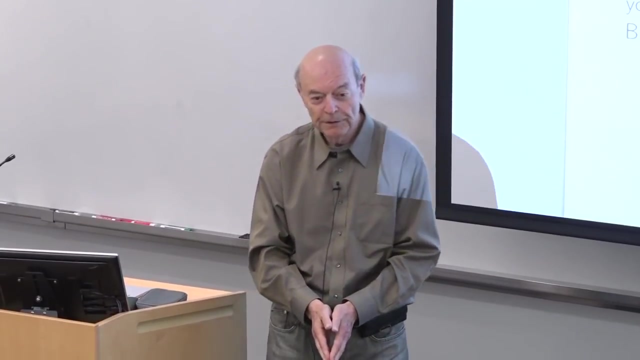 From traditional point of view, non-determinism is non-deterministic. algorithm is a contradiction in terms, Because what's a non-determinism? It's an algorithm. Algorithm is a recipe which you execute exactly Now. if you come to the fork in the road, take it. 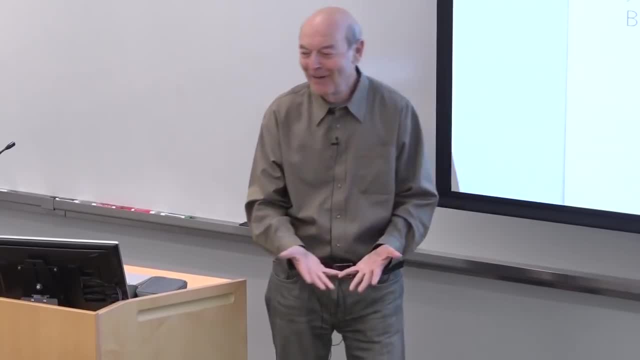 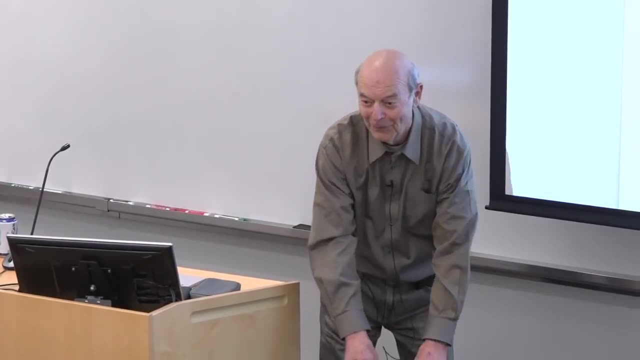 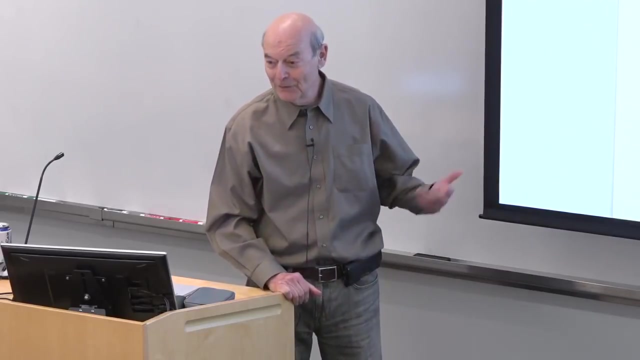 What? Take what? You know what kind of algorithm it is. It's a joke, Okay, I don't mean the physical fork on the bottom, you know forking road. So now, today, of course, they are ubiquitous. 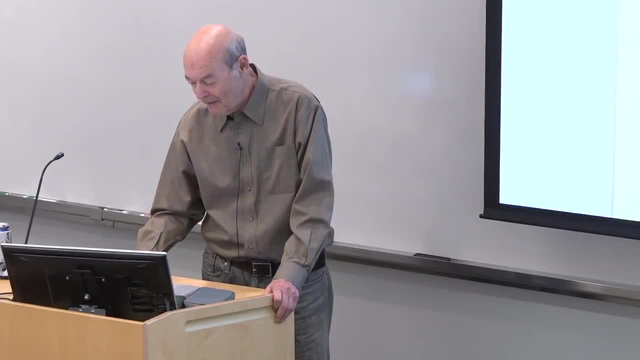 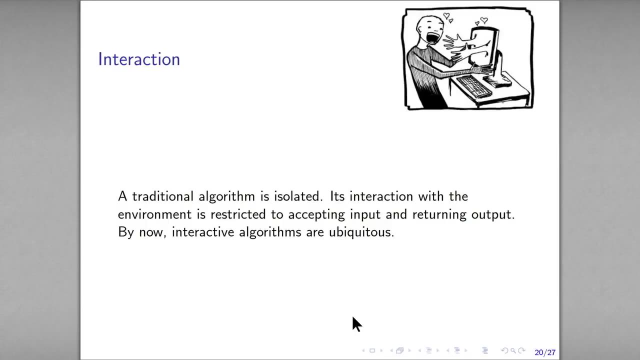 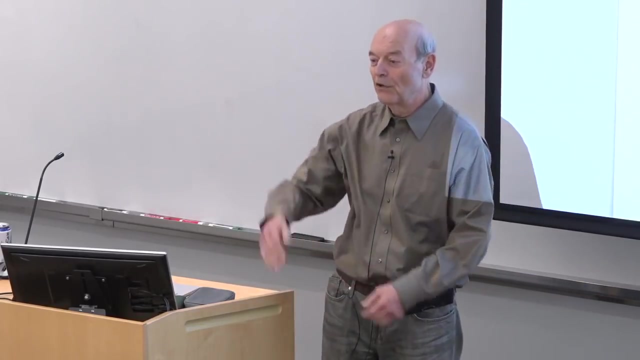 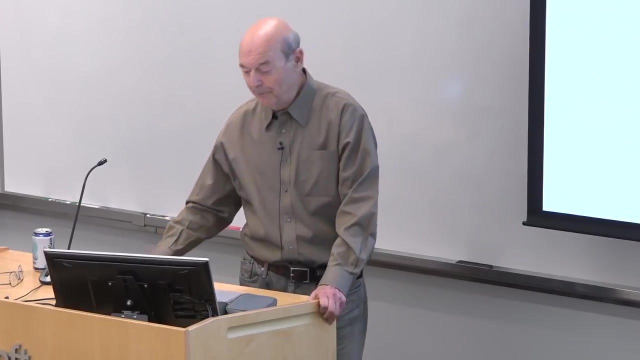 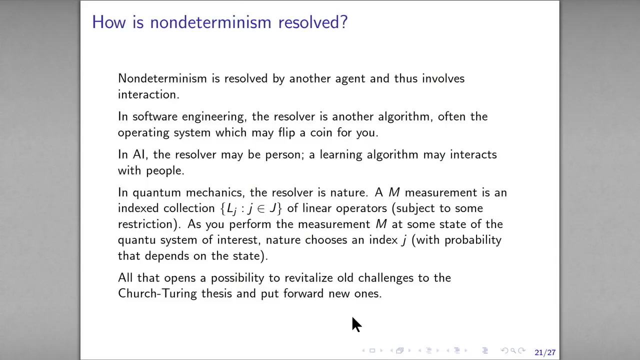 Also, oops, interactive algorithms. So algorithm was supposed to be isolated. That's why you couldn't, you know, measure rain. It contradicts isolation, But by now interactive algorithms are very, very common. Oops, Excuse me. 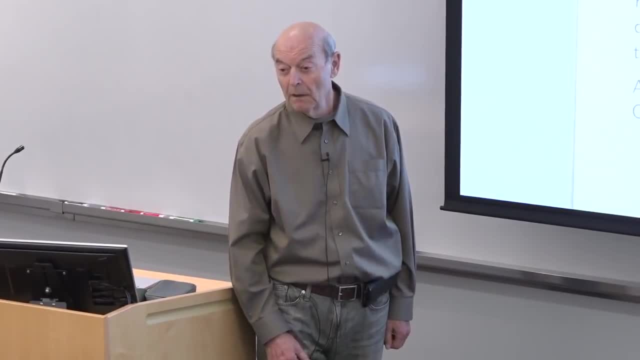 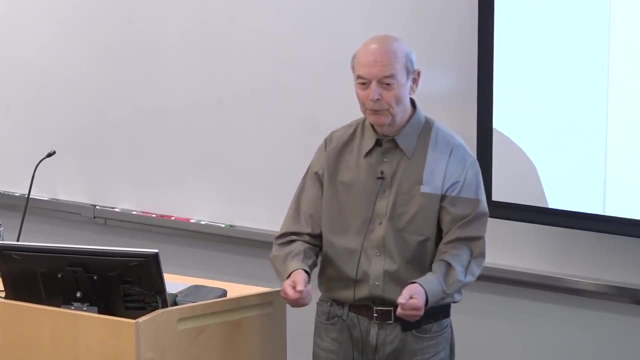 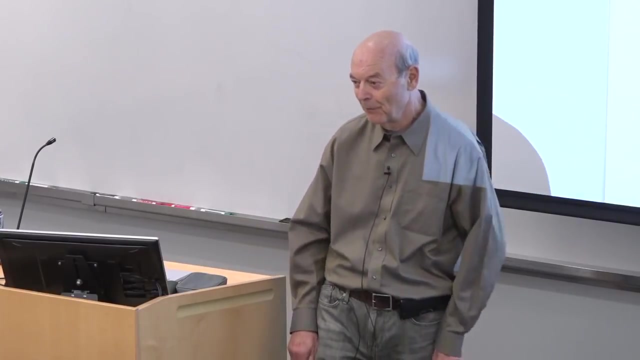 So how is non-determinism resolved? It's by interaction. Now imagine you have an algorithm. come to the fork in the road, take it. So some operating system will flip a coin for you or does something. So it's interaction. 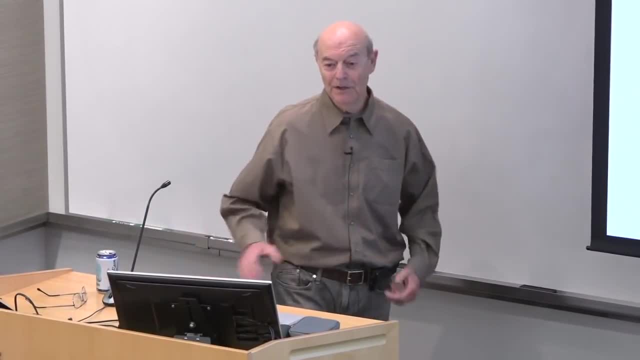 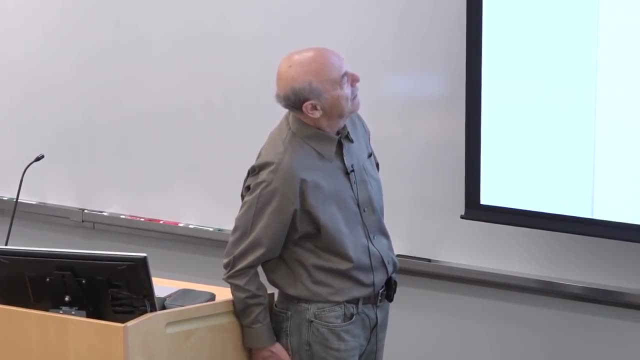 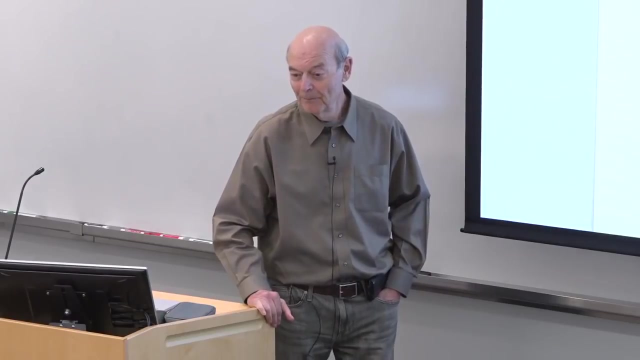 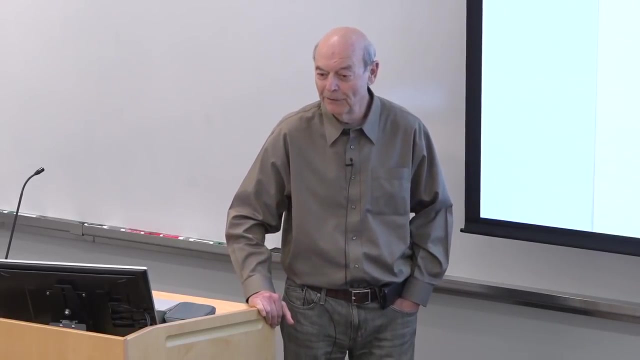 In this example the operating system, but in general there are interacting algorithms In AI, there are learning algorithms. They often learn from people, So they interact with people And they're definitely algorithm learning algorithms. Now we can argue, say learning algorithm is not an algorithm. 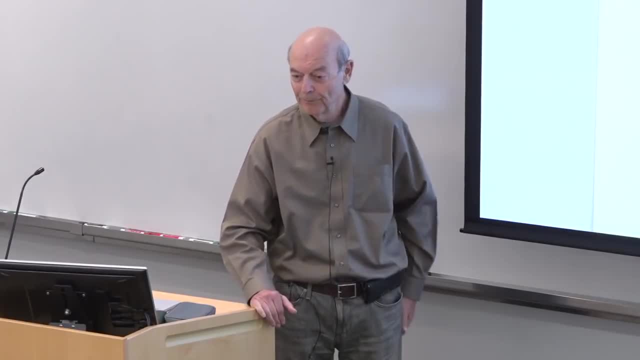 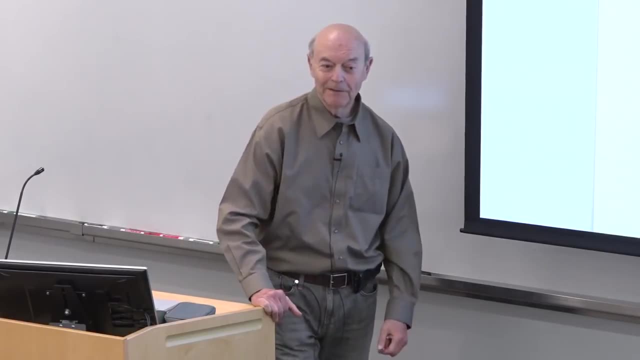 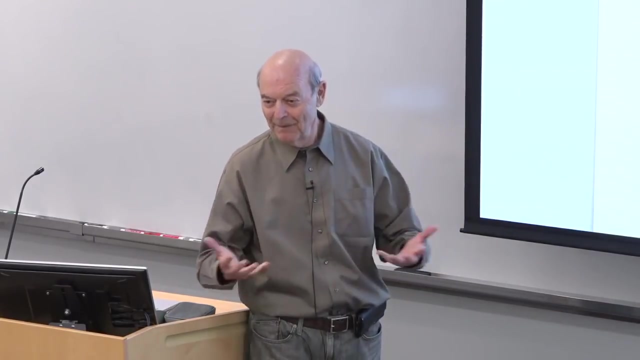 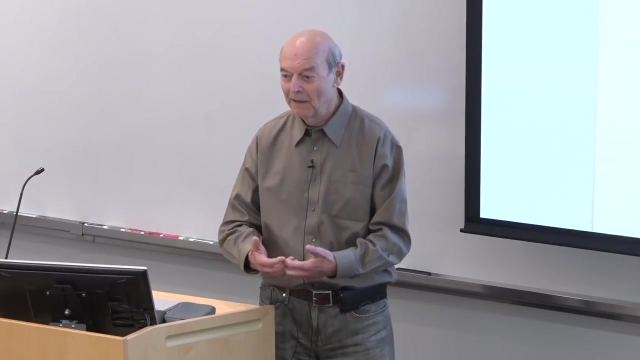 You know, it doesn't, it may change its own program. So in quantum mechanics quantum mechanics actually is very different Before quantum mechanics. all this example, all in computer science non-determinism always is resolved by interaction with another agent. 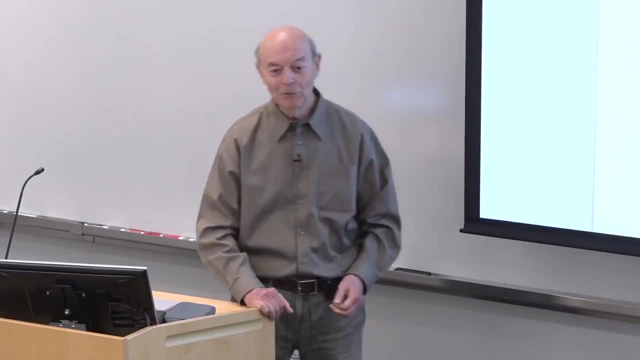 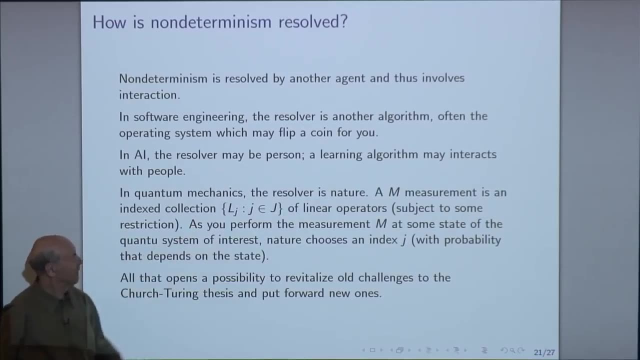 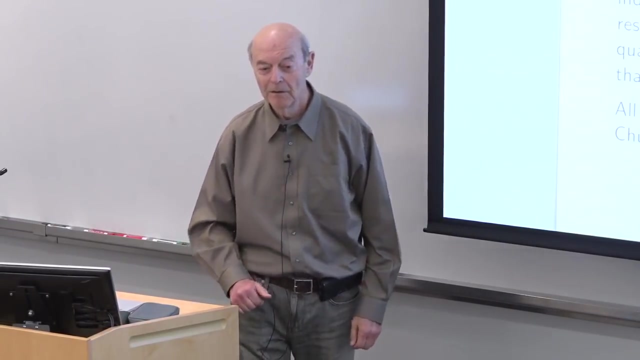 obvious agent, computer person. In quantum mechanics you interact with God, with nature. So when you measure, a measurement is collection of linear operators, And when you measure by field, one of the indices is chose. So here we have a couple of experts on quantum mechanics. 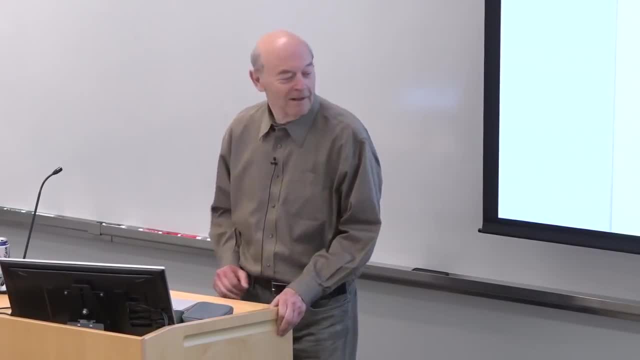 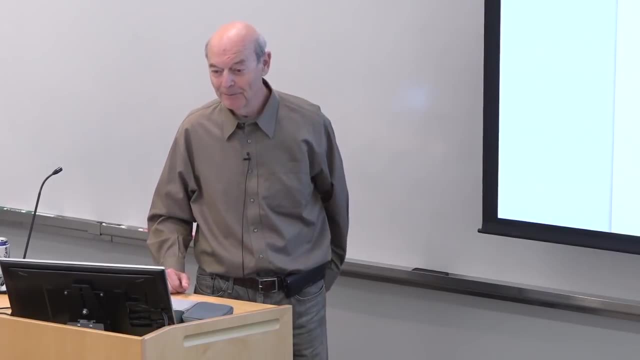 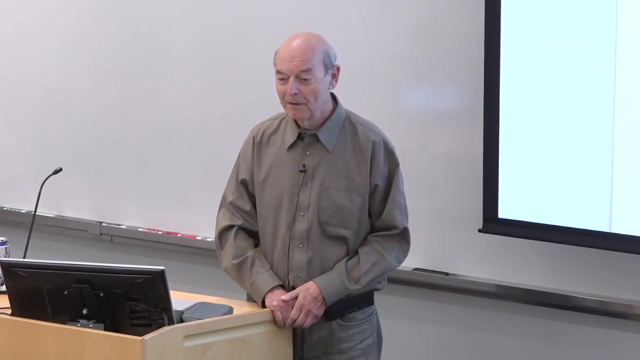 which hopefully will keep me honest: Nobody knows. it's a lot. it's kind of mysterious how it happens, but that's how it happens. So you interact with nature? Ah, but if you interact with nature and with people, that opens. 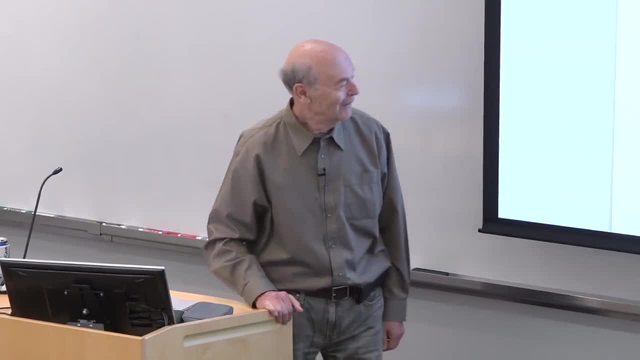 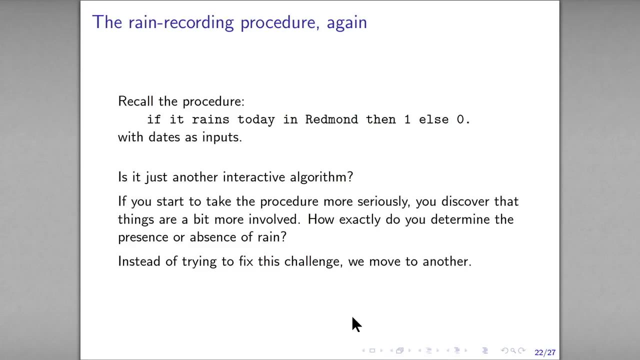 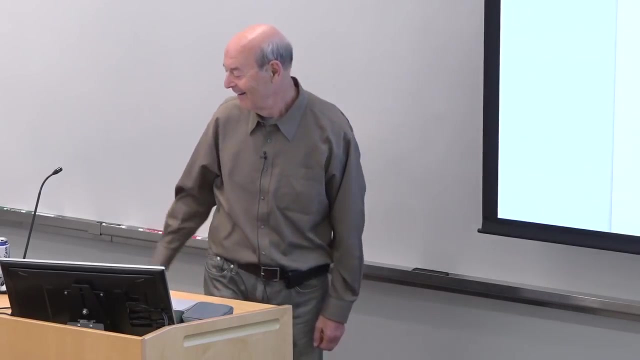 opens up a lot of possibilities. okay, For example, that same example. What's wrong with it? It's interactive algorithms. Well, it interacts with nature. It's not a matter of definition, though, because you might say that something is non-deterministic. 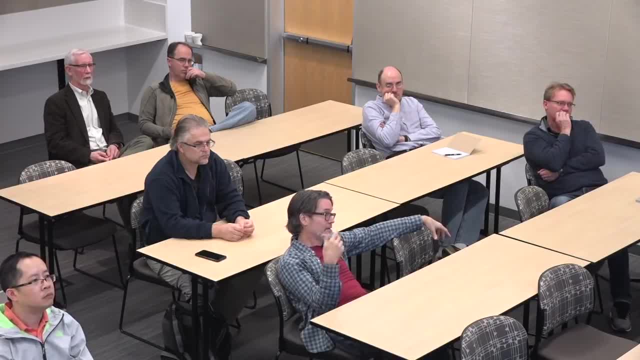 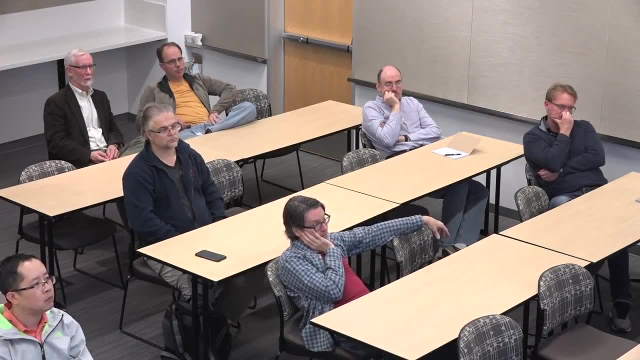 Well, it's really a game, you know, and it's playing against an adversary, Or, you know, you can imagine lots of processes that are not algorithms- A game. A game is much more complicated because- Well, I mean when you have non-determinism in a system. 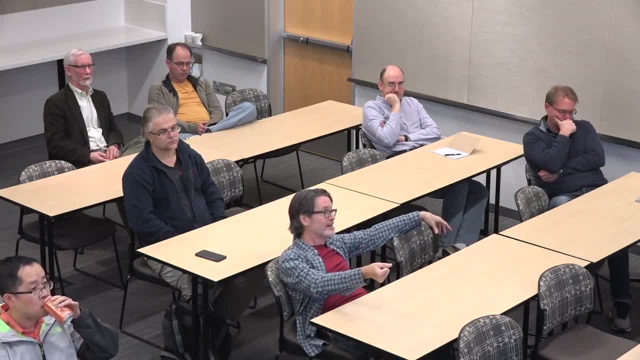 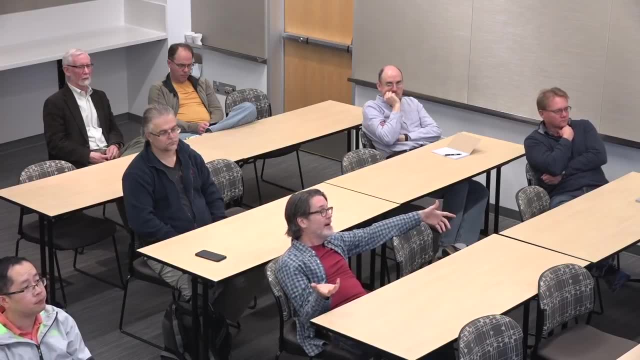 you have to ask, as you say, the question of who is providing that? Yes, Right, And so is it an adversary, Is it cooperative, And so on. So all I'm saying is you could define that to be an algorithm, right. 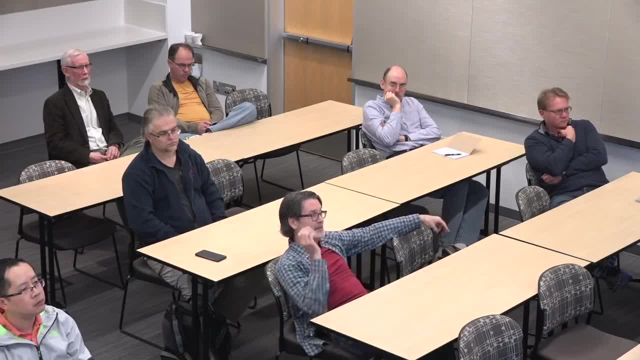 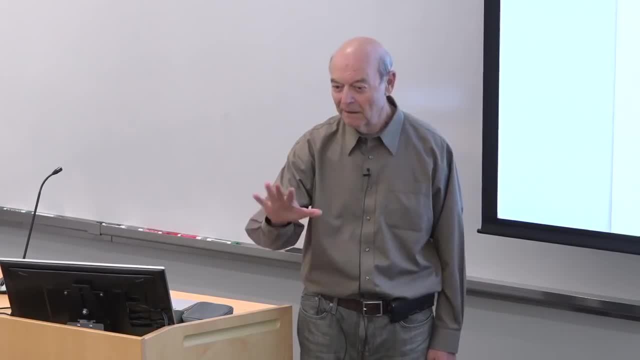 Something that interacts right. Or you could say, no, that's something else. I mean, it's not, it's not clear. I mean, why would I- Wait, wait, wait, wait. So the point you're making, 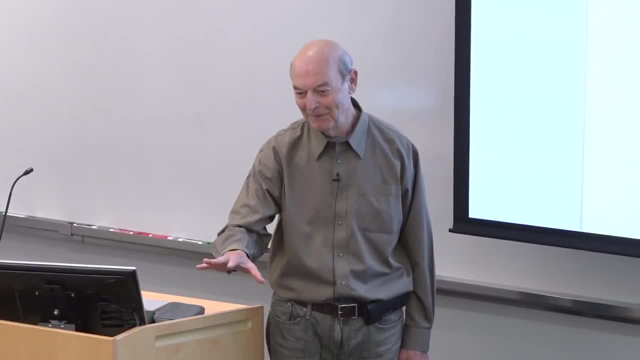 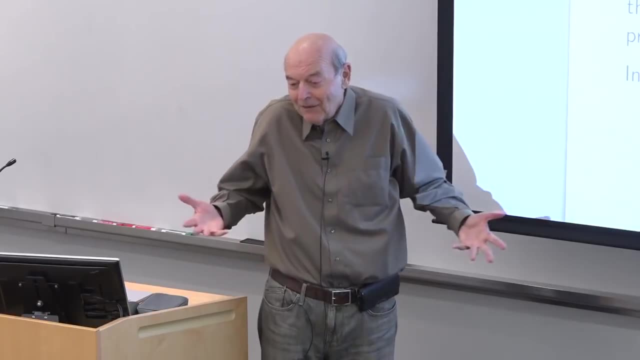 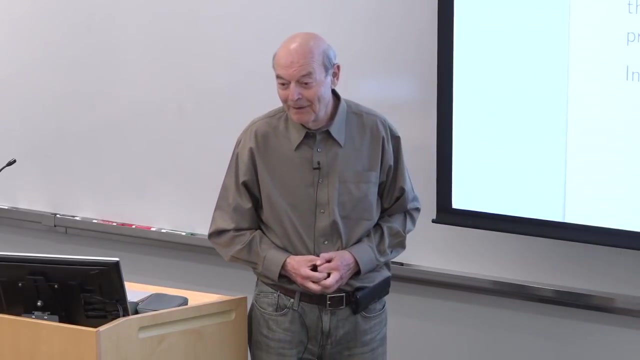 actually is a point. what I want to make, That's a matter of agreement. Do we consider this algorithm or not? Probably not yet. But it interacts with nature. It's the way you know. measurement interacts with nature. Act of measurement is some kind of interaction. 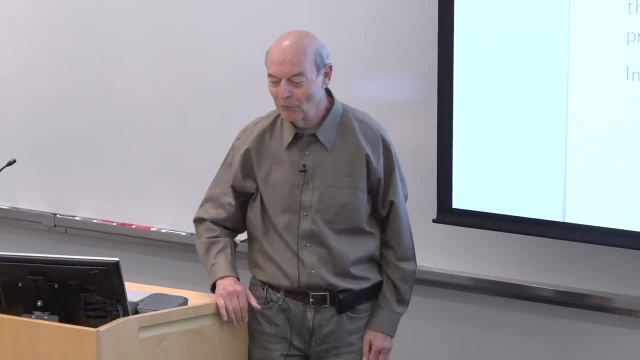 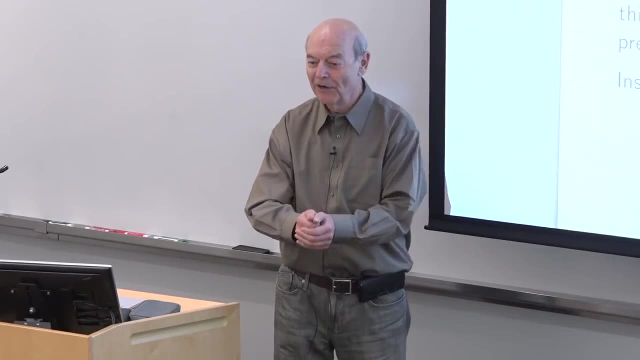 Now there it's kind of mysterious and something happens as you measure. Here it's very openly. Now you have to fix details. What does it mean? a rain? So one can argue that's not quite an algorithm, because is it raining or not raining? 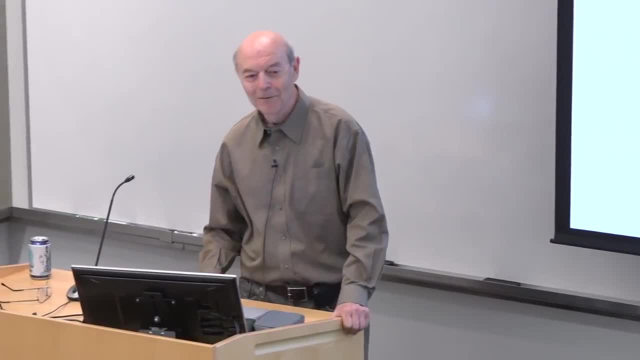 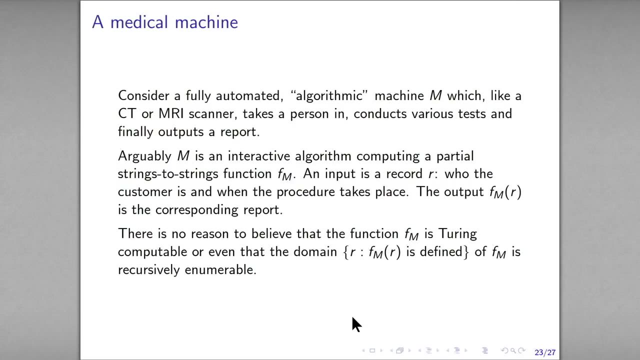 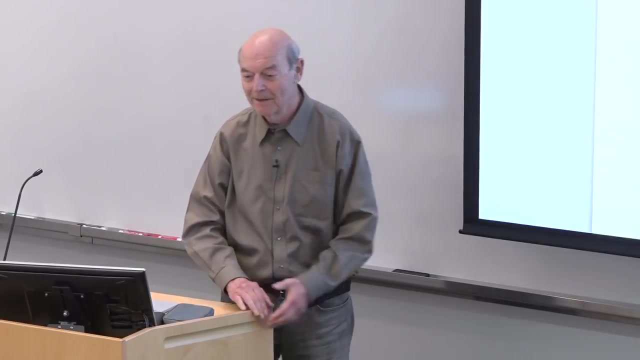 There are some. one can try to fix details Instead. I'm going to something else. So let's consider this medical machine. Like CT scanner or MRI scanner, it sucks you in and makes all kind of measurements, tests. So in the process, 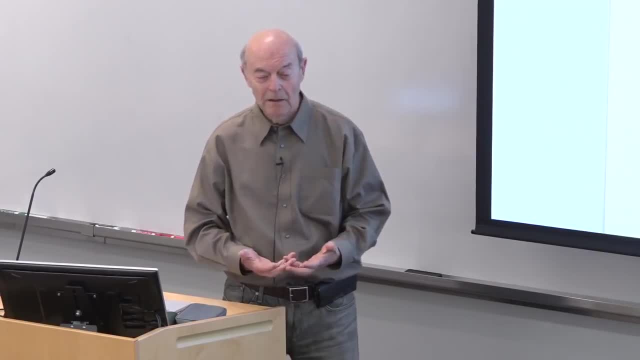 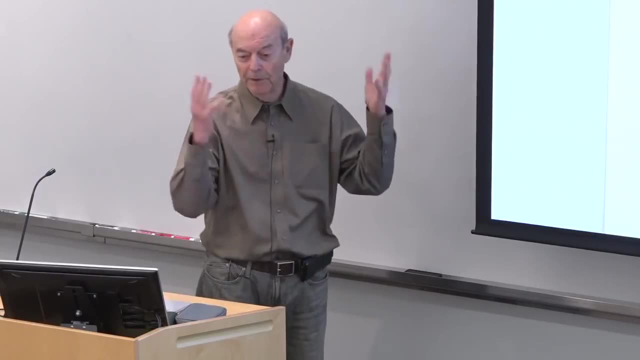 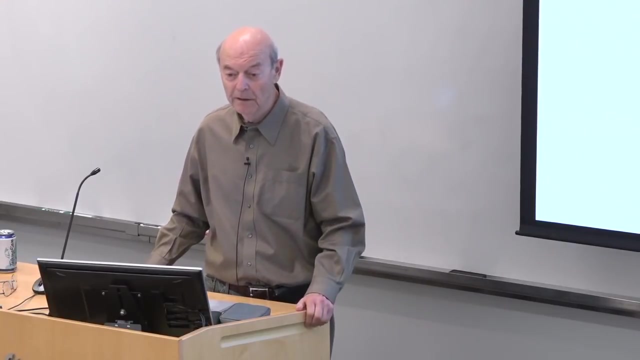 it computes a function. The input is your ID, who are you, and the time it was done. Now the output is whatever report machine produces. The machine is completely automated, algorithmic, So in that sense I'm not making any claims. 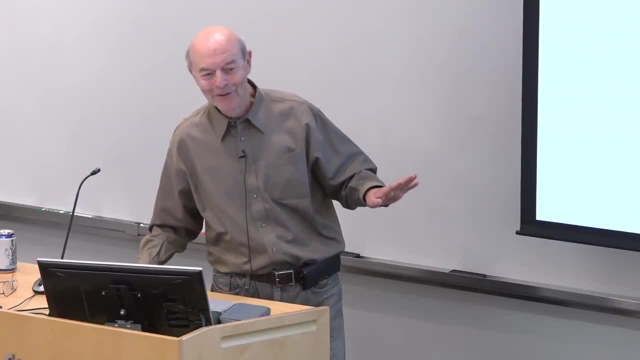 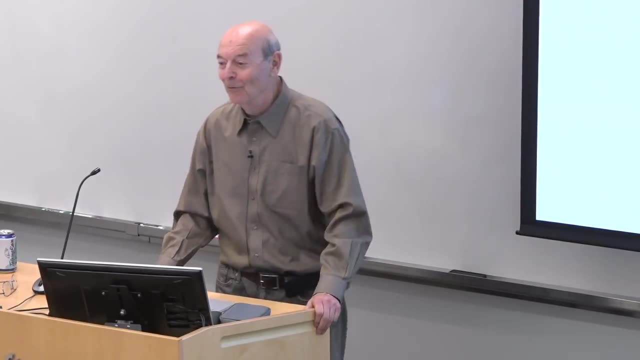 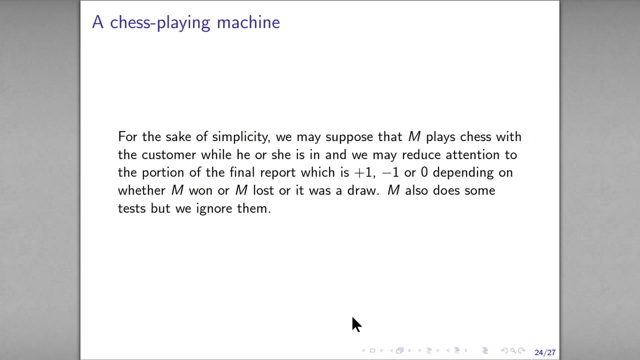 I'm not trying to convince you. this is an algorithm. All I want to make to shake your belief that we know exactly what the algorithm is. So do we want to consider this an algorithm? So let me simplify a little so that it produces just zero. 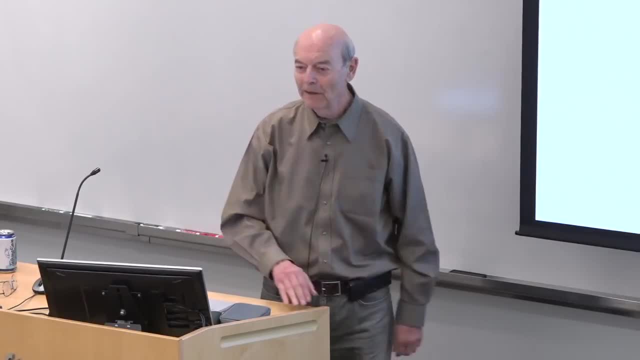 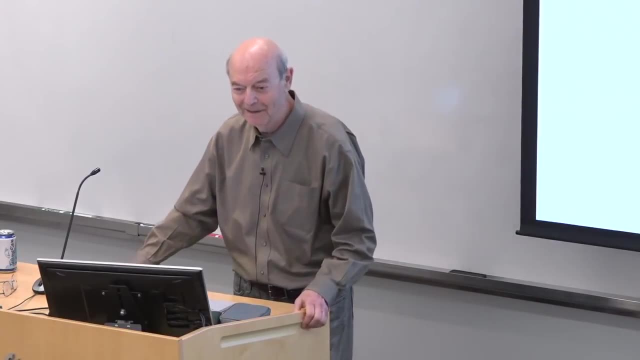 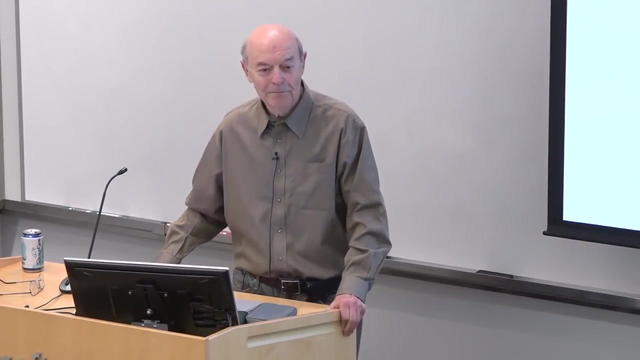 one or minus one, So it still can make all kind of tests. but it plays chess. Suppose you always white and the machine is black. it plays and then it produces plus one, minus one or zero, depending on whether the machine won. 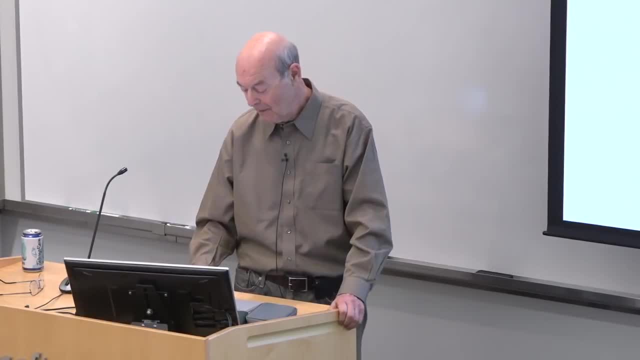 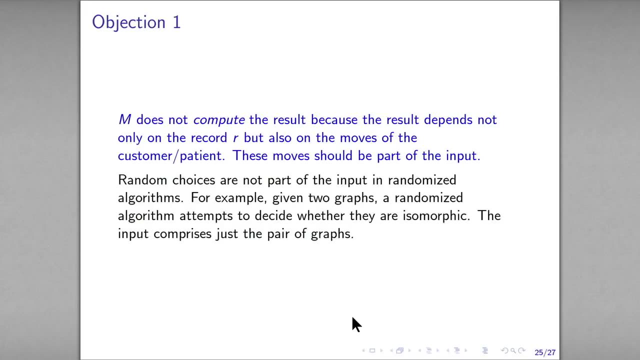 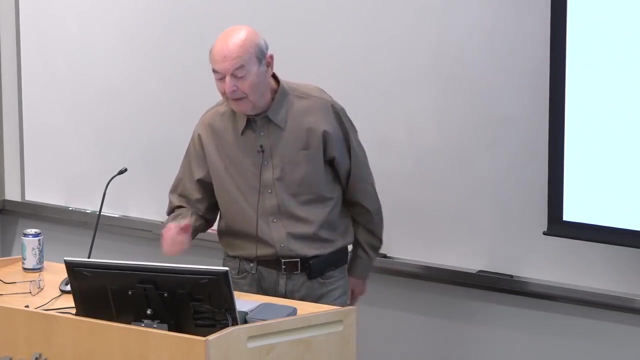 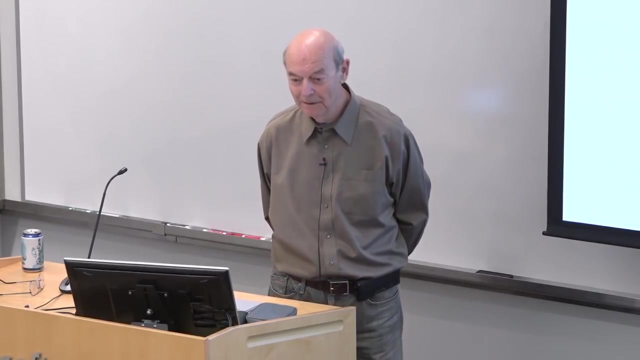 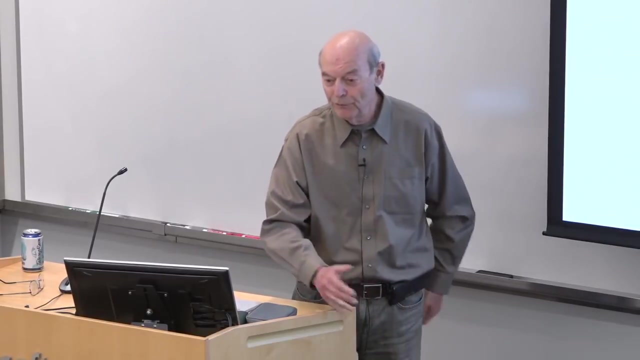 lost or it was a draw. So here's one objection. Yes, So it doesn't compute, because the result depends not only on your ID and time, but depends on whatever you say in the chess game. depends on your moves. 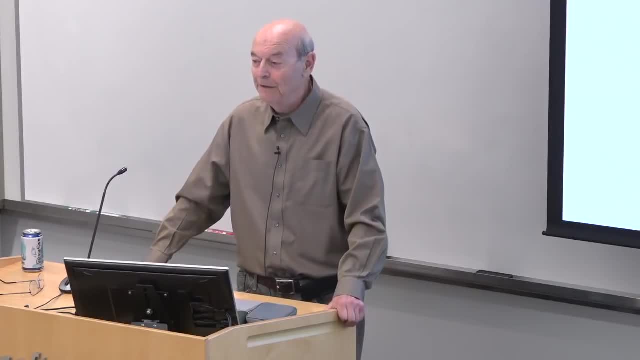 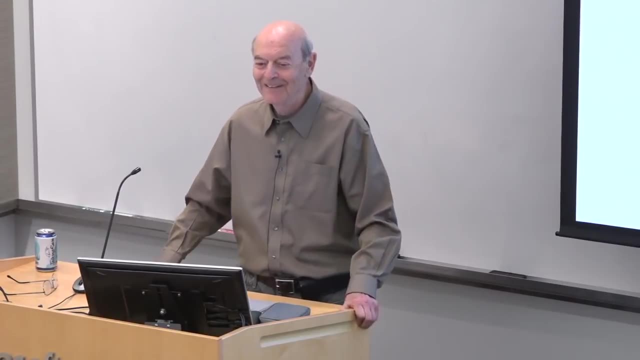 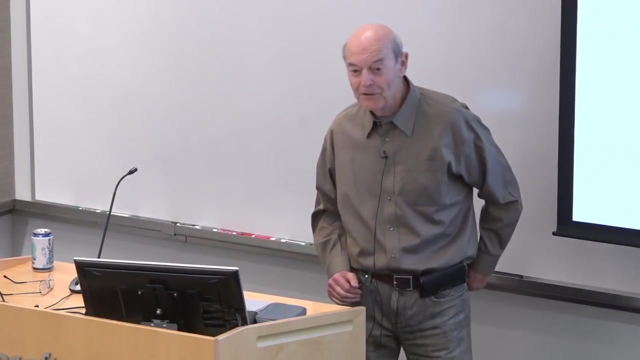 Maybe, but your ID and time completely determines the game Historically. that's the game, So it determines it Also. we know we don't, we don't often require that all this additional data should be count as input. 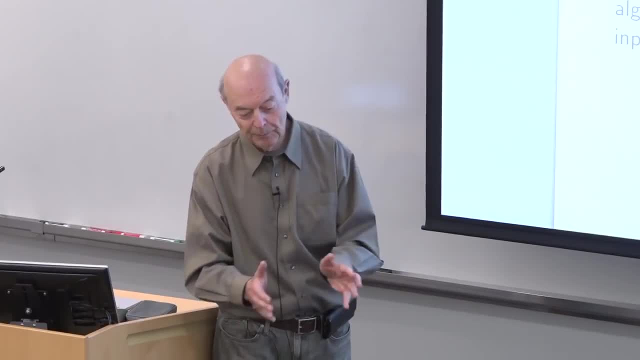 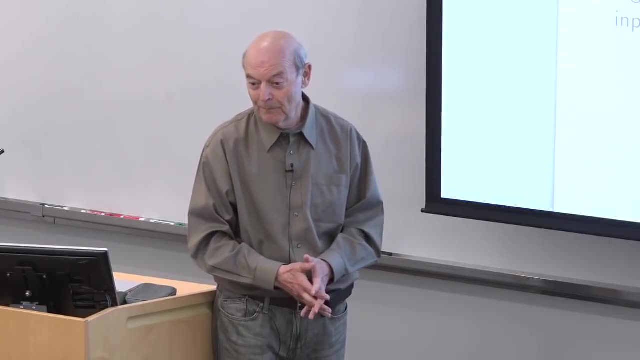 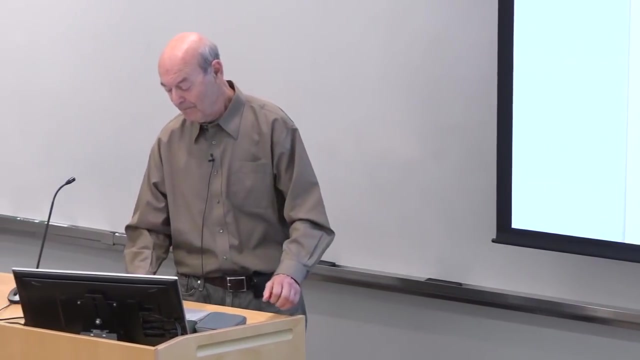 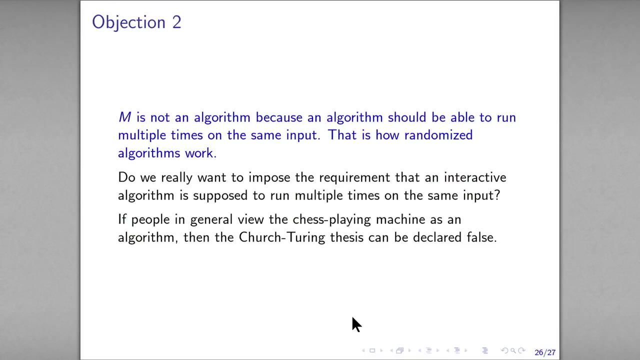 When you consider, say we have randomized algorithm giving two graphs, you want to determine whether they are isomorphic or not, Okay, You flip coins, but the input is just pair of graphs. So it's not an algorithm. because with algorithm, my component says: 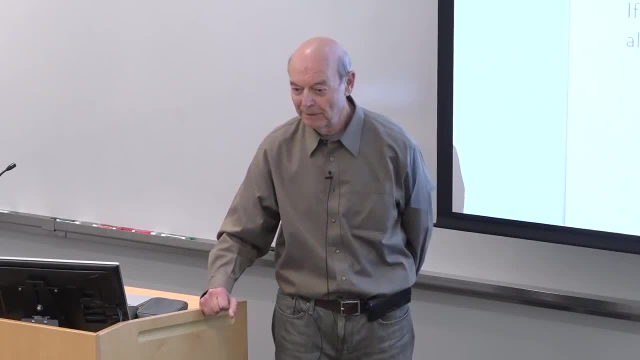 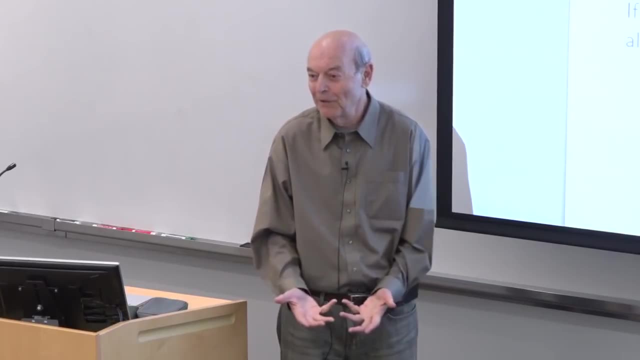 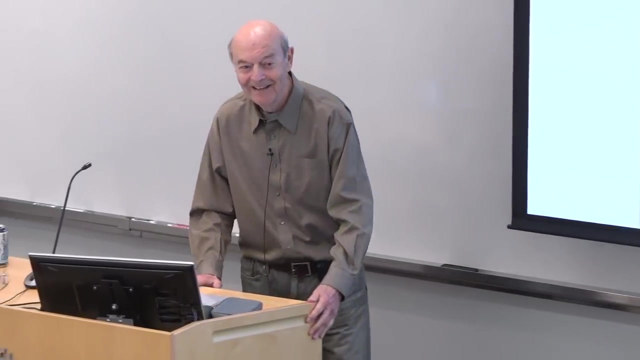 you should take the same algorithm, run again on the same data, Maybe, but this is legislation, This is stipulation. You say every algorithm has this property. We never agreed on this. Why should be the case? So the whole idea of sucking you into the machine was: 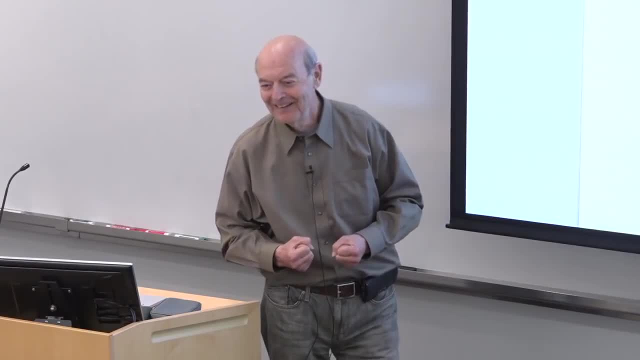 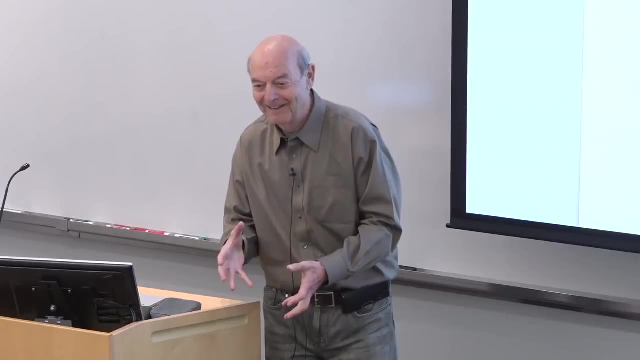 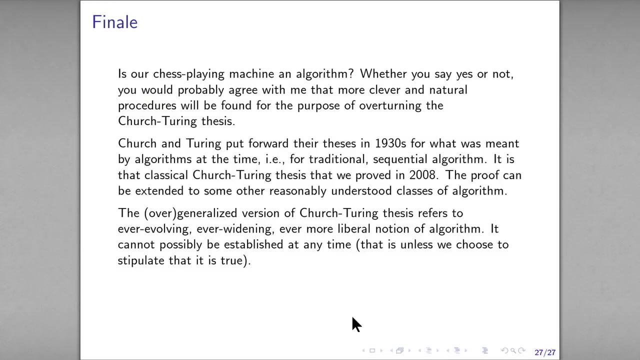 so you cannot play two games. So I specifically tried to construct scenario which you cannot repeat, definitely violating this requirement. Okay, So I'm coming to the end. Is a chess playing machine an algorithm or not? I think out of this context, 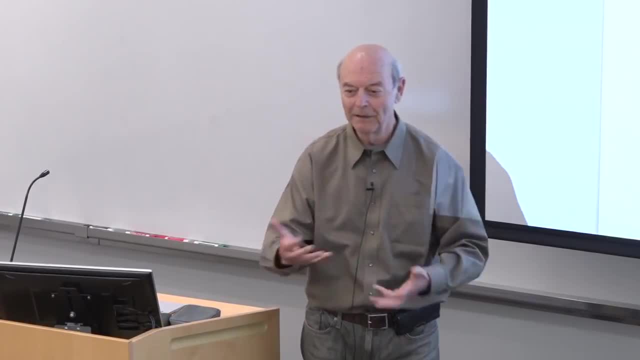 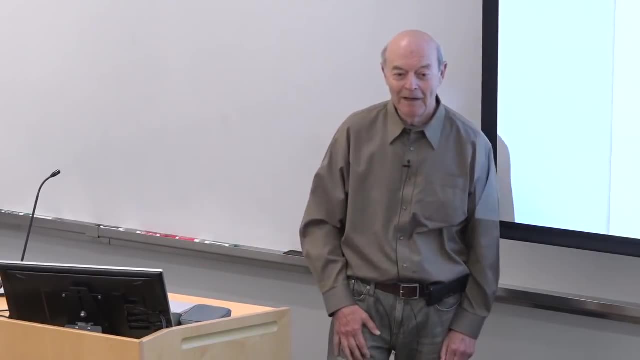 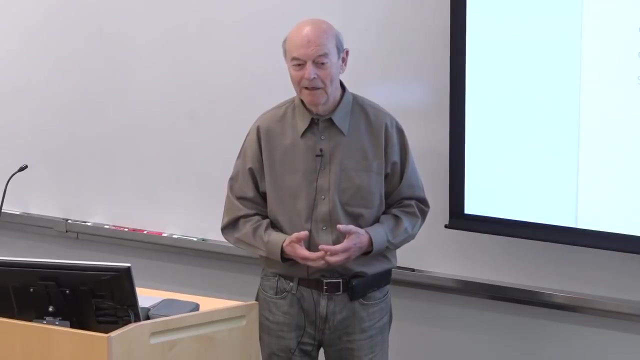 when we discuss this. if you talk to somebody who says: here is an algorithmic machine, some people may accept it as an algorithm, Some not. But my point is: whether you accept whether it's algorithm or not, you probably accept that they will. 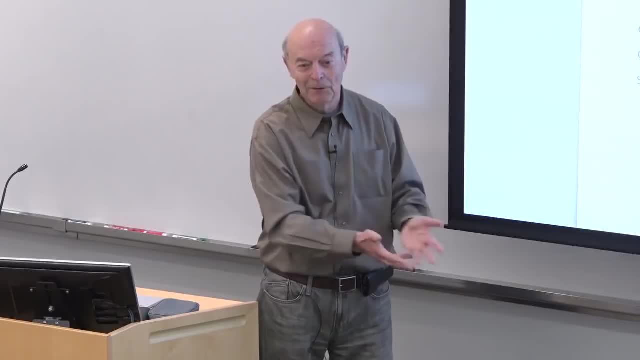 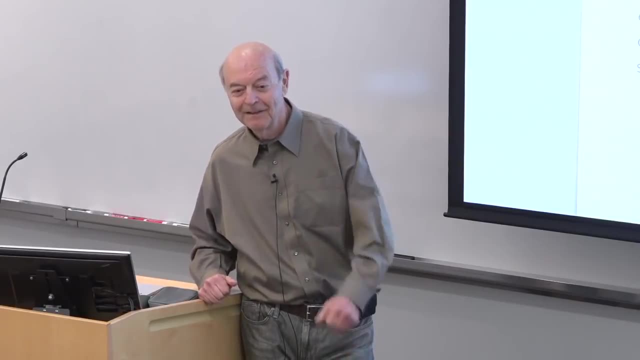 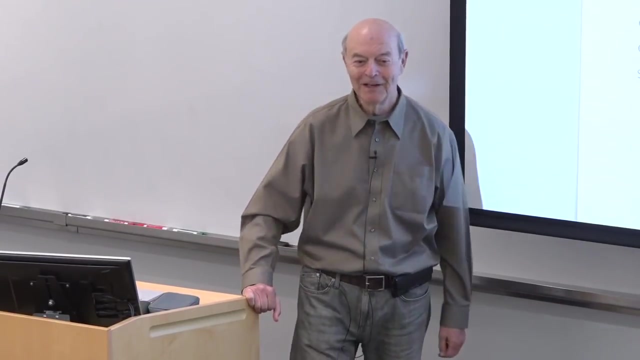 I just constructed this in last few days because I was preparing this talk. Some more clever algorithms will appear. Yes, Here's a guy who is. you studied deep learning right, So you have more interesting examples, which I have no idea what they are. 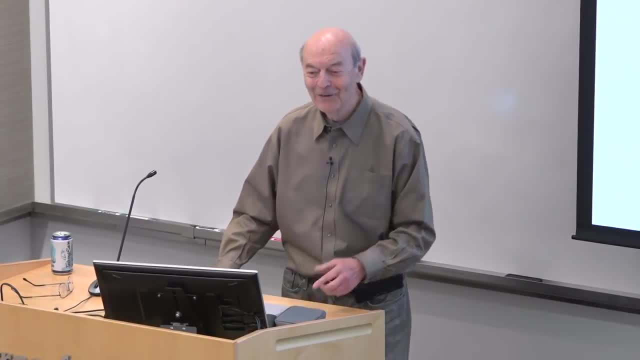 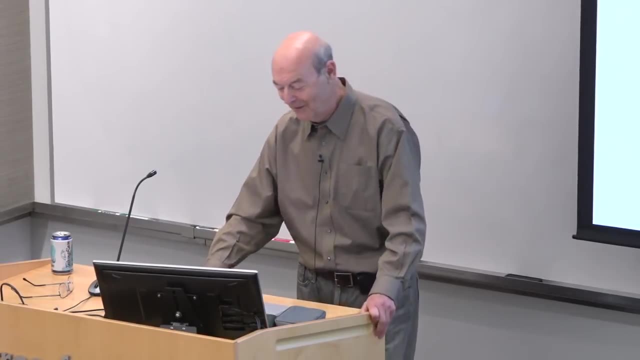 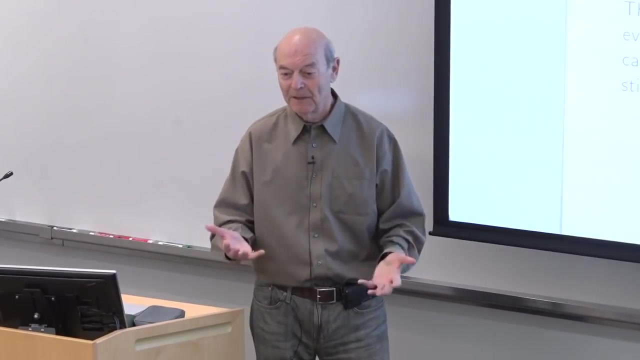 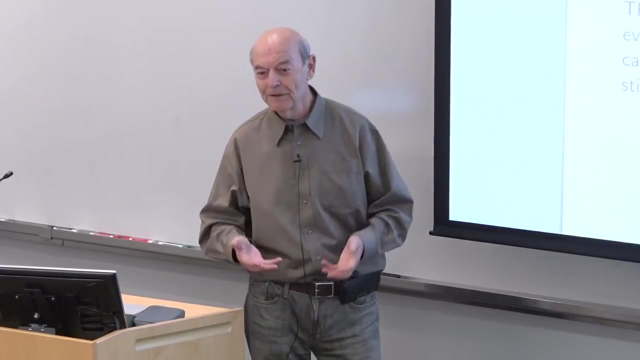 Yes, Okay, So maybe learning from that point of view, the most interesting species. unfortunately I don't know much about it. So we have these two versions which Great Shore confused. One is the original Church Turing thesis for traditional algorithms. 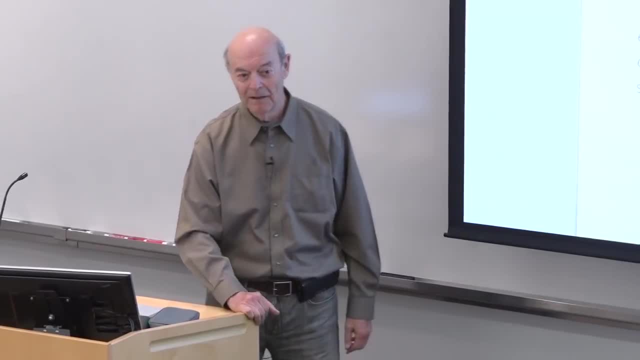 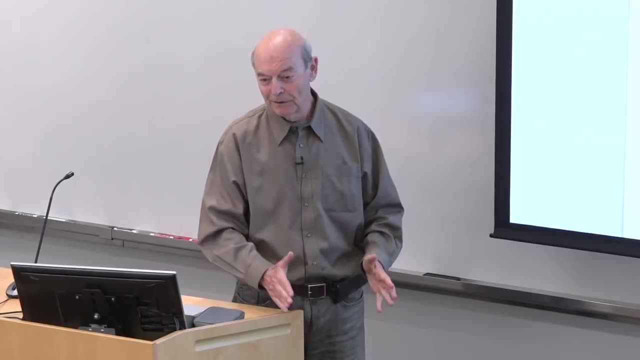 The one they had in mind when they spoke about all this, and that has been proven. Now it's still until now I didn't see any objection. So in the very beginning, when they came with this, I wrote practically to anybody I knew. 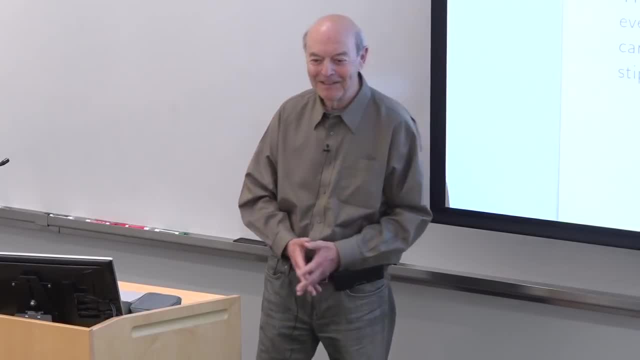 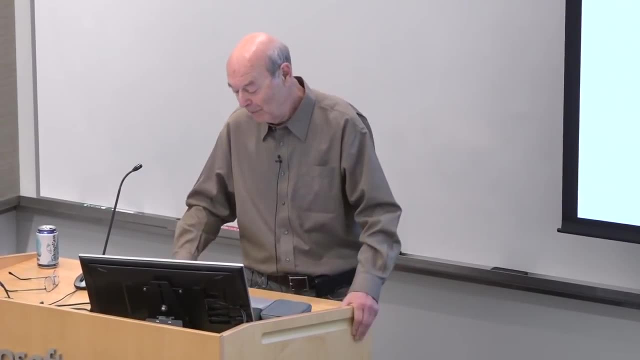 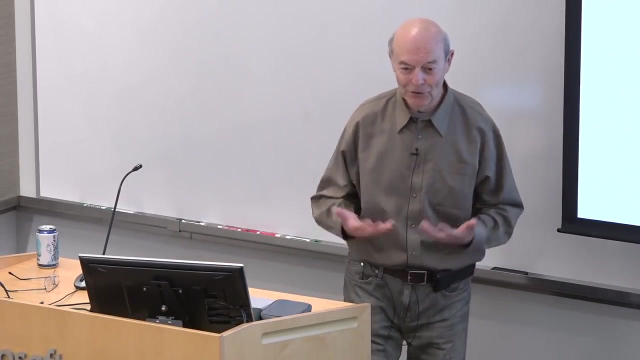 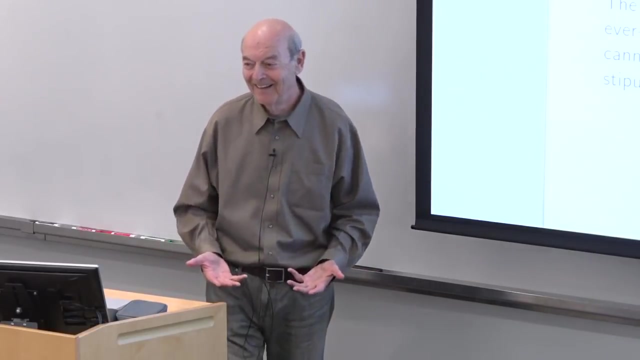 please give me your critique. and people seem to buy Now. sure, still maybe right. But now you take this generalized and generalized, over-generalized version. We still call it Church Turing. They would not recognize it. So you speak about a notion which is evolving. 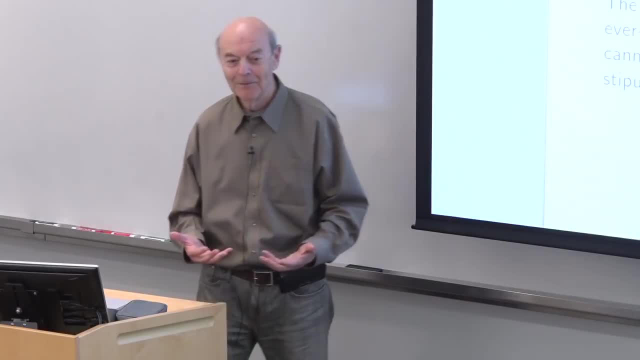 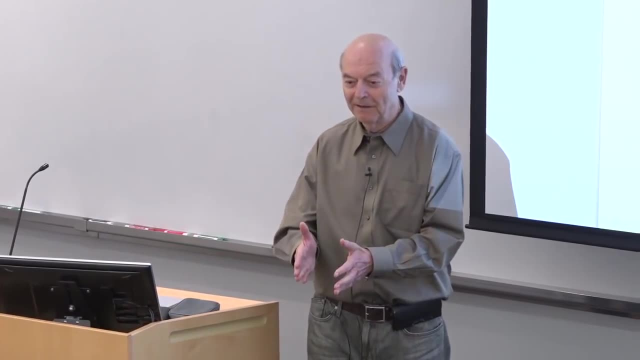 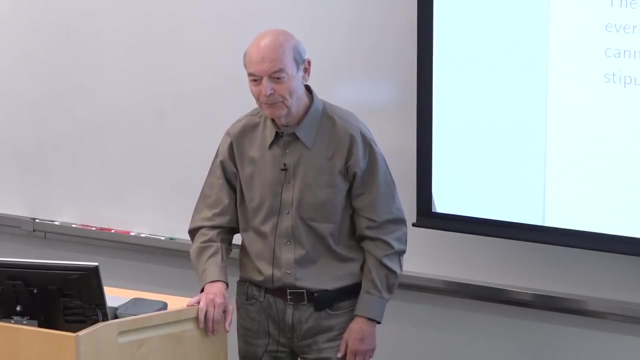 widening ever more liberal notion. You want to claim something about this? Now, of course, we can agree, we can stipulate, We can introduce new species of algorithms, but if they don't compute whenever they compute a function? let me also remark in the beginning: 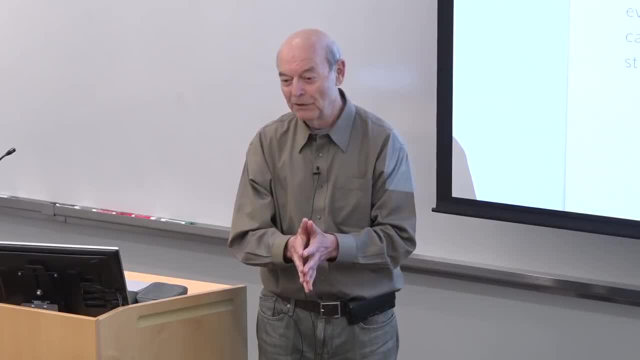 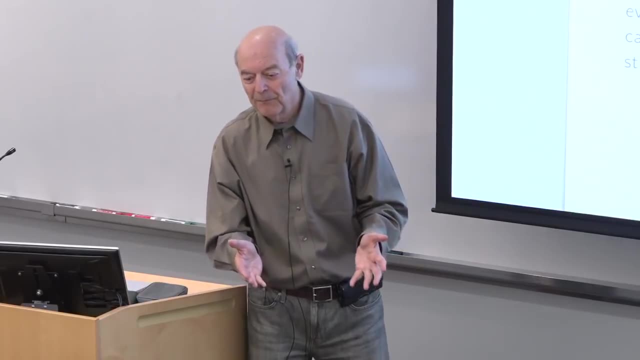 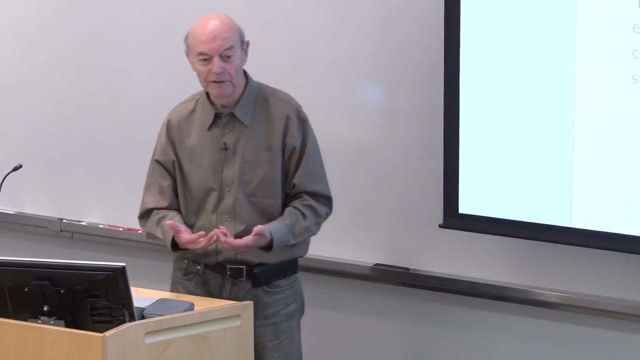 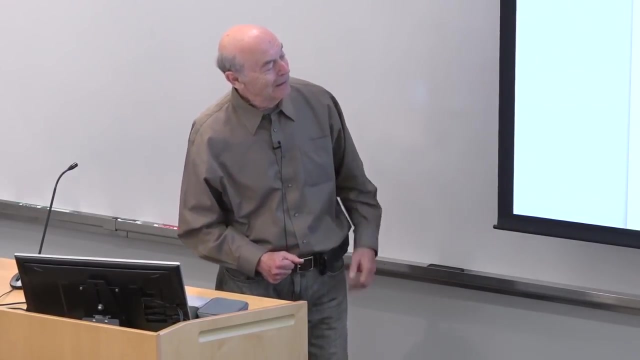 mathematicians who did computations. they spoke about functions. Today, computing functions is tiny, zero. Algorithms don't compute functions. they do tasks, They execute all kinds of things. Very few of them actually compute functions, but nevertheless So, unless we stipulate. 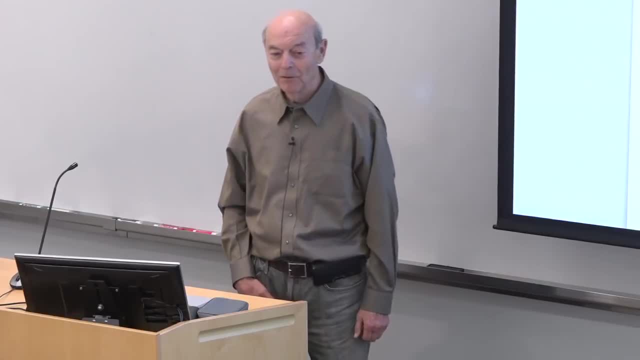 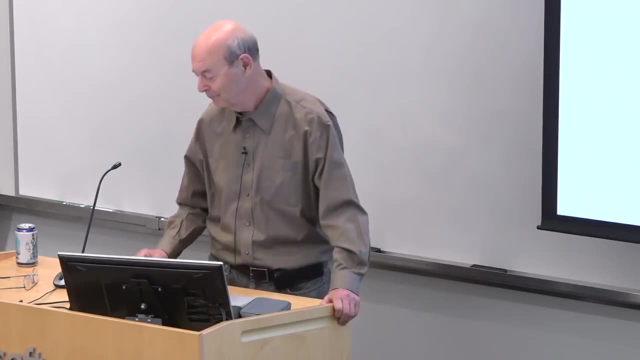 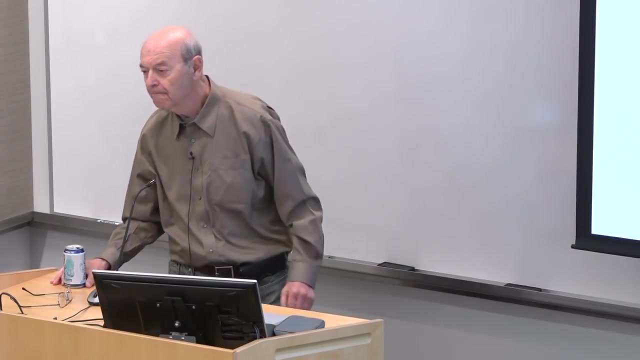 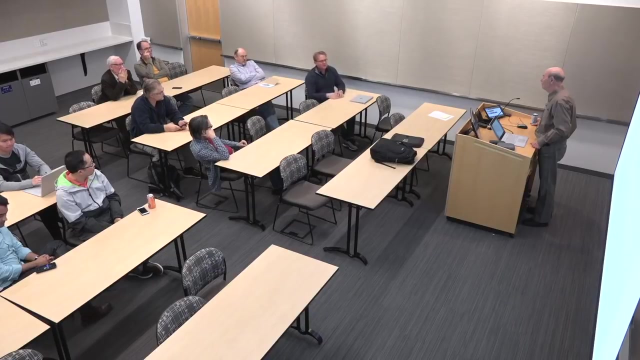 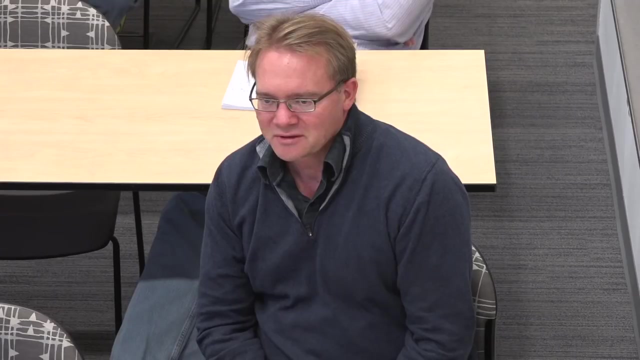 I don't think on any point in history it can be established in any way. That's the end. Thank you, Okay. What are the? so? are there any reasonable restrictions? And what the environment may do in the interactive algorithms? So? 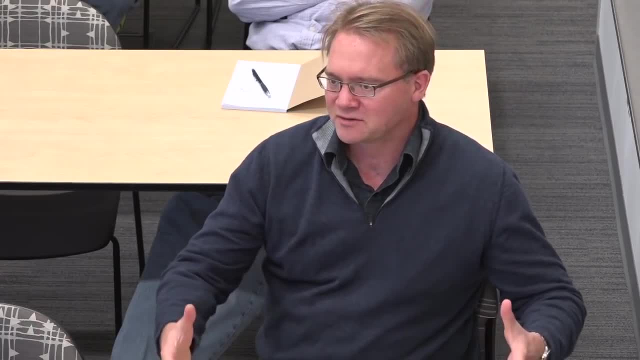 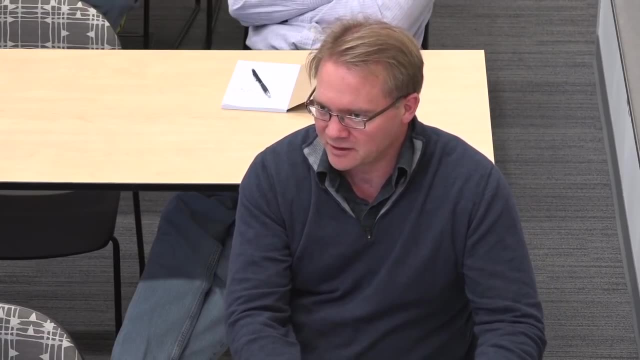 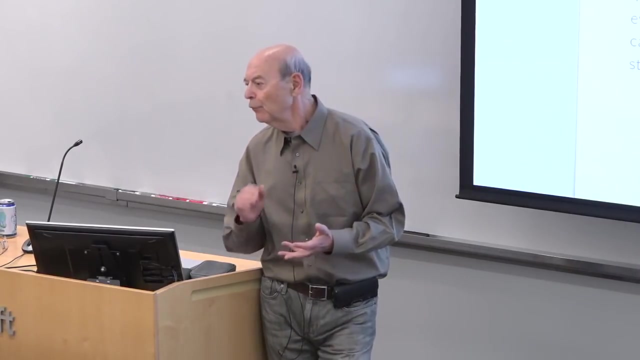 You have restrictions on what the algorithm can do in terms of finite bounded work and bounded finite work, but are there-? So let me say two things. So, in full generality, no, But I tell you what. So Andreas Blas and I will formalize. 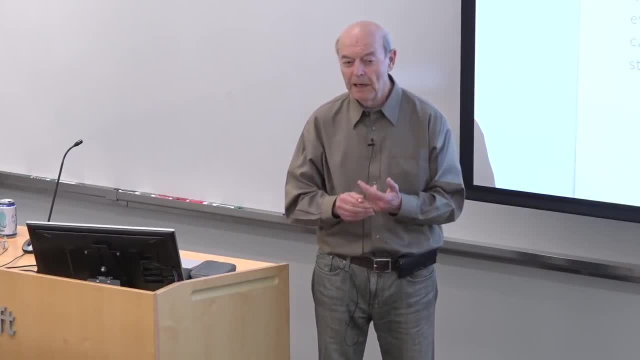 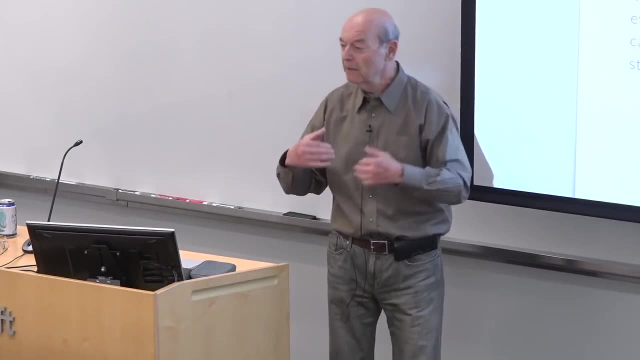 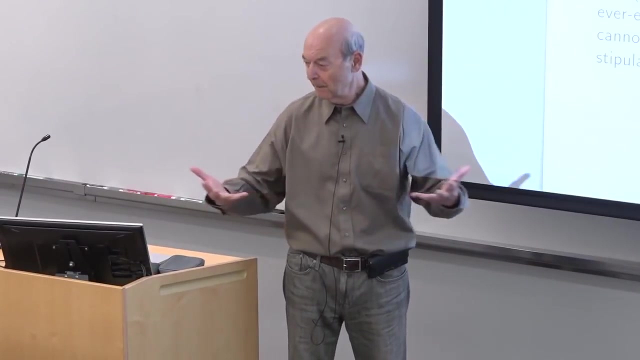 so-called interactive algorithms, And our restriction was that agents may be spread around the world. but when you sent me a message, it makes sense to me, So in my, since my world is mathematical structure, what you sent is an element of this world. 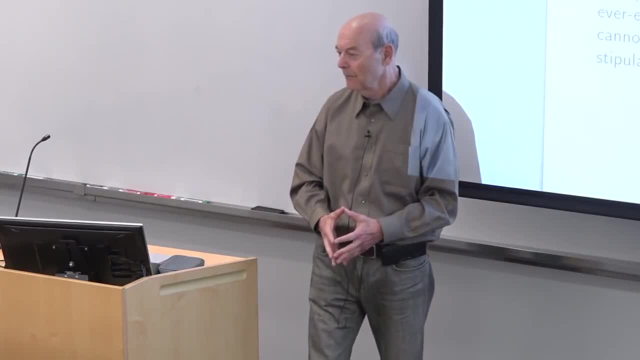 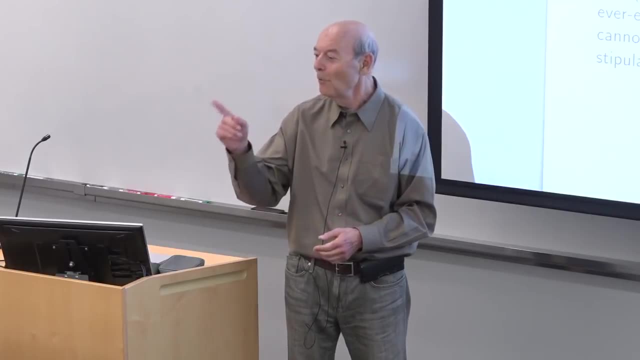 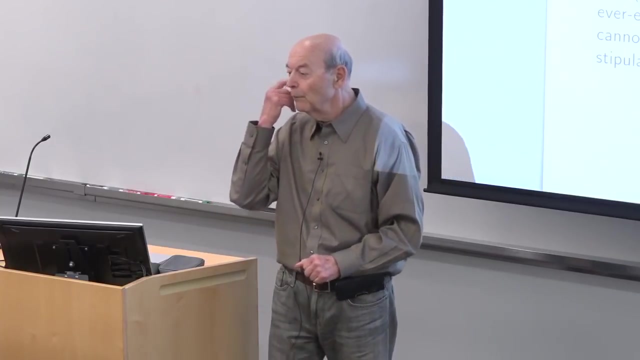 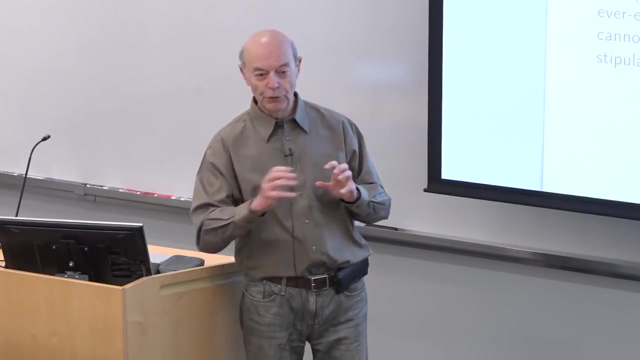 or maybe few elements, Finite observability- Not about observability, but meaningful. In a moment I'll say what I'm trying to rule out. And for this we proved Yes. What exactly did we prove That? if you look at one agent who interacts with many agents? 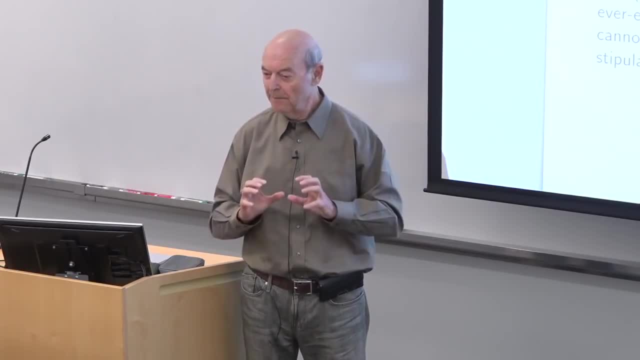 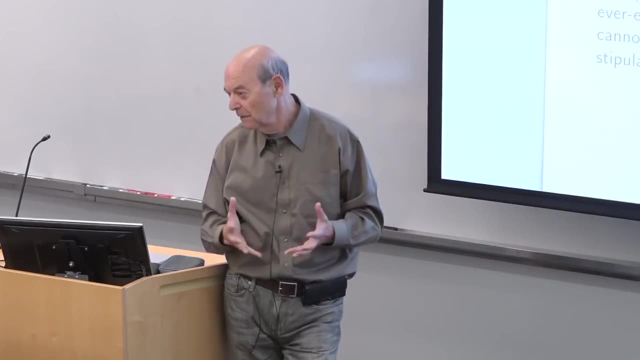 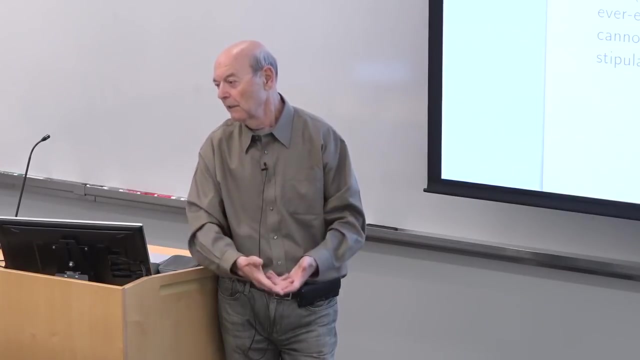 but whenever he has a message, this message makes sense. not to him. you know, he may be an algorithm, he's an algorithm, but it makes sense in this world. It is an element of his structure. What he receives, or representation of an element of his structure. 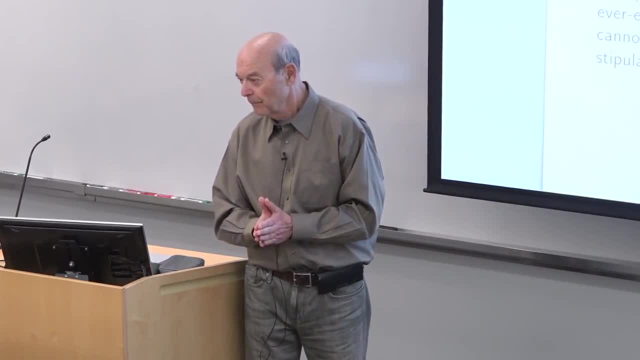 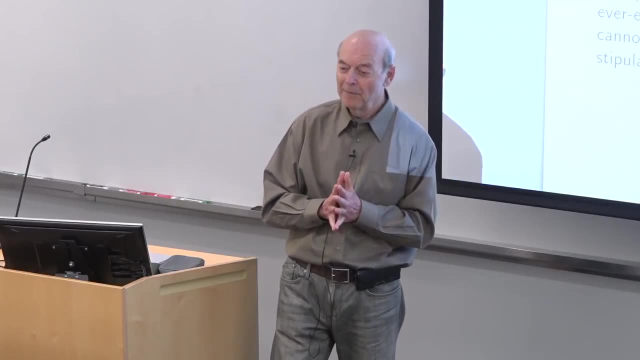 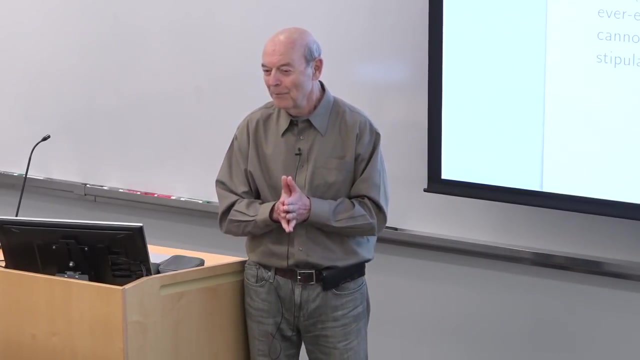 And this we axiomatized. There is another thing: I defined distributed algorithms And at the time I thought in full generality and it was used very successfully. So, for example, there was ITU, International Telecommunication Union. 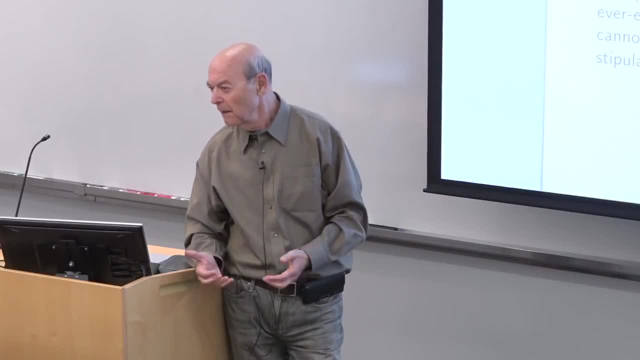 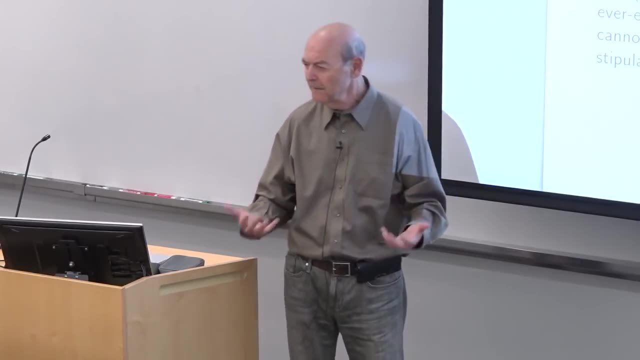 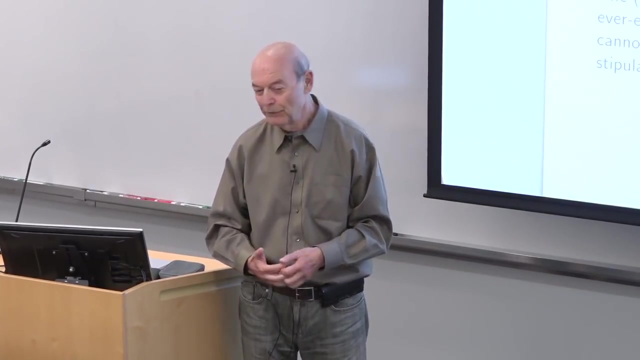 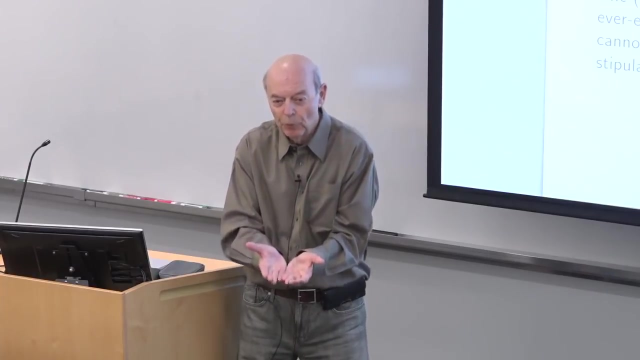 They had some algorithm which they programmed themselves. then they revised it and at certain point the whole thing, their system, became so complicated. they needed help. So they wanted to take their system, to specify it precisely which will allow them to move forward. 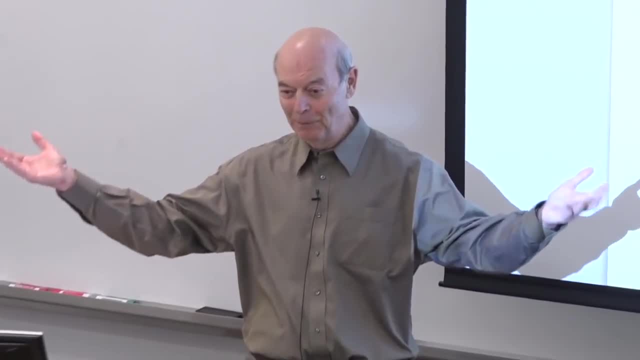 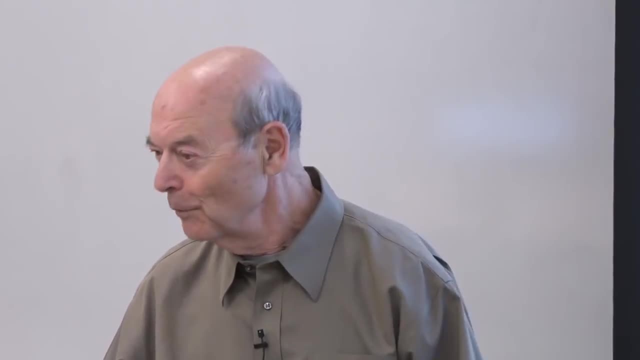 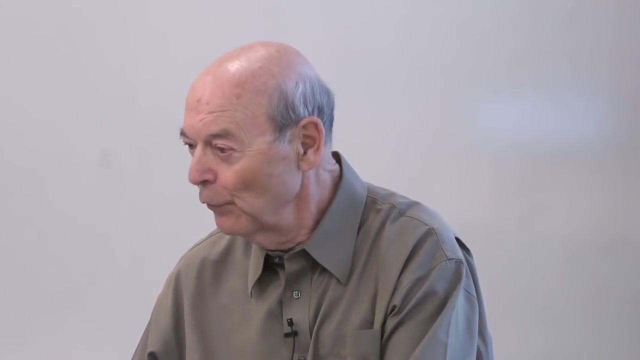 And so they allowed to. all theorists in the world, please do Okay. And not only the same group, which consisted of German professors. not only they won competition, but at certain point they were the only ones, quite early, who were willing to participate. 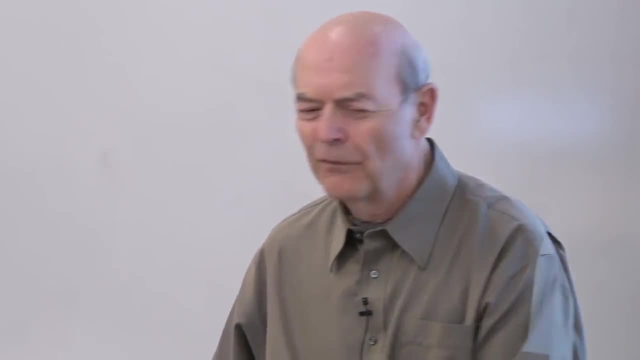 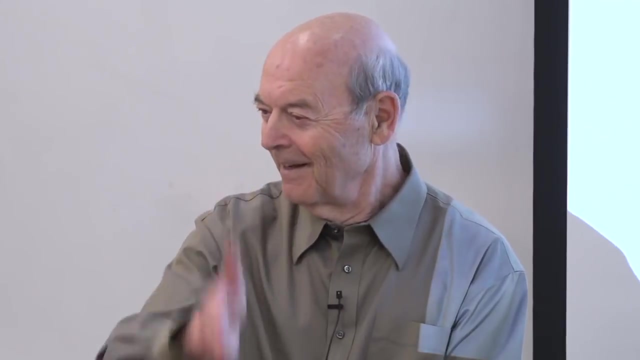 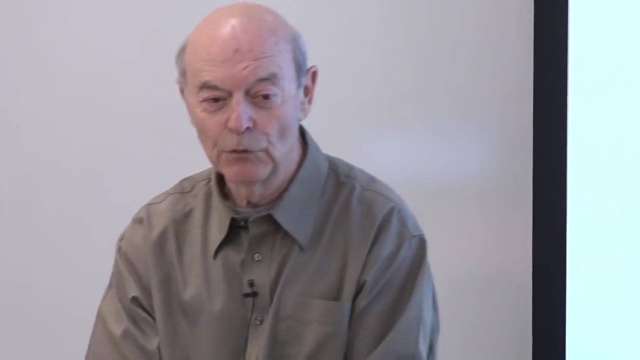 Because this thing was, for example, you can do a lot of things in zero time, Because it was a physical time, but a counter, as they realized, It's never written. Just in zero time you can do all kinds of things. 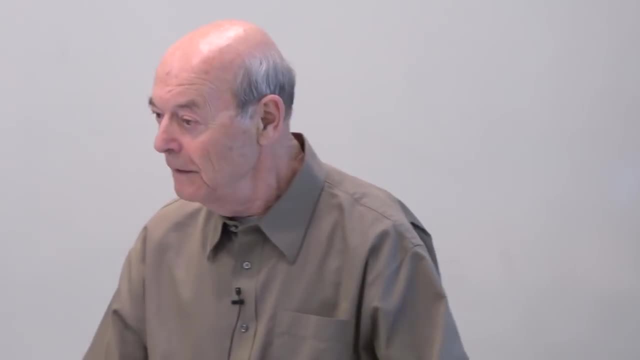 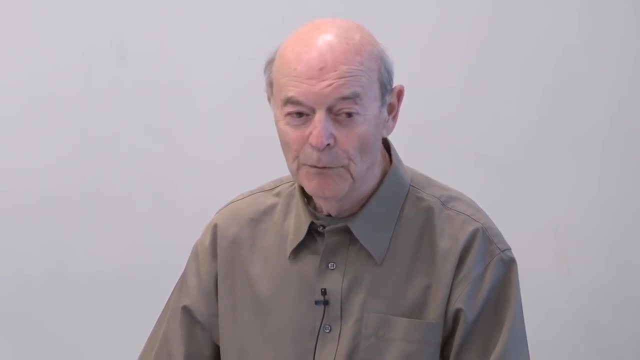 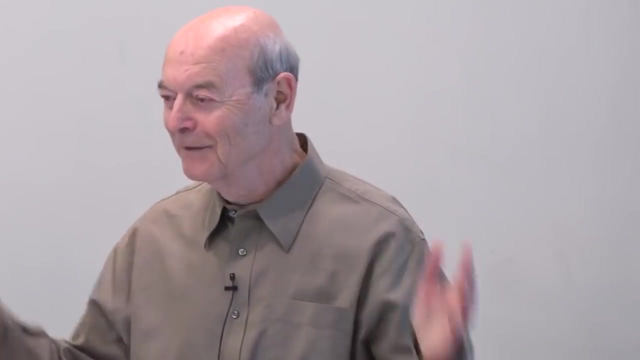 So what kind of zero time it is. So they did it And so I went to Stockholm, gave a talk on, took to community of people whom I never knew on something. I had no idea what it was, Just spoke about abstract state machines. 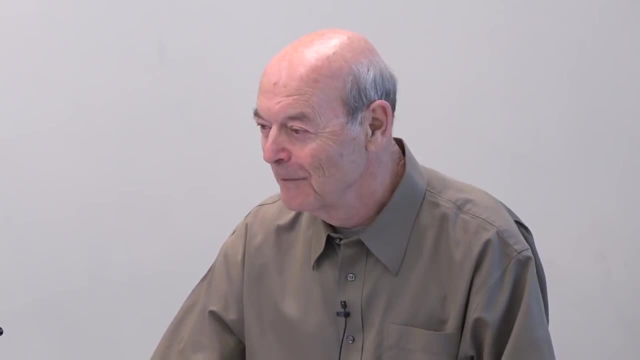 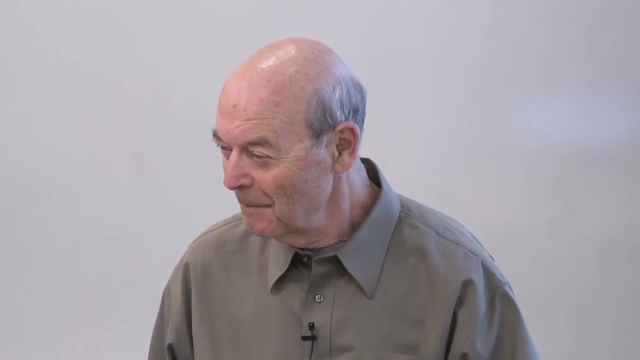 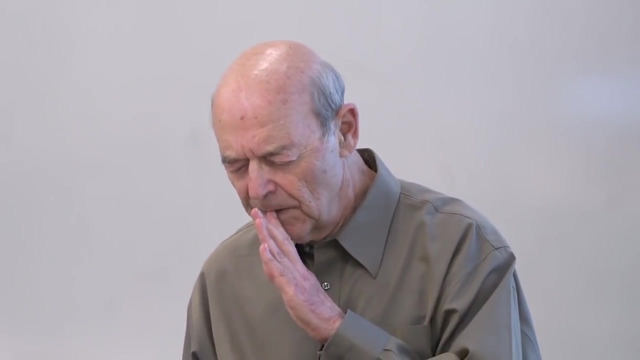 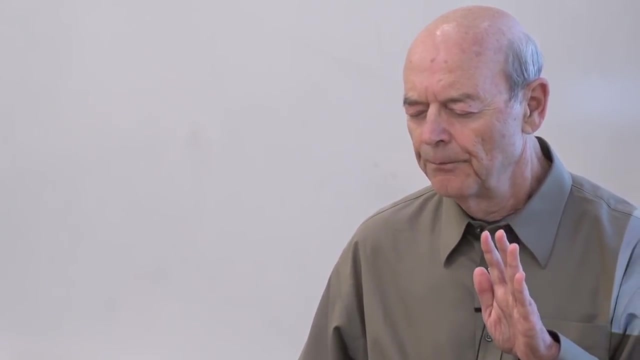 kind of foundation for what these German professors did. Then there was not a single example in the world where it didn't work, But in principle it couldn't work. So it's pretty clear that there is no general, there is no axiomatics for general distributed systems. 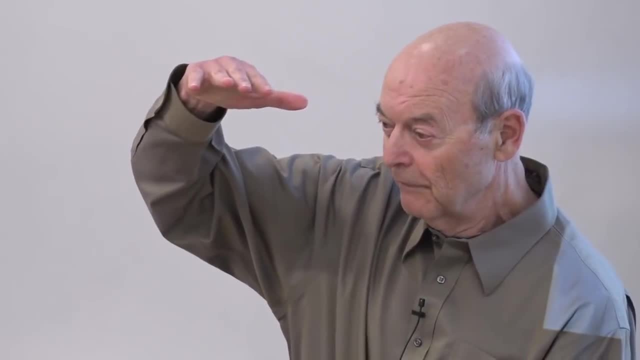 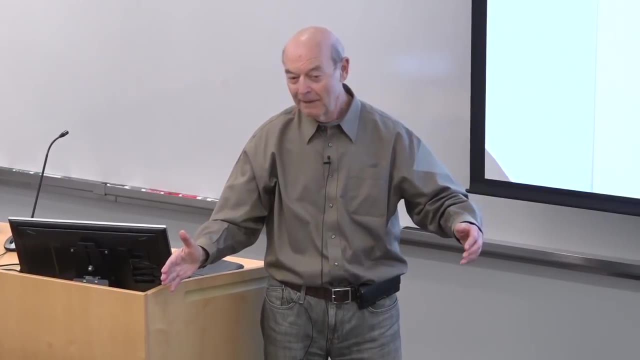 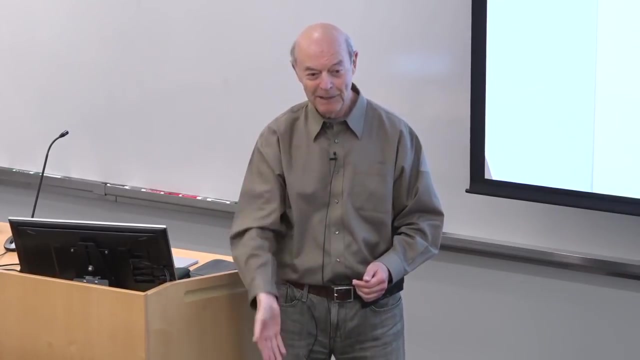 And the reason is this: you can work on completely different levels. That's what's on the real world. So you have very clever algorithm. you proved, you verified it. Somebody comes from outside. Russian hacker changes bits On level of the algorithm. nothing happens. 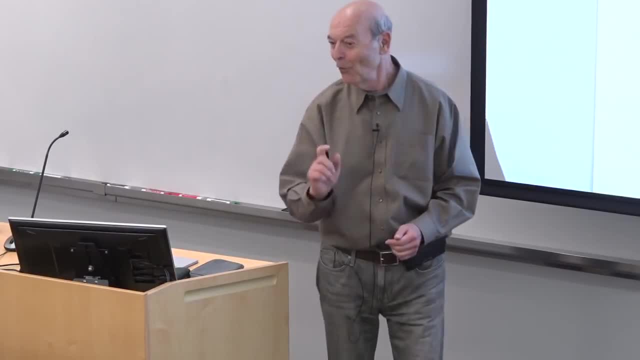 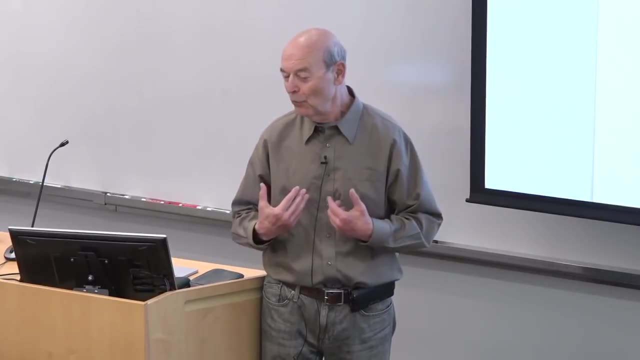 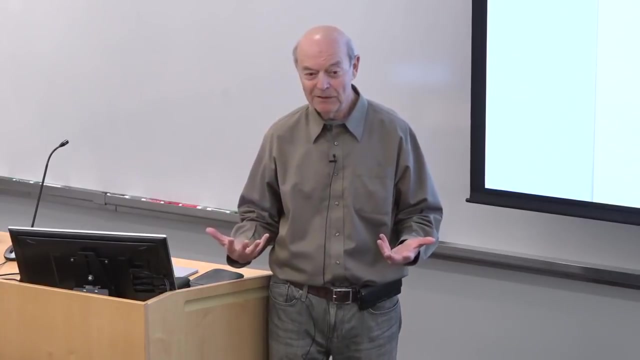 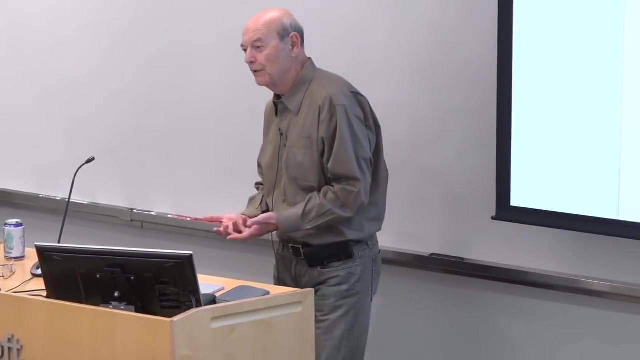 But on the level of single bits he makes a whole and comes in. So from the point of view of mathematical world, of agent one, the incoming messages have no meaning. But that's what in software engineering they call the leakage problem. 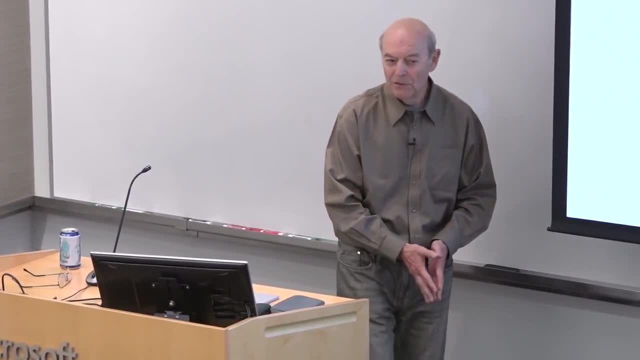 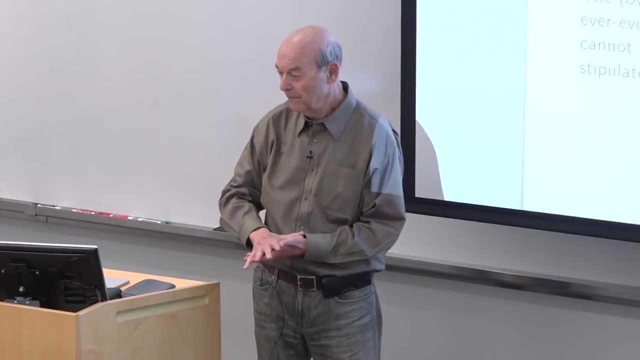 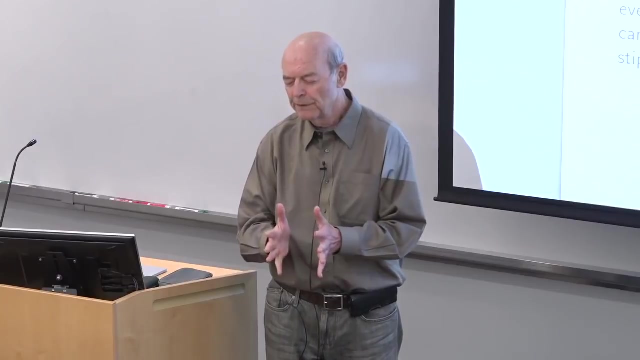 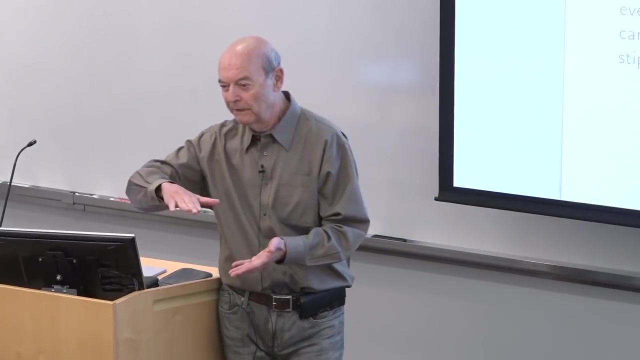 Information leaks down. So if you realize that there is an infinite variety of abstraction levels. So what I didn't prove, but I'm pretty sure the following is true: That if you consider one or maybe finite minimum, but certainly one, 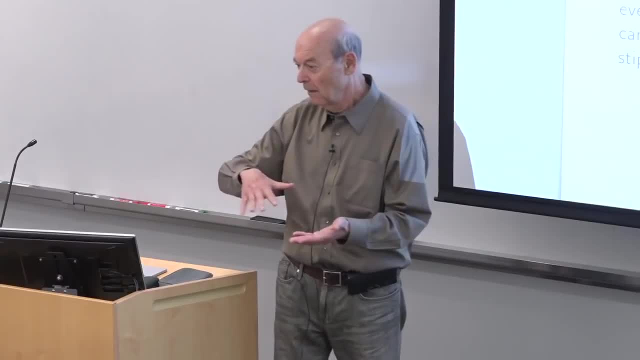 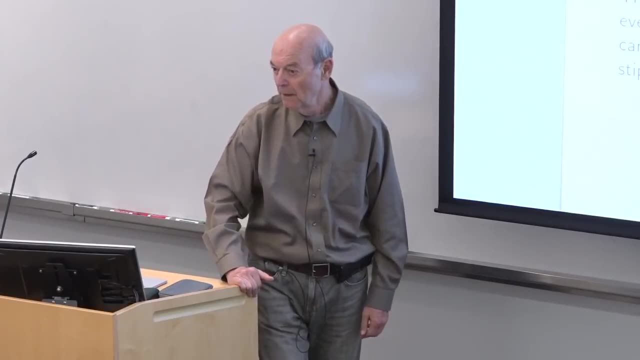 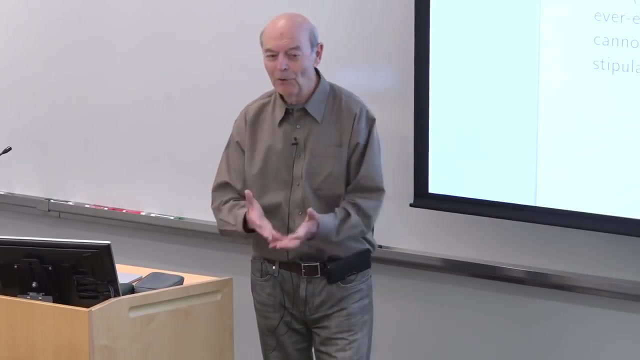 So everybody works on the same abstraction level- distributed. Well, that's how distributed algorithms are written Today, what people call distributed algorithms. That is all reasonably understood, But the implicit assumption is that we all work on the same level. So when send me a message, 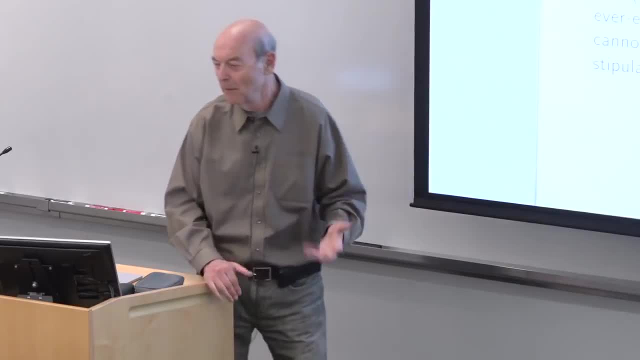 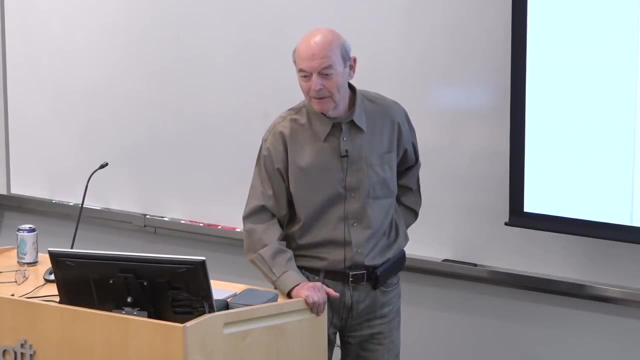 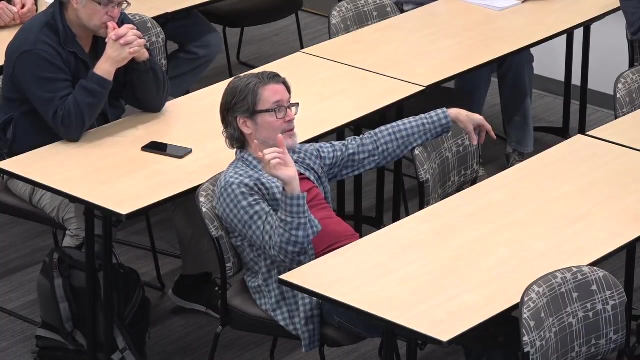 it makes sense to me, or at least it makes sense in my world. Okay, That's the answer. Yeah, I mean so. you talked a lot about abstractions and isolation. To me, those ideas are more important to the idea of computing. 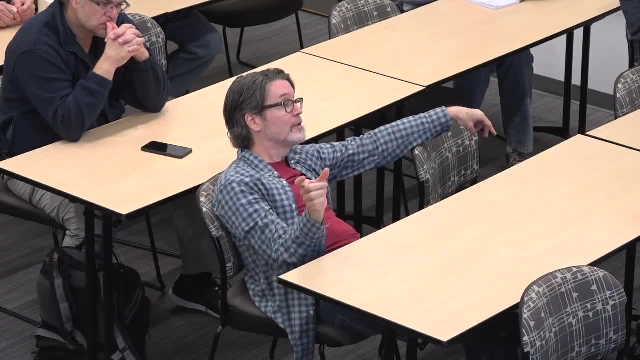 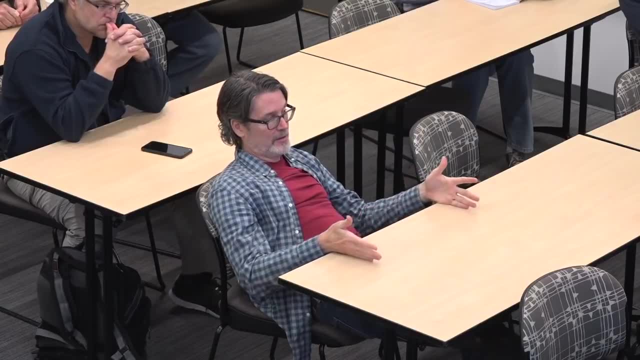 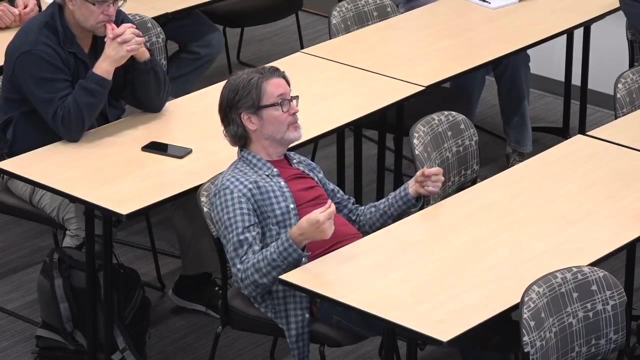 than this church during idea of computing function. So, in other words, to me, computing is taking the physical world, setting up its initial conditions and its boundary conditions such that its behavior simulates an abstract system. In order to simulate, you have to have isolation. 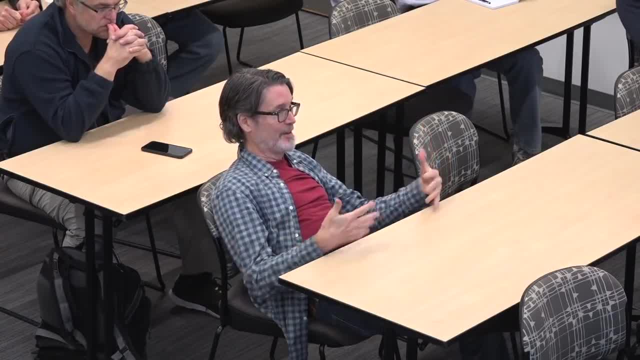 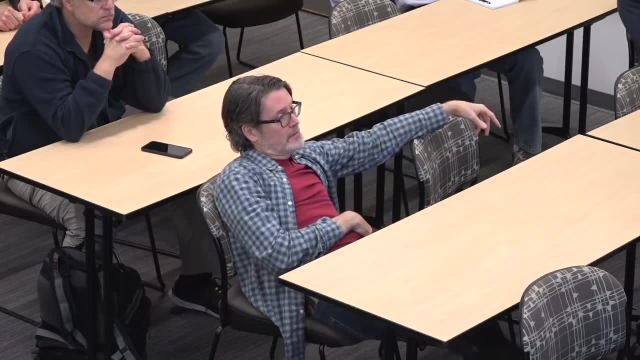 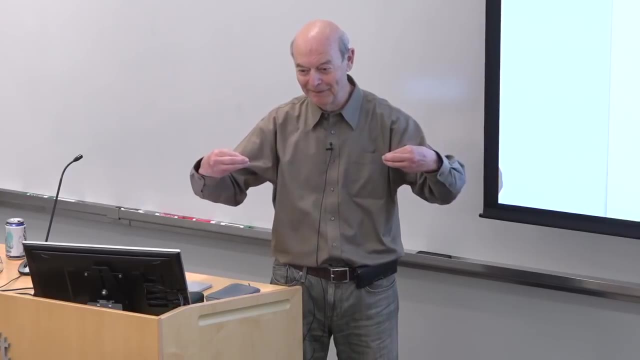 In other words, you can't have information leakage from the outside world, so to speak, into your system. It has to be its own closed universe, Right? Or a little more general: in distributed case you may have exchange, but exchange should be highly disciplined.